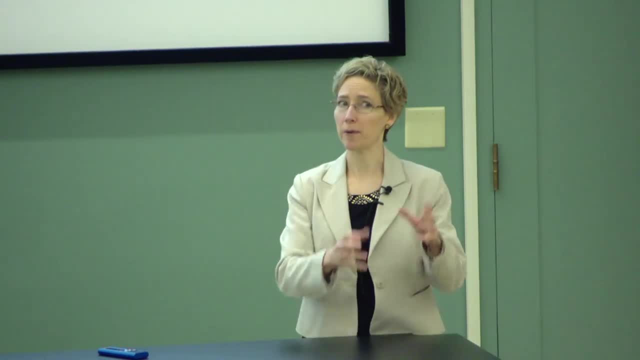 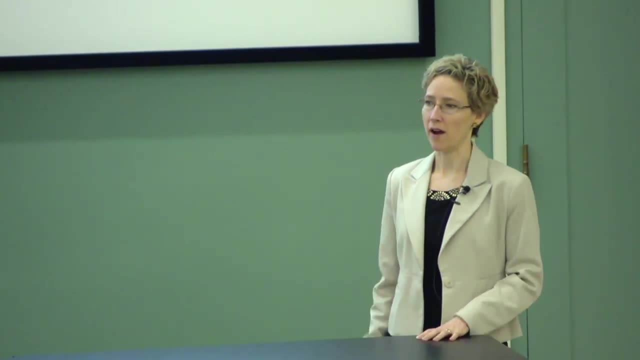 Not that you shouldn't also study those alright, But it gives you an opportunity to know which pieces you really need to focus on. And then you can go into WebAssign and find those practice problems alright And practice the ones that you need extra help with. You may even spot a pattern. 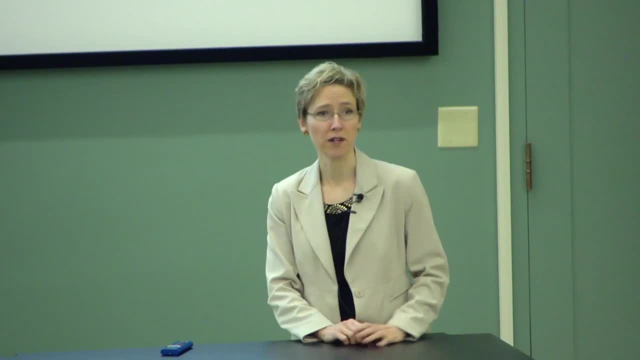 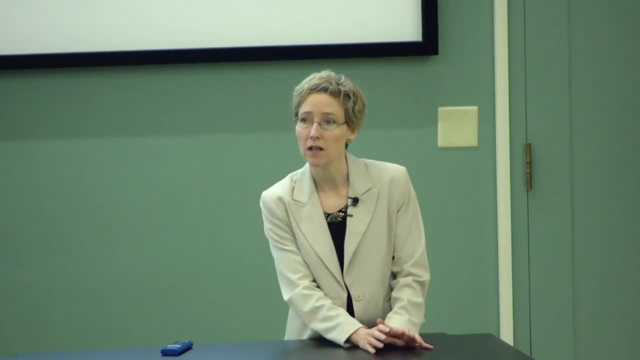 Right. Oftentimes what we find if a student misses, say, five questions on the exam, oftentimes what we find is that they're all kind of in the same category. Sometimes they're all about the same set of material. 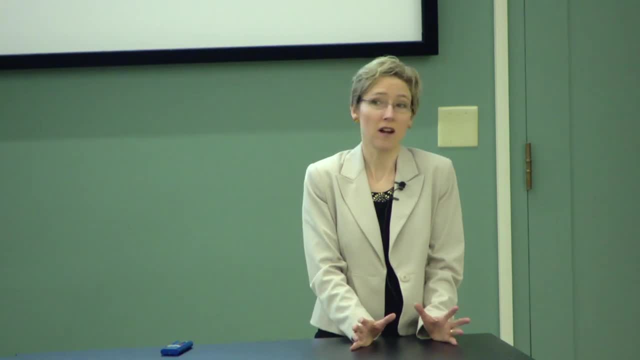 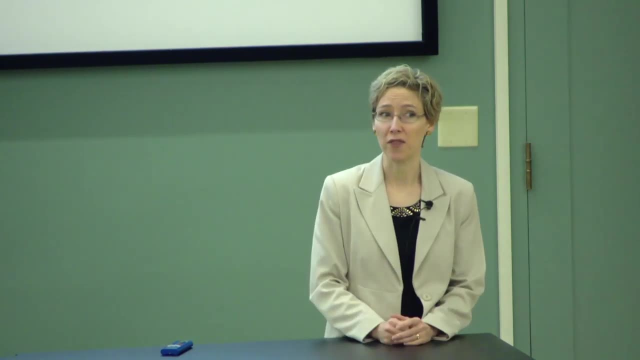 Sometimes there's something else that's biting you, Like: maybe you're not drawing diagrams carefully, So maybe sometimes you might figure out that, Oh, if I had just drawn my diagrams carefully, I would have gotten those five questions correct. 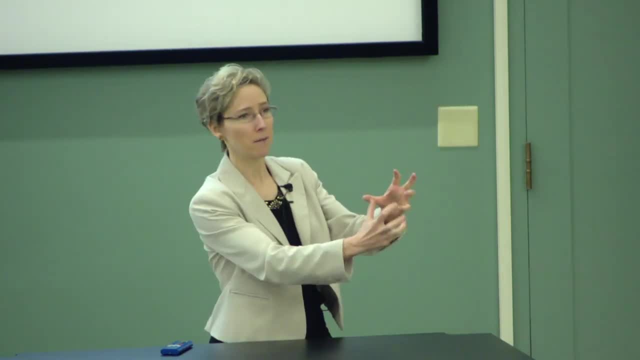 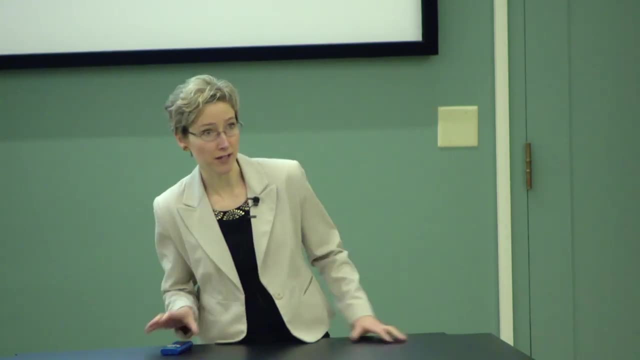 Or maybe you'll find out that, Oh, what got me on those five problems is that I wasn't thinking very carefully. is that I wasn't thinking very carefully? is that I wasn't thinking very carefully about the vectors, which again usually goes back to drawing your diagrams? 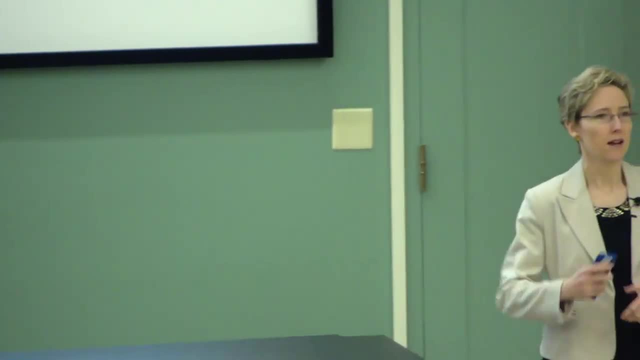 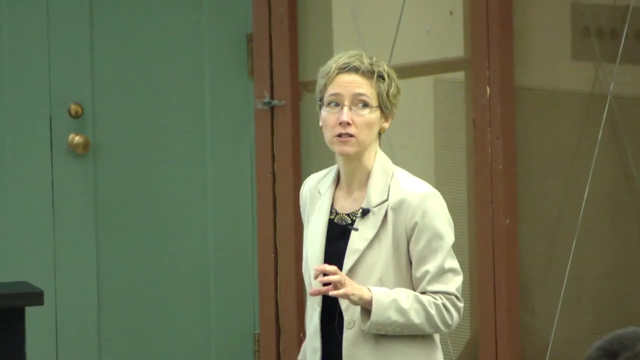 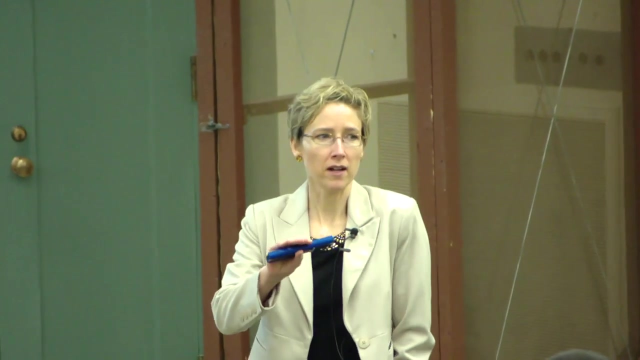 really carefully. so take that practice exam, okay. give yourself a full two hours. take it, see how you personally do and then use it as a diagnostic to help you know how to spend your study time. then you'll make the best use of your study time. the right way to study at this point okay is- is the book, I'm assuming. 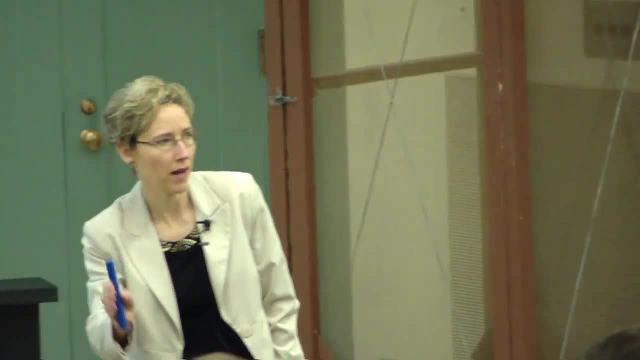 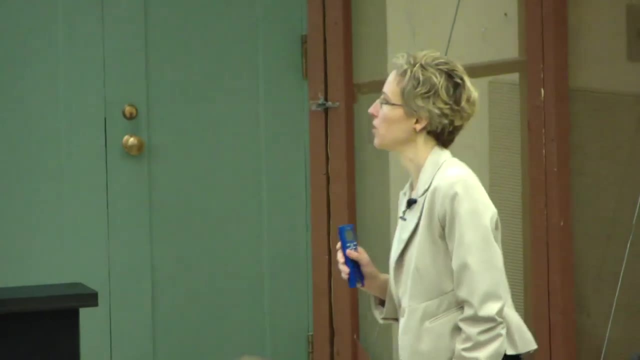 you already read and if, at this point in the in the class, you haven't read those chapters yet, the right way to recover from that is to just dive in and do problems. okay, solving the problems, that's what's going to help you solve problems on the final exam, all right. so study hard and good luck. remember the: 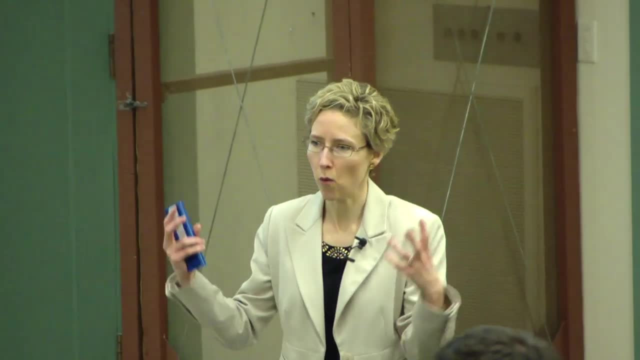 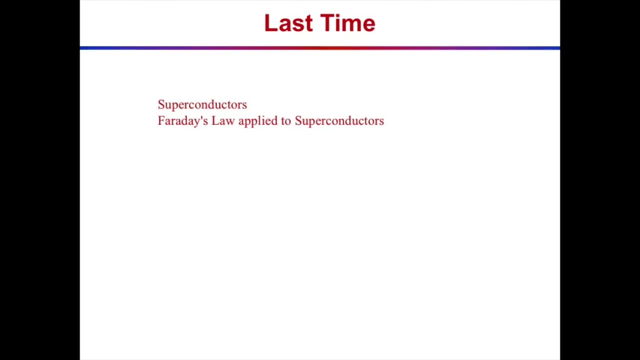 better you do, the better we feel about ourselves as teachers. so we want you to do well, because we want to have taught you well, and so so do well, okay, study hard, good luck, okay. so last time in class we discussed Faraday's law. we learned all about Faraday's law. this time we're going to get to. 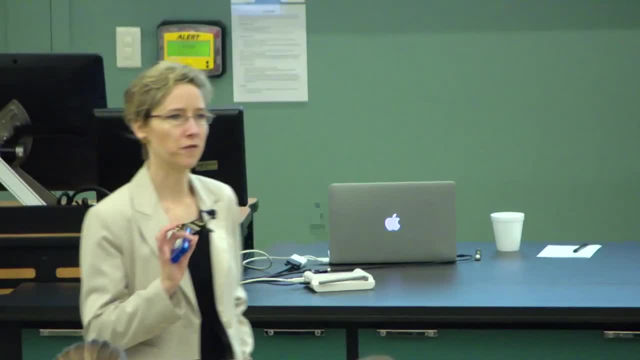 the next chapter and we're going to get to the next chapter, and we're going to the next chapter and we're going to get to the next chapter and we're going to entire complete set of Maxwell's equations. so we will finish out. everything that's known about electricity and magnetism well, not. 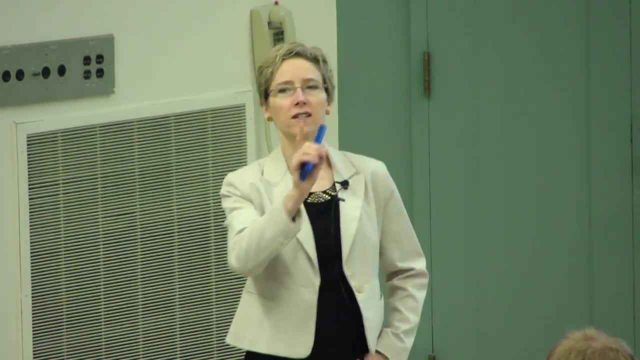 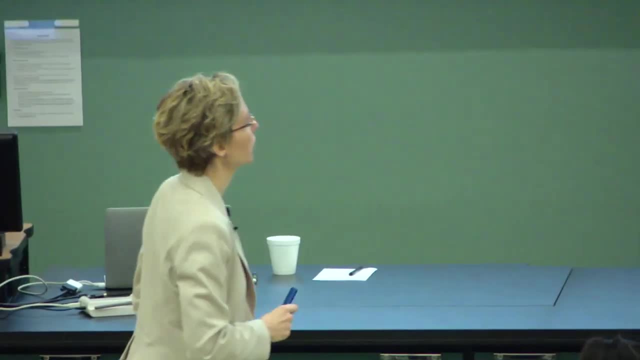 everything that's known, but we'll- we will finish out the equations that govern it. okay, working out the consequences is actually very hard, but we'll finish out the equations that govern it and we'll have the complete set of equations that govern everything having to do with electricity and 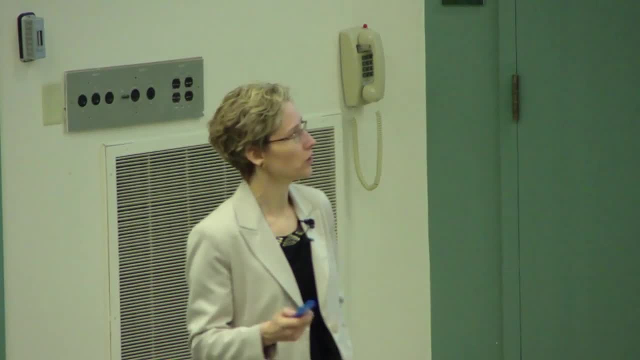 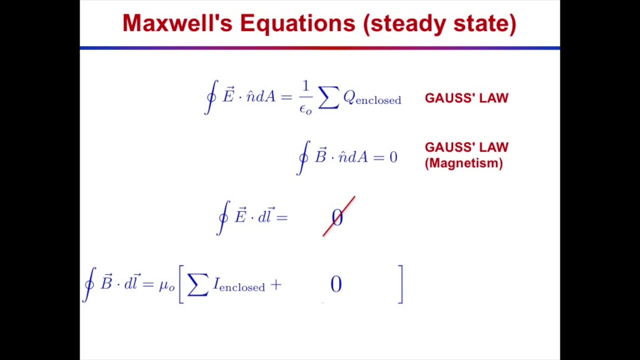 magnetism, and if we have time for it, I'll show you the wave solution of those guys. so here's what we've had when we were talking about the time-independent pieces of Maxwell's equations. So what I mean by time-independent is the steady-state case. okay, 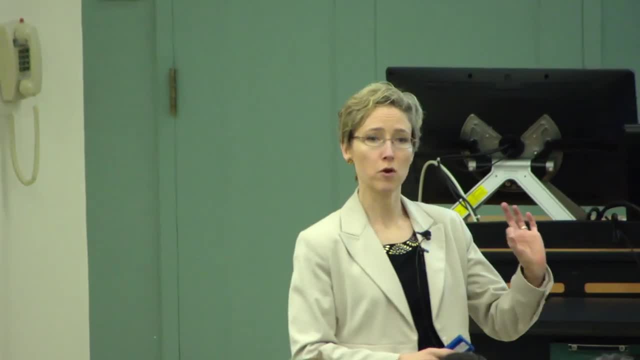 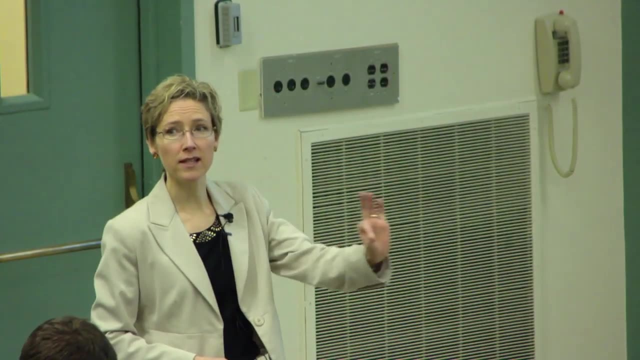 So this was a case where we had charges and we could have charges moving as long as they were moving at constant velocity, which we report in Maxwell's equations as a constant current. So in the steady-state case, these are Maxwell's equations. 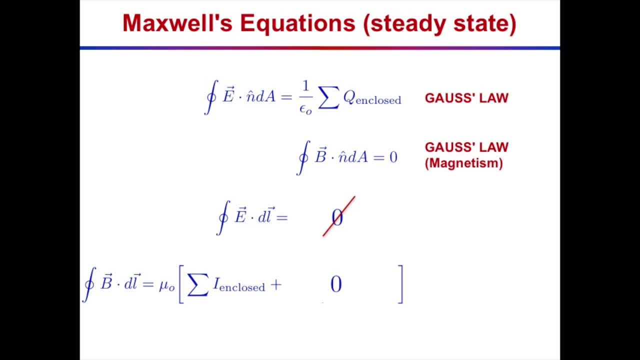 What we did last week, though, was we said: okay, these places where there's a big fat zero we're going to update. okay, Last week, in chapter 23,. we updated this piece and said: well, look, a changing magnetic flux with time. 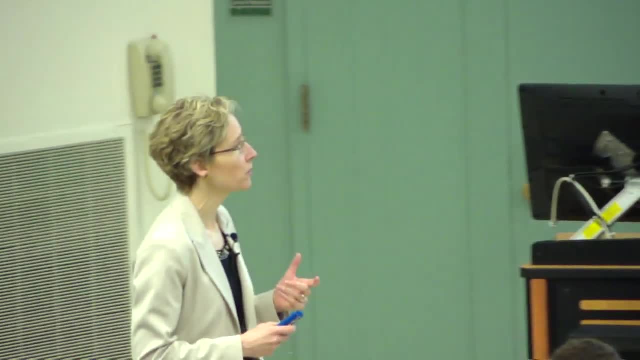 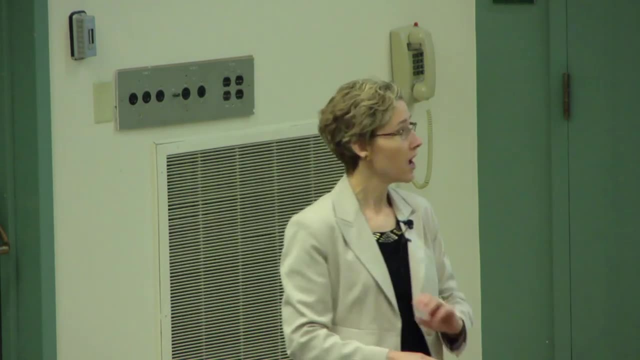 can cause a curling electric field. That was Faraday's law, And so we updated this piece. That's not a steady-state piece, right? That's got a time-dependence to it. So what it told us was that if there's a magnetic flux, 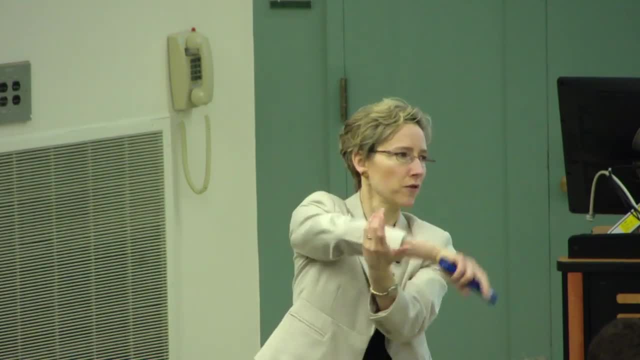 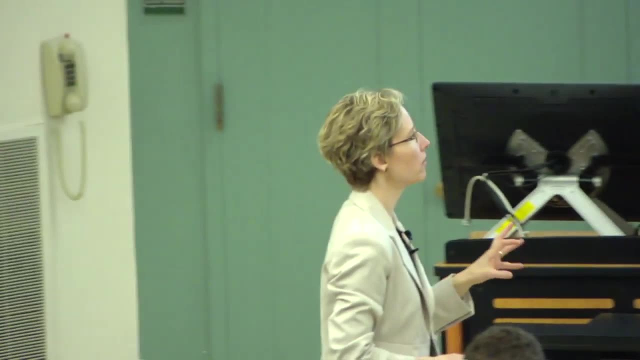 and that magnetic flux changes with time. it causes electric fields to curl around itself. What we're going to see today is that this part here Ampere's law also needs to be updated with a time-dependent piece. So Ampere's law told us that. I can get a curling magnetic field if I have a current. So a current running causes a magnetic field to curl around itself. But by analogy with Faraday's law you might think, well, look, a changing magnetic flux, just a changing magnetic flux. 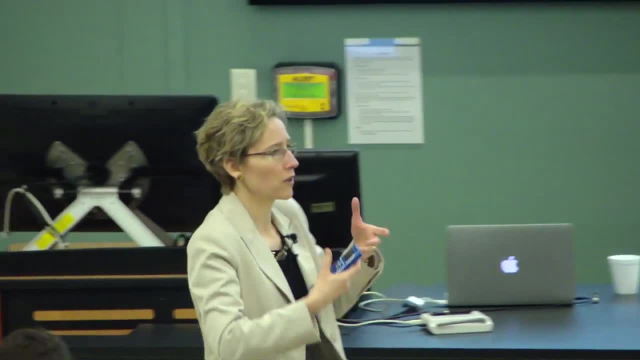 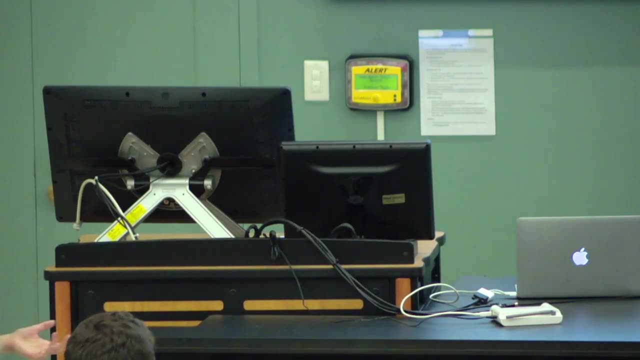 caused a curling electric field. Maybe a changing electric flux causes a curling magnetic field? okay, And this is exactly the insight that James Clerk Maxwell had. So this was called Ampere's law, but if you add in that time-dependent piece, 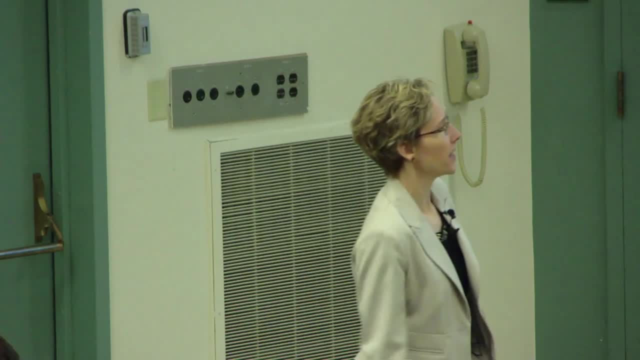 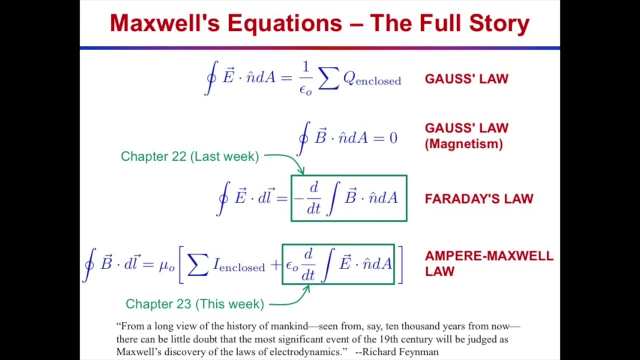 that we'll study today. this was Maxwell's big idea that now that's the complete set of equations for electricity and magnetism. So this piece was added by James Clerk Maxwell, and everyone agrees this was a great leap of genius to do this. 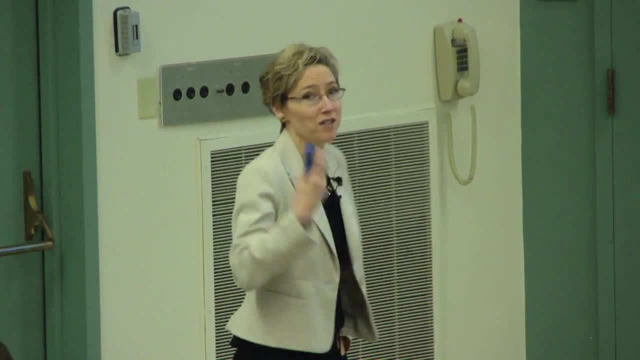 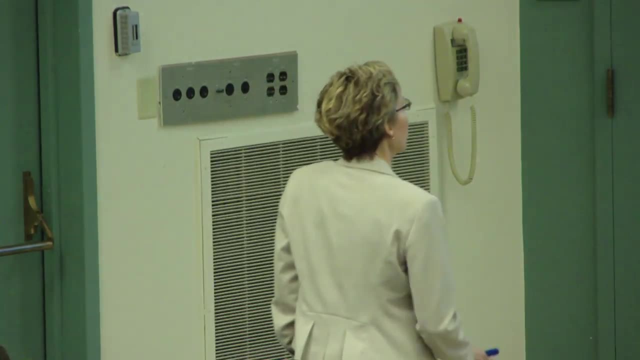 He was thinking about the symmetry of these things. Actually, he also reports that he was thinking very deeply about the concept of trinity. So he was having deeply spiritual thoughts while he was trying to solve these equations. And you can't, it's impossible to overemphasize. 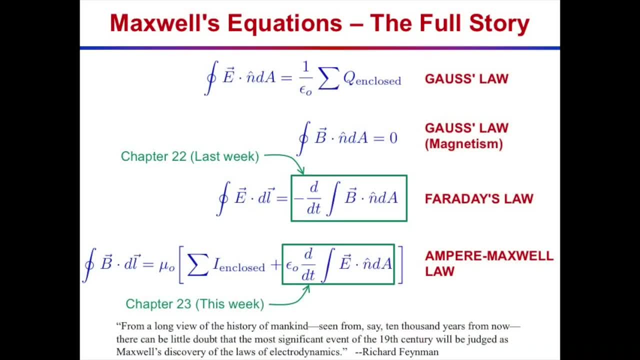 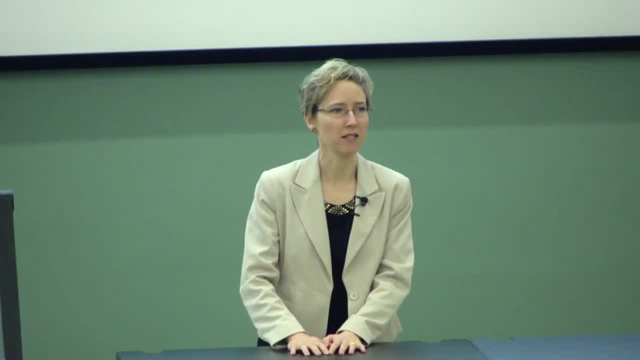 the importance of having put this term in. okay, So once Maxwell did that. that's the complete description of electricity and magnetism. This is: if you have this stuff in place, you can predict all the other things you need to know. 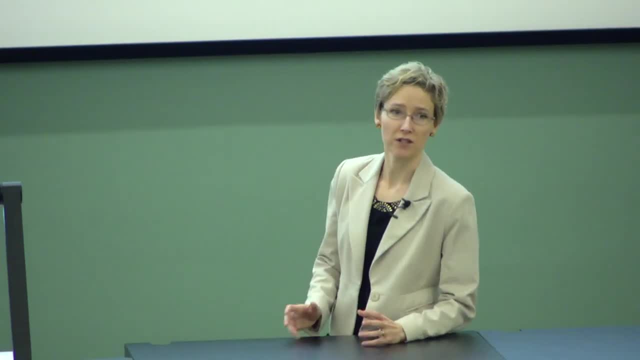 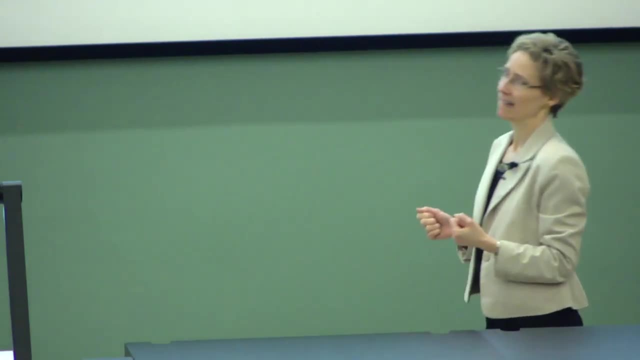 So, for example, if you just took this piece of lecture and you said, okay, I got it, I wrote these equations down and now hop into your time machine, because I know you keep one in your garage, right? So hop into your time machine. 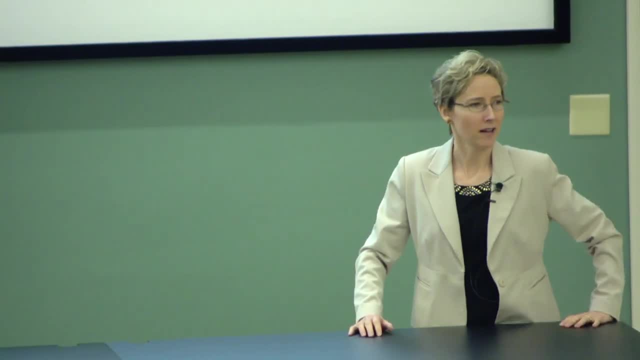 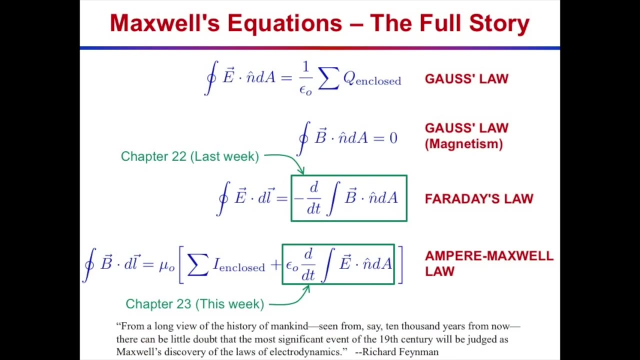 and go back in time 300 years. You would change the world right. You would have in your power to do things like: oh my goodness, based on this, I can create. I can create telegraphs. alright, I can set up a whole telegraph system. 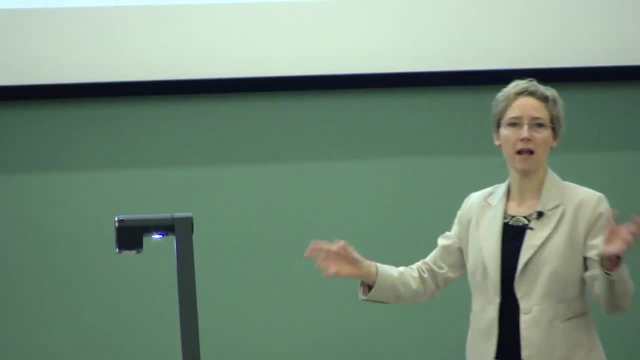 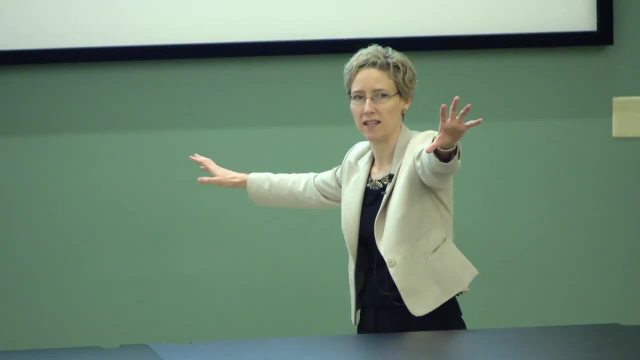 of telegrams. and this is what these equations right here are, what enabled us. this is why we, as a world, laid down that big ol' cable in the Atlantic Ocean connecting two continents and allowing telegraph communications. That was enabled by Maxwell's equations. 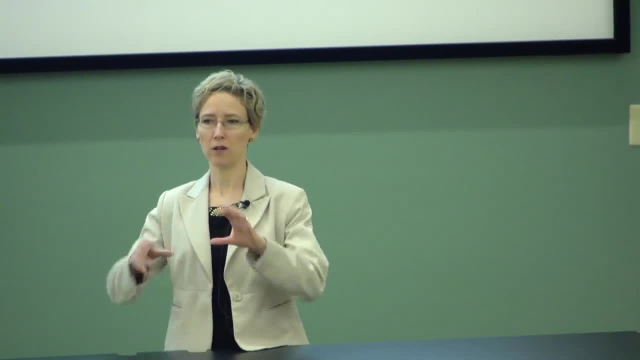 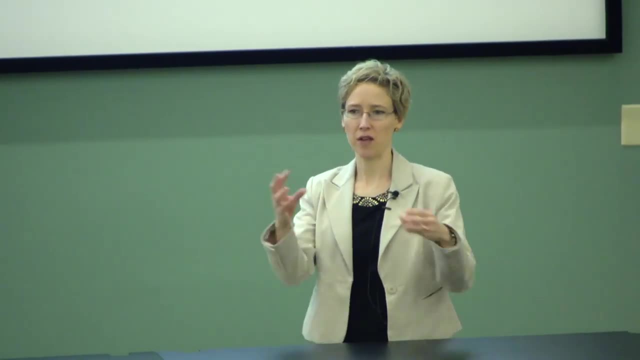 This is what enabled the telephone, okay, So communications over whether they're over wires or without wires. So this enables your cell phone technology. It enables everything from the electronic circuits that are inside the little chips that you can't see. alright, 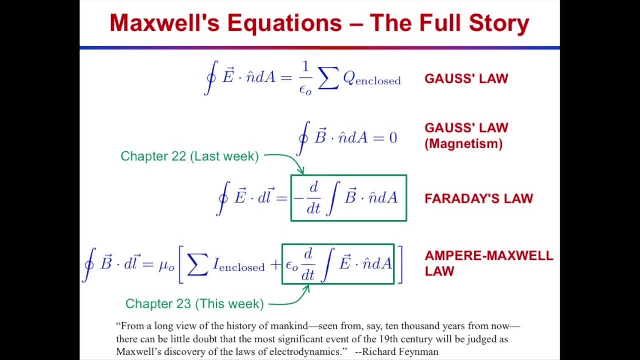 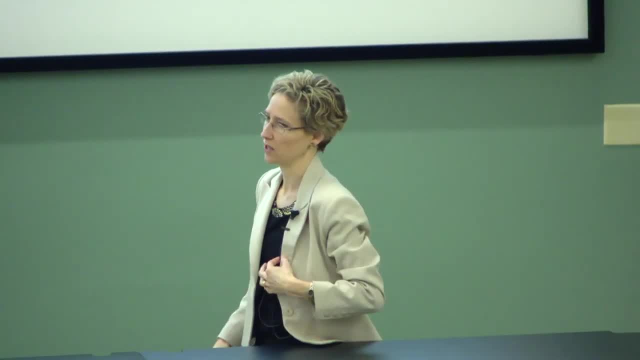 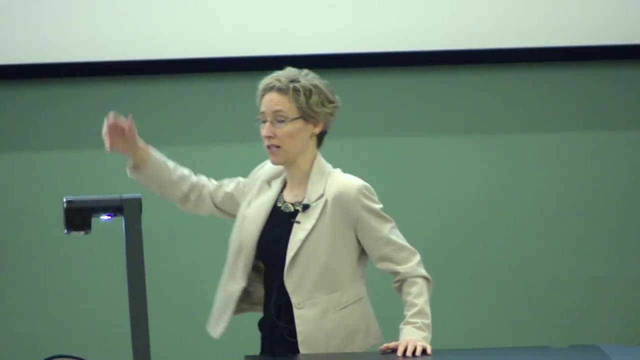 To the wireless communications that let your phone connect with the cell phone towers. It also enables light, so the fact that light is propagating in this room is controlled by these equations: Radio- okay, So radio communications are enabled by having put all these pieces. 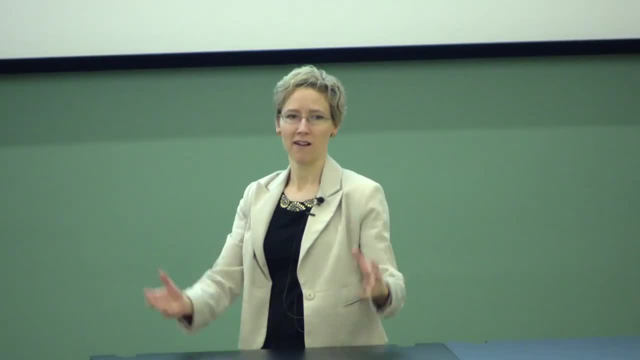 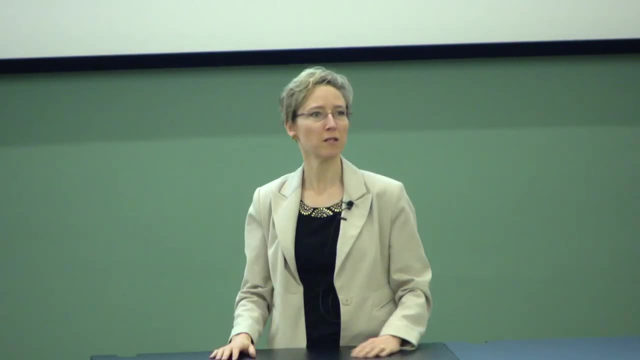 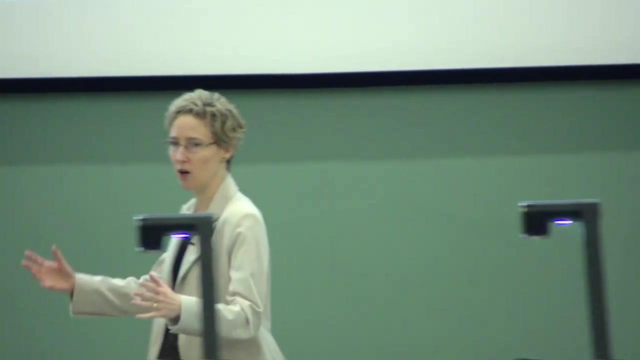 together Satellite communications, I mean our entire, you know, modern society basically, is founded on these equations up here. You can't overemphasize it. Could Maxwell possibly have foreseen all of the societal implications of figuring this out? No way, alright, Did he know he was gonna? 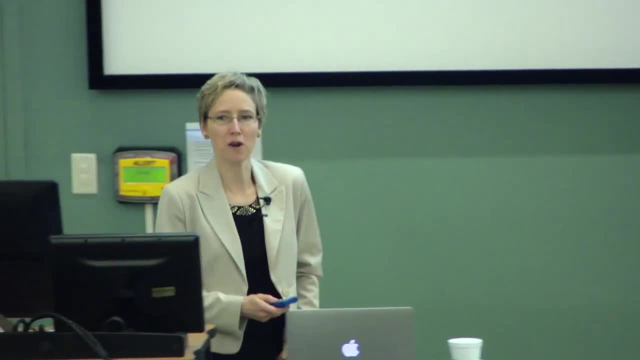 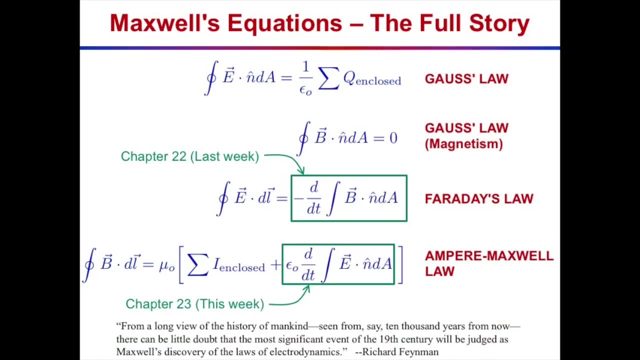 make a global society by having done that? Nope. So who knows? Alright, if you decide to, you know, switch into basic sciences and do something pretty amazing like that, who knows what the implications will be for your work in the future as well? 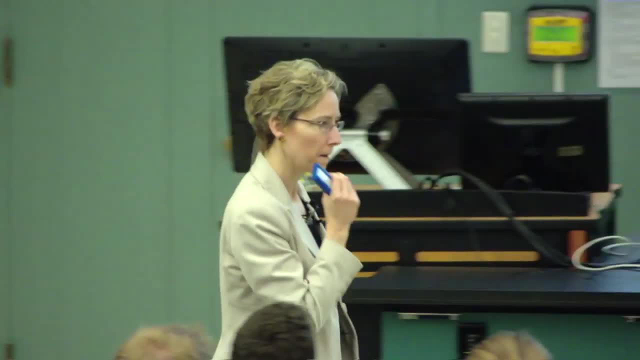 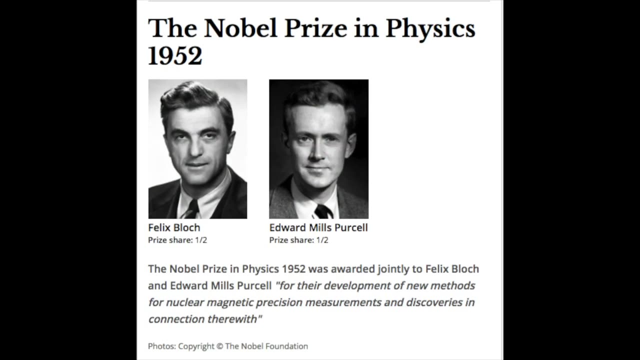 Actually I should also tell you, since you're sitting right here in Purdue. alright, there's um once, a long, long, long time ago, there was a man here named Edward Purcell who got his bachelor of science degree in electrical engineering at Purdue. 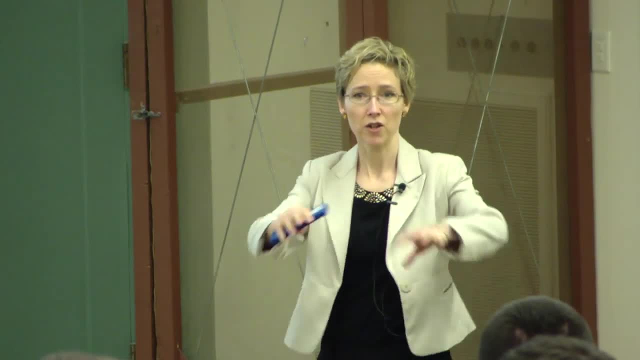 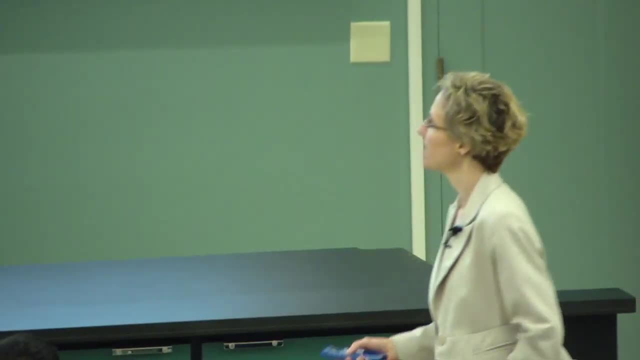 and he went on to get a Nobel Prize- alright, So sitting amongst you right here, maybe there's another Nobel Prize winner right now who's gonna do something else amazing like that. Alright, so adding time to Ampere's Law. what do we need to do? 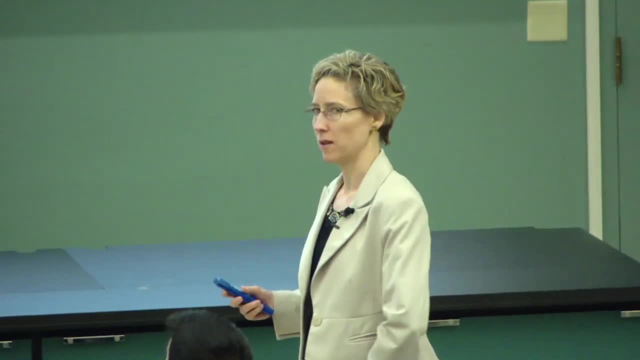 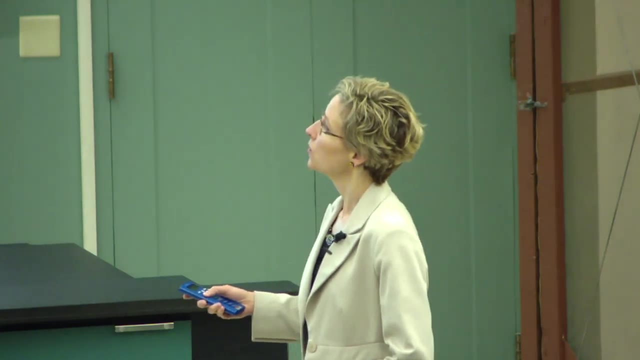 to do that. We had Ampere's Law last week and the previous weeks, but it didn't have explicit time dependence other than the current. The current was assumed to be steady state alright. So now let's think about what happens if we think of 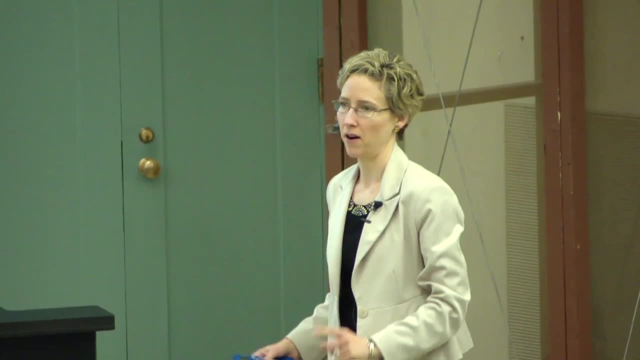 well, let me set up a conundrum first. So first I'll set up a paradox, and then let me show you how Maxwell solved the paradox. So here's Ampere's Law, which, as we know, is incomplete. it doesn't. 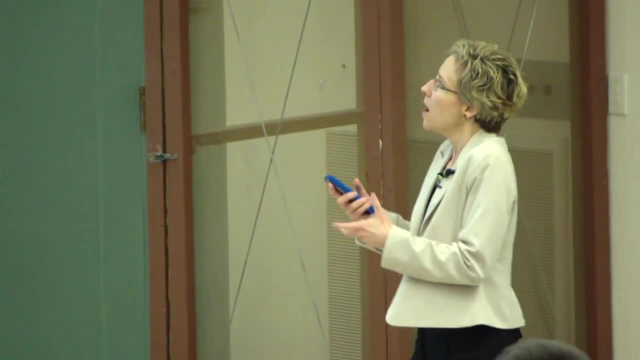 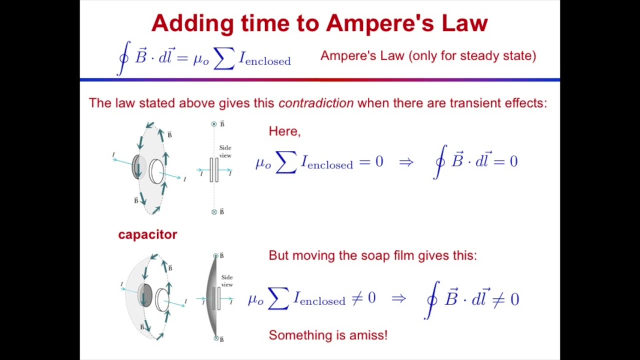 have explicit time dependence other than that steady state current. but if things are changing with time, we're gonna get a contradiction. So the law stated in this way gives a paradox. Let's say that we apply this to a capacitor, alright. 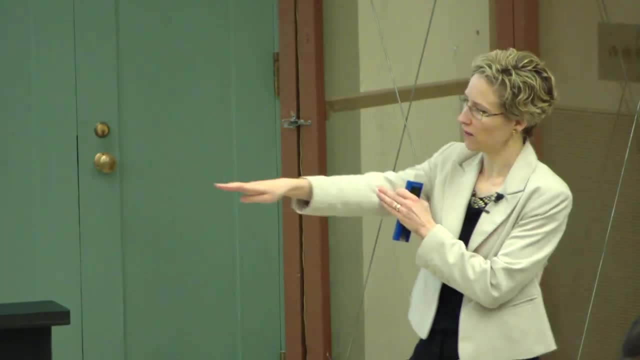 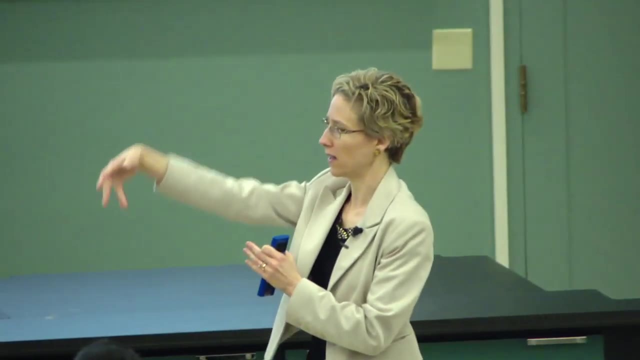 So what this equation means, what Ampere's Law means, is that if there's a current running, there's a magnetic field curling around it. okay, So current running- magnetic field curling around it, current running- magnetic field curls around it. 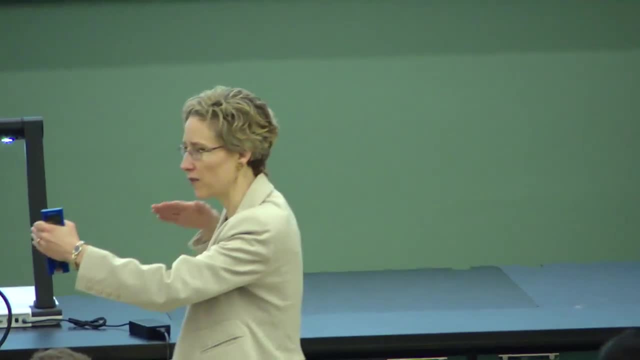 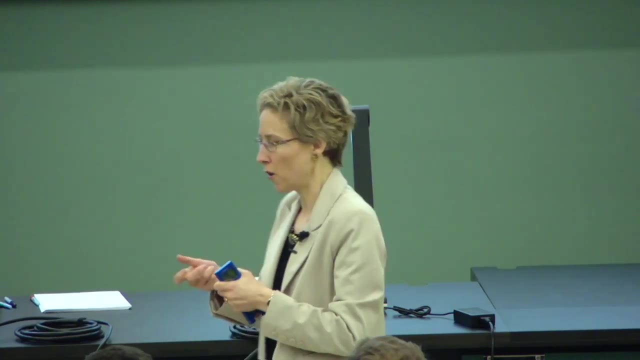 What happens when we get to a capacitor? alright, When we get to a capacitor, if current's running and gets to the capacitor, the current doesn't go through the capacitor right. The current just charges up the plates. So think of it very much like. 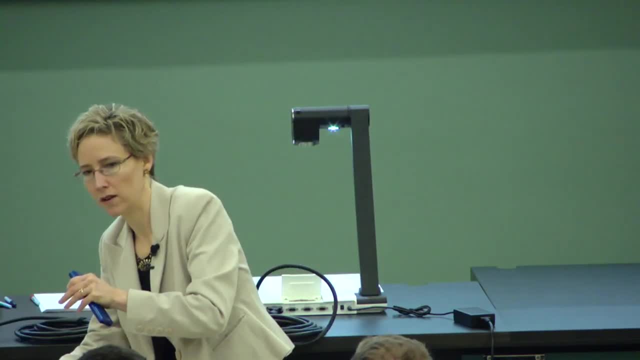 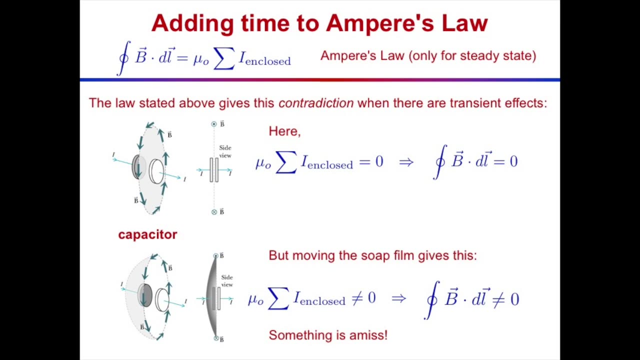 a water hose carrying water up to a bucket, and then it dumps the water in the bucket. Okay, So let's think then of applying this to a capacitor. So what do the equations tell us? The equations say: the line integral of the magnetic. 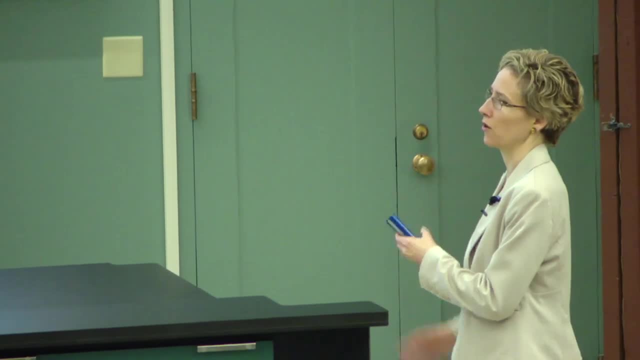 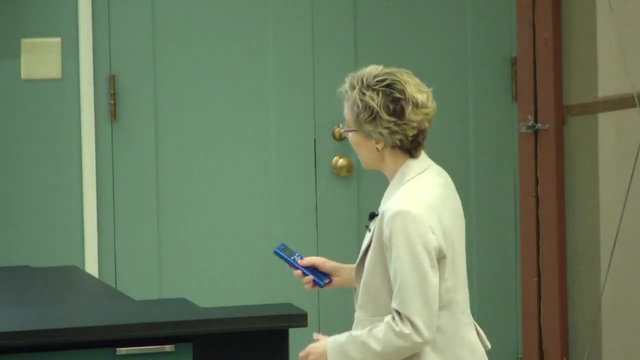 field loops back around itself. Anytime you see a circle on an integral, it is something that's closed, It's a closed integral. So this is a closed line. integral comes back to itself, And so I take that line integral and what I've told you before 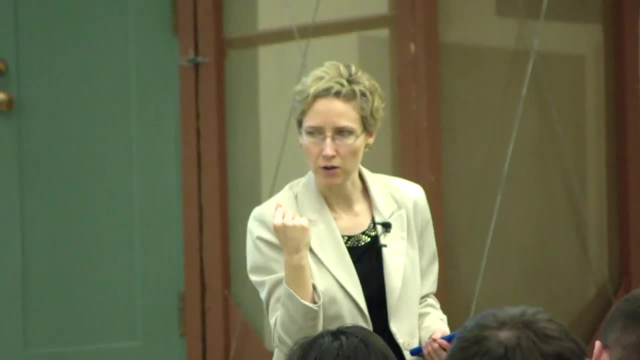 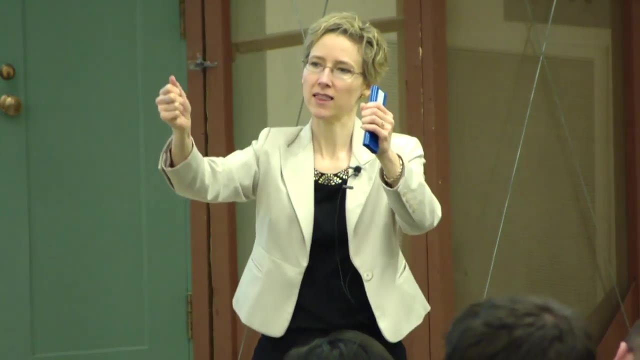 is that this current enclosed? here's the way you know whether the current's enclosed or not. take the path that the line integral's gonna go over. pretend that that's a bubble wand. okay, Now you're gonna take that wand and dip it in bubble. 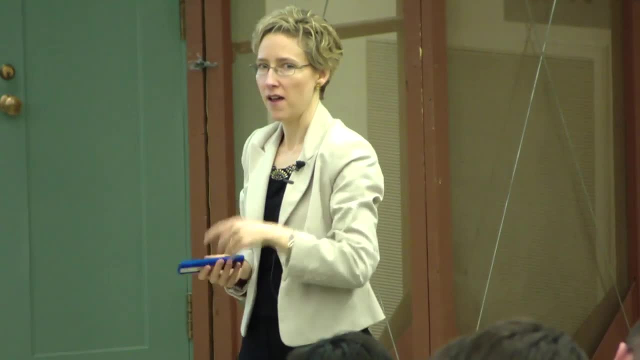 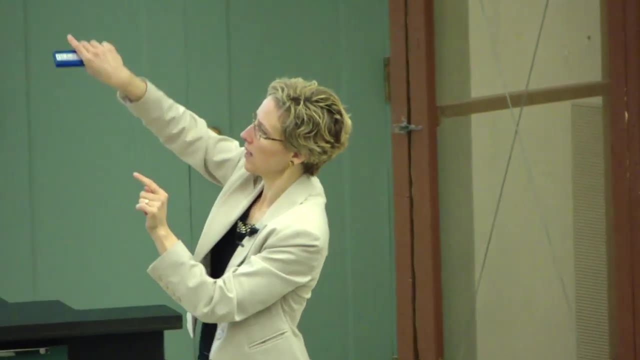 solution and then the soap film that comes out of that. if a current pierces that soap film, it counts alright. So when we had the big long wire and we thought about taking the line integral of magnetic field along the big long wire, 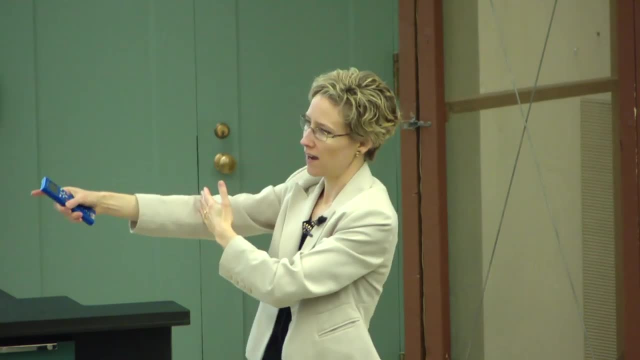 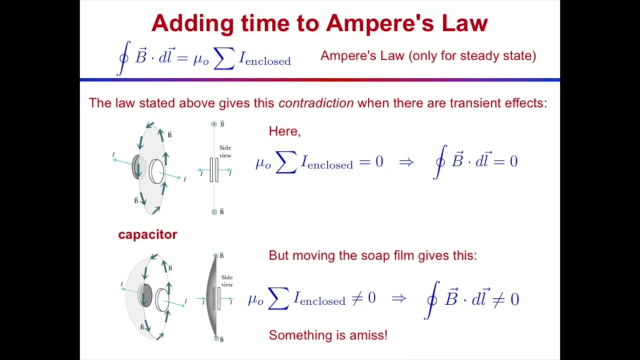 clearly the current cut the soap film. we counted that as ion closed and we knew that we had to have a curling magnetic field around it. So now do that here in the capacitor. Oh, we get something kinda strange, alright. So what? this law? 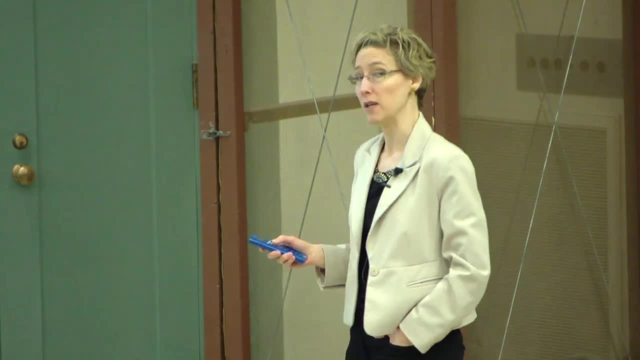 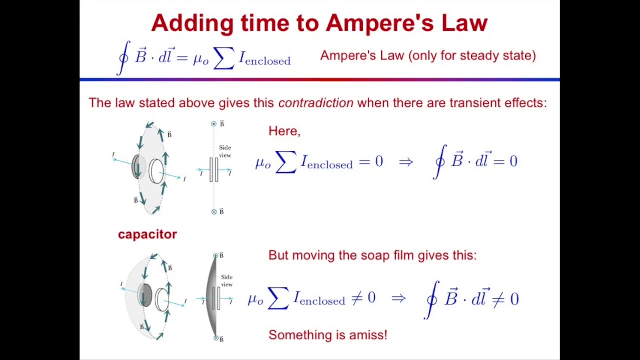 would tell us is that if the soap film passes in between the plates of the capacitor, there's no current piercing the soap film. If there's no current piercing the soap film, we would get zero contribution and we would find that the integral 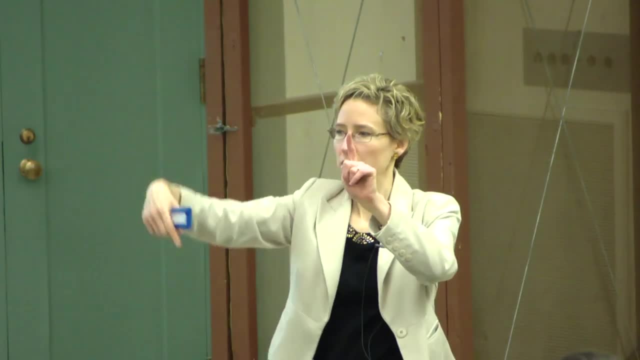 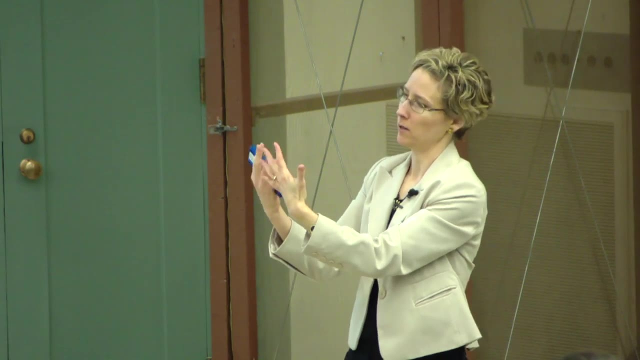 the line integral of B dot dl around the boundary of our soap film, right around the bubble wand itself, would give us zero. But now let's take the same soap film and we're just gonna blow on it a little bit, okay, So just. 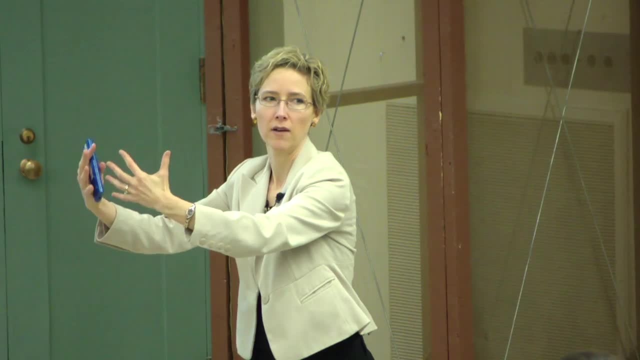 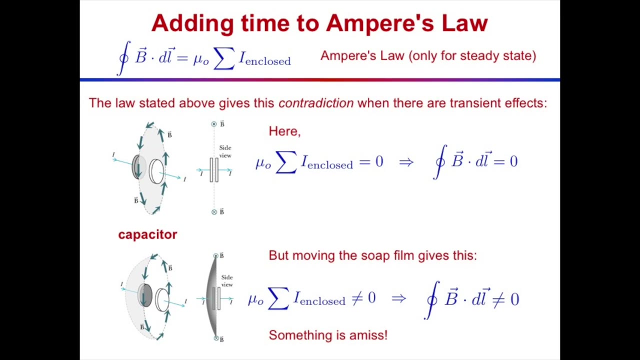 blow on it a little bit, extend it so that it passes the capacitor and now catches some of the current. Okay, so it's the same bubble wand. I've just deformed the soap bubble a little bit. I can do that. the math allows that. 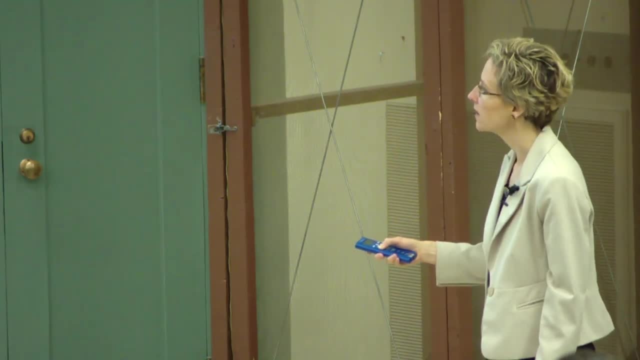 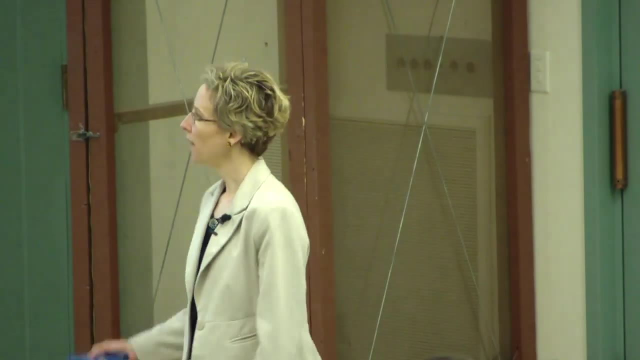 okay, So we deform that, and now we're catching some current. now we'd get a current enclosed and now we would find that integral B dot dl is not zero. okay, And this, actually this makes much more sense because 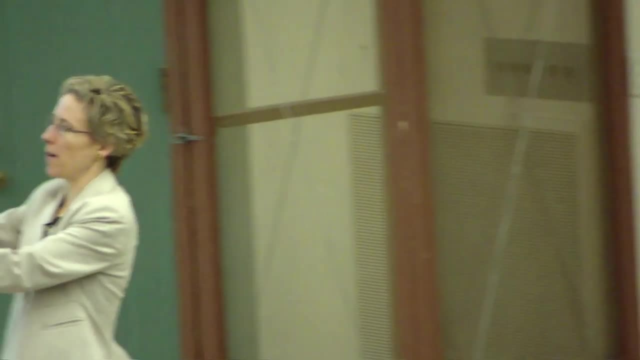 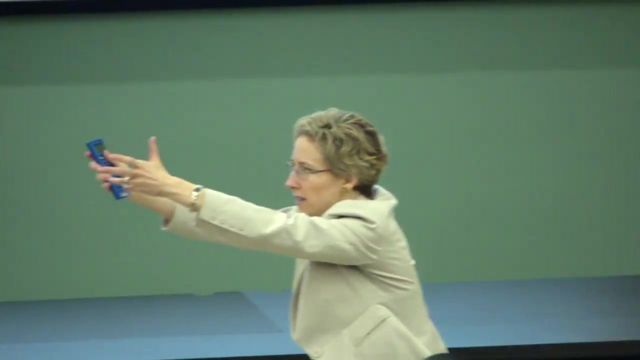 who you know. how could I possibly say that all this current leading up to the capacitor and this large curling magnetic field around it, it's not gonna just go away when I get to the capacitor. okay, So the curling magnetic field continues on unabated. 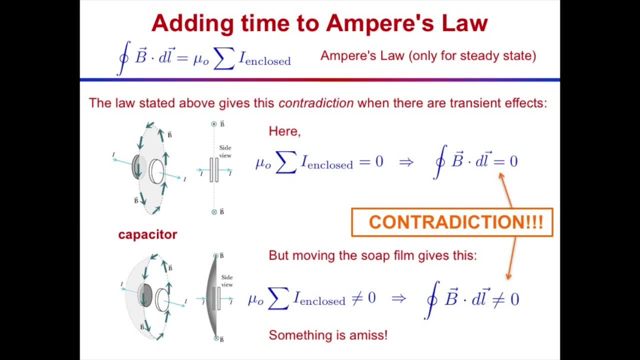 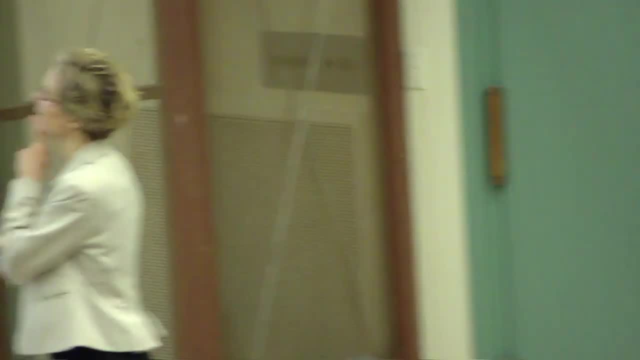 So this is what we call a paradox, right? We've got a contradiction in these lines of reasoning, and so something is amiss. the equation has to be updated, and what's missing is the time dependent term that Maxwell added to these equations. 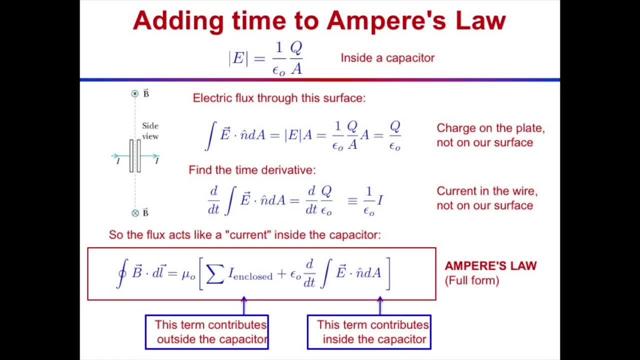 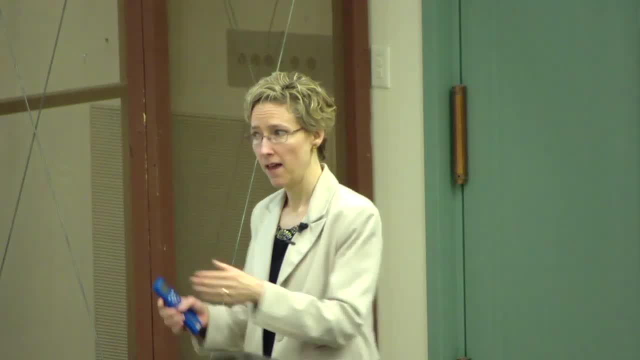 So here's what we need to do to fix it. We're gonna add time to Ampere's law, and what we're going to see is that we need to take into account that, while the capacitor's charging, the electric field inside of the 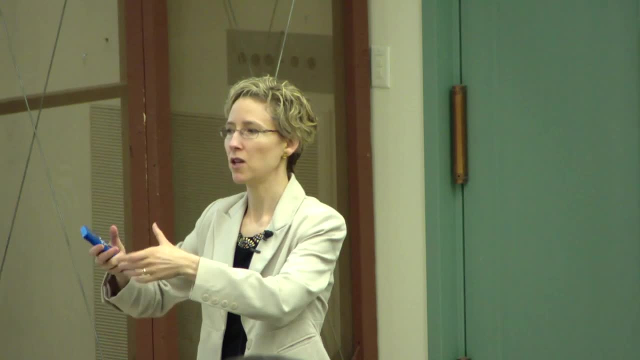 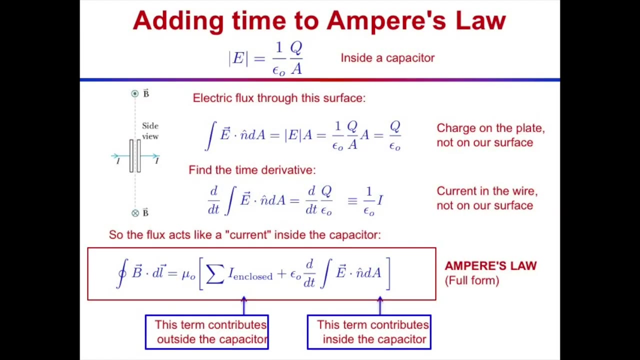 capacitor is increasing, which means there's a region of space where the electric flux is increasing, So that time dependent electric flux is what's gonna save the day. So let's calculate the electric flux inside the capacitor and then we'll calculate the time derivative of the electric 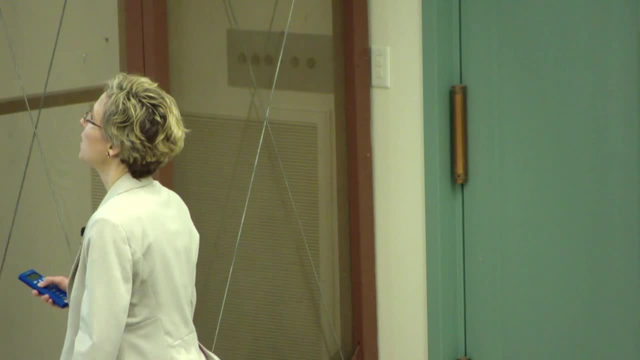 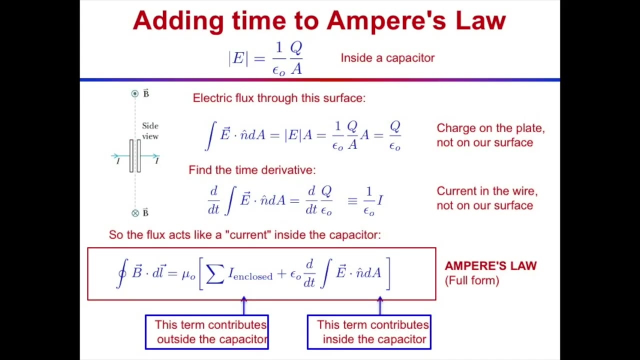 flux and we'll see that it's the piece we need to solve the puzzle. So inside of a capacitor the electric field is 1 over epsilon, naught, Q over A, Alright, and this is the electric field deep inside a large parallel. 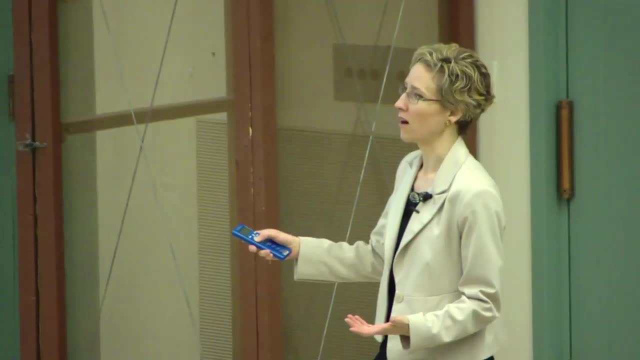 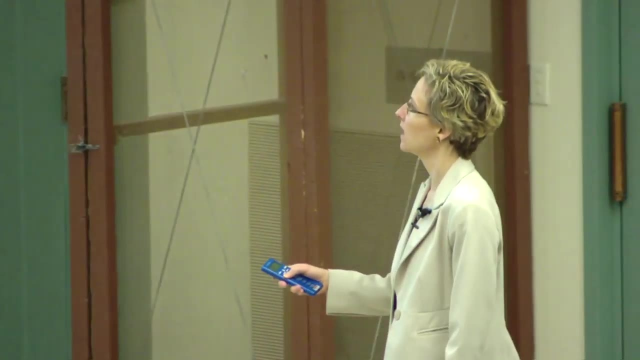 plate capacitor. You know there are also fringe fields that are typically negligible, so we'll focus on this piece that's deep inside the capacitor. So the electric flux now through our surface. alright, what we're showing here. the dotted line is where the soap film is now. 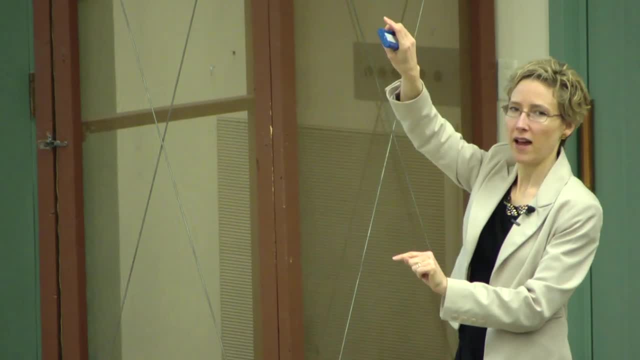 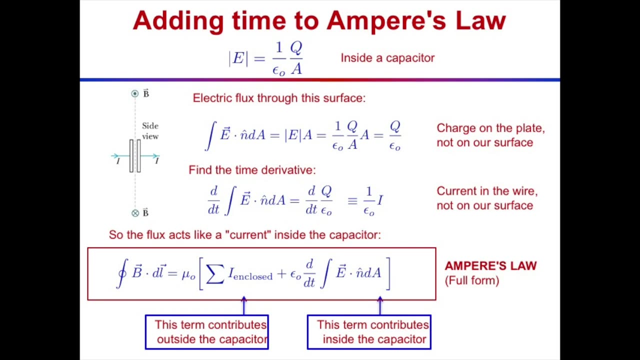 inside the capacitor and I've got the ring okay, over which I'm gonna measure. B dot DL is far away from this. alright, So the piece of the electric field then that contributes is not over the entire area of the soap film. 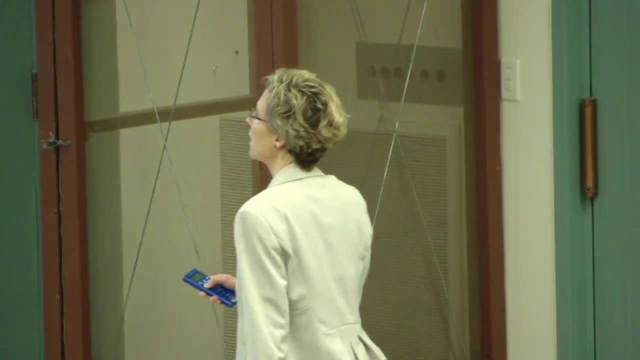 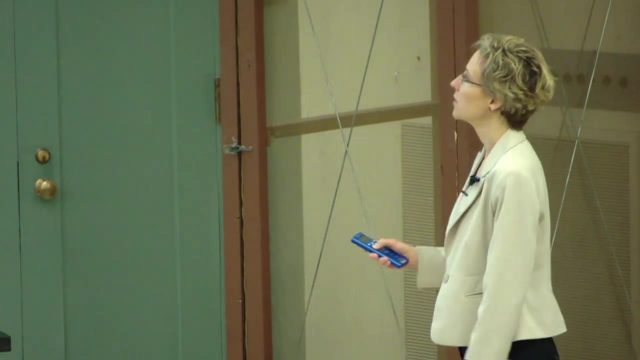 but it's only going to be where there's actually strong electric field. So here integral E dot N D A is going to end up being the electric field inside the capacitor times, the area of those plates. So E times A, and that gives me the E itself. 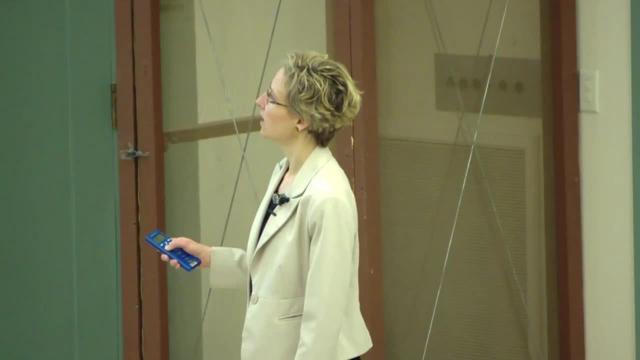 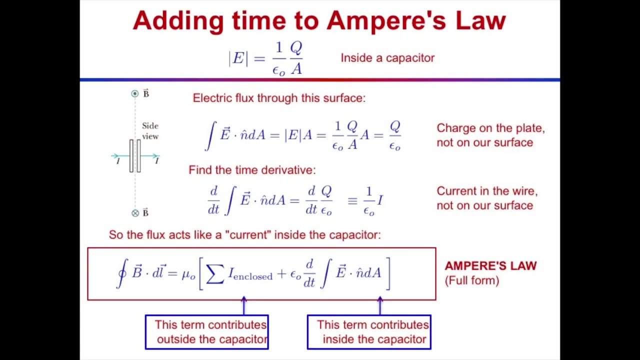 inside of a capacitor is Q over epsilon naught A times this area of the capacitor plate. that's the flux. okay, that's the electric flux through that surface. And now the A's cancel and I get Q over epsilon naught. 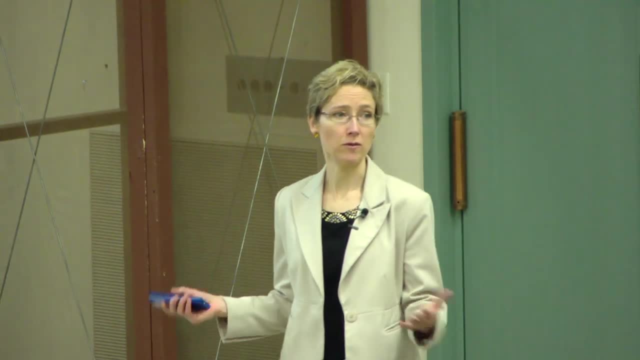 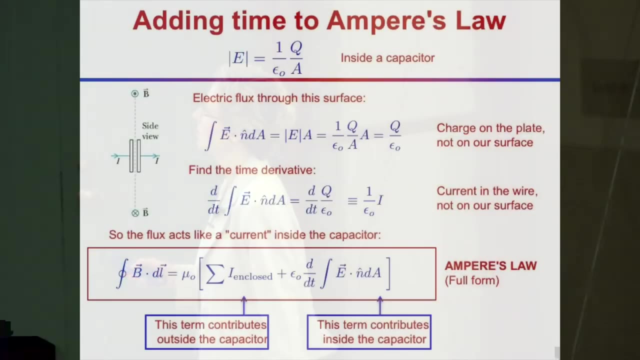 where this Q now refers to the charge on a plate, It's not where our soap film is, but it's the charge that's next to the soap film. So now find the time derivative of that. So now I need D by D, T of. 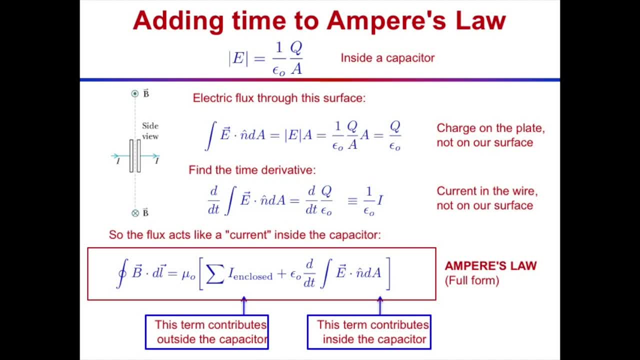 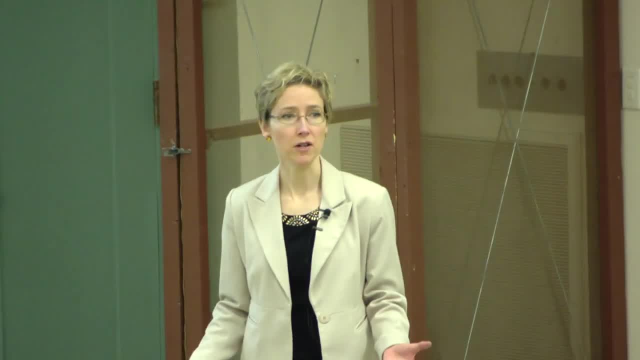 electric flux, which is just gonna be D by D, T of Q over epsilon naught. Epsilon naught's a constant, it comes out of the derivative, and D, Q by D T, you might remember, is current. Okay, it's just. 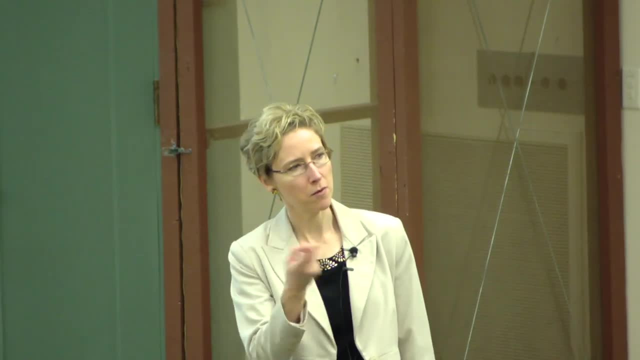 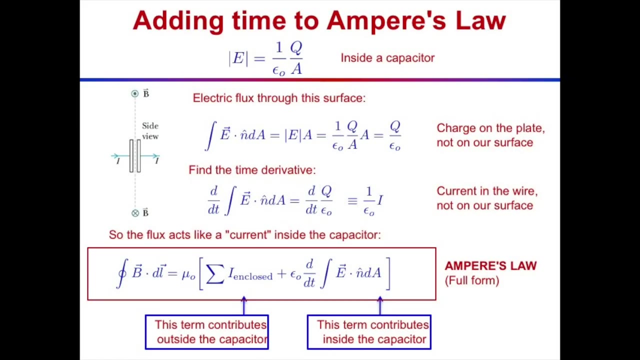 another way to state current Current is charge per unit time moving by, which is formally a time derivative of the charge. So D Q by D T gives me current. And again, this is current in the wire, not on the surface, so it's something. 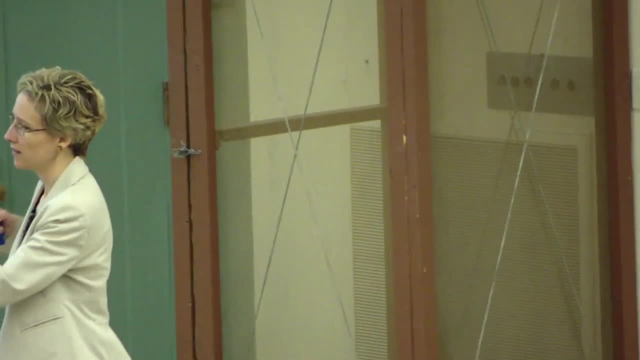 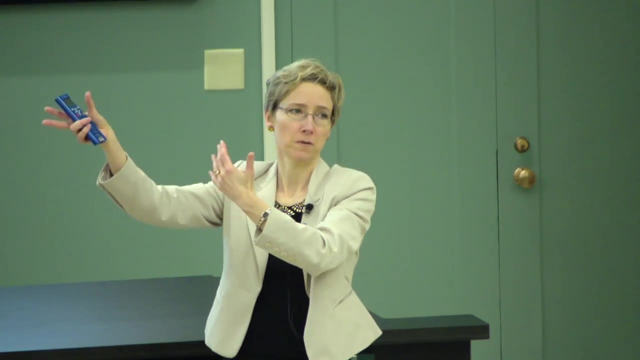 that's happening nearby the surface- not right on the surface- but the current that's coming up to the capacitor is charging the capacitor, and as the capacitor charges, the electric field inside of it grows, And so of course we can then attribute. 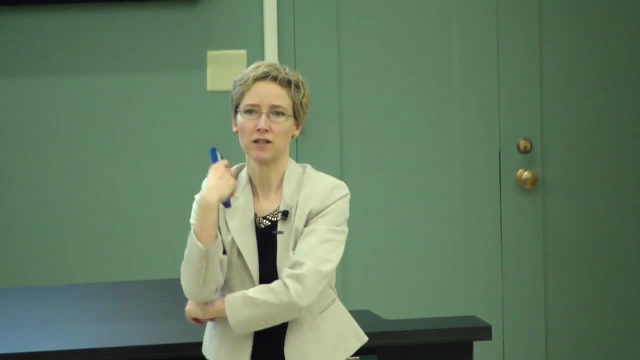 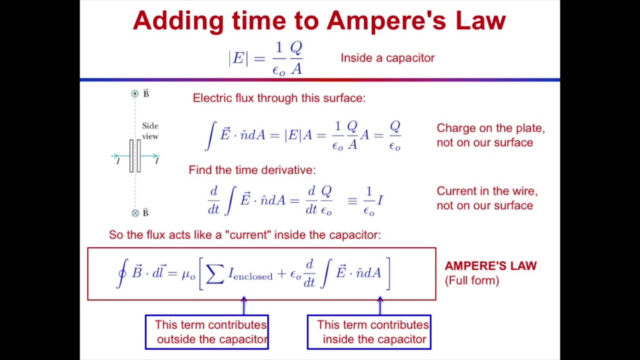 right, the current coming in is what gives me the changing electric flux inside. So that's why those are determining each other. So the flux inside kinda takes the place of the current. So if I add, then in this piece here epsilon naught D by D T. 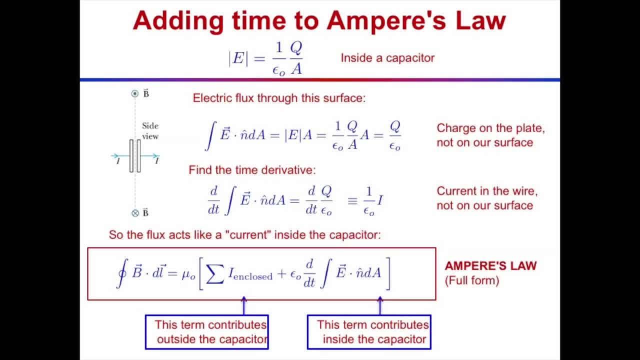 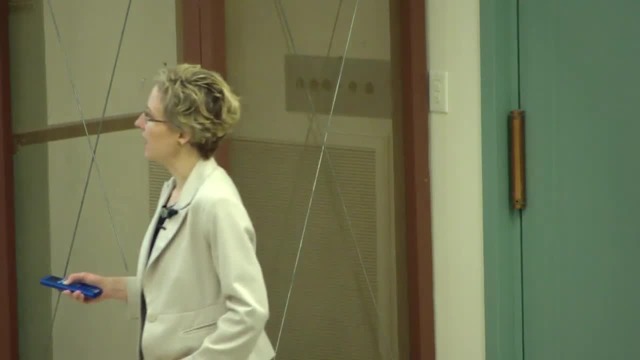 integral E, dot N, D, A. that gives me the full Ampere's Law, okay, which now gets to be called the Ampere-Maxwell Law, So basically outside the capacitor. so if I think now of the geometry we had before, where I had 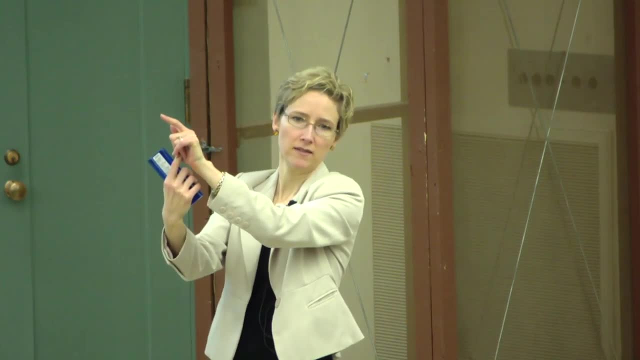 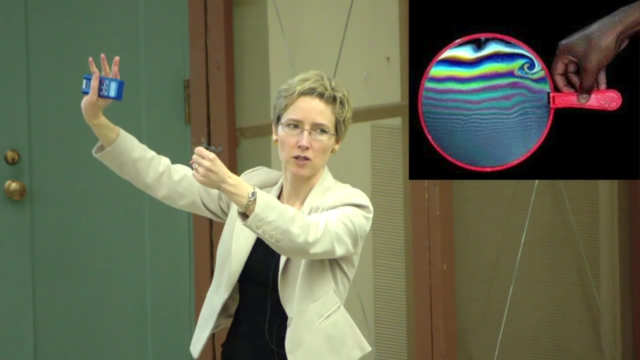 I'm gonna be taking integral B dot L around a line right, a closed line that then forms like the ring of a bubble wand. dip that in bubble solution and take the soap film. So now whether the soap film goes straight through the capacitor. 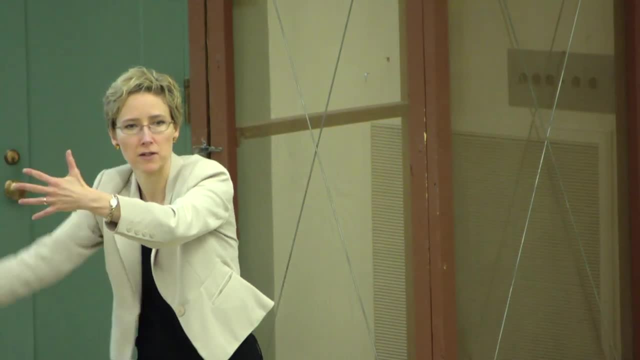 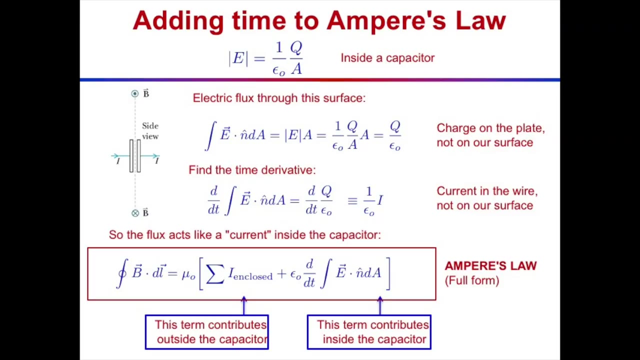 or whether the soap film is extended a little bit to go beyond the capacitor and catch the current. either way, it's going to give us the same integral B dot L, So the soap. so going back to our geometry here, right, the soap film will either catch 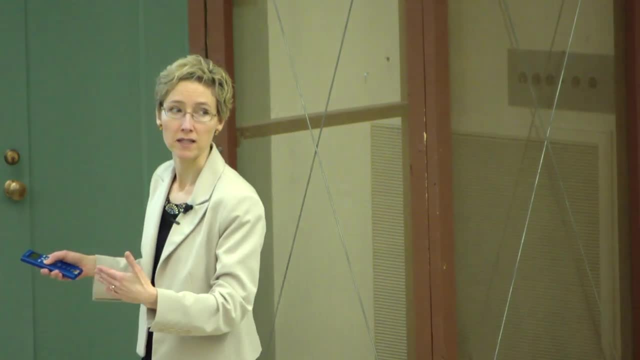 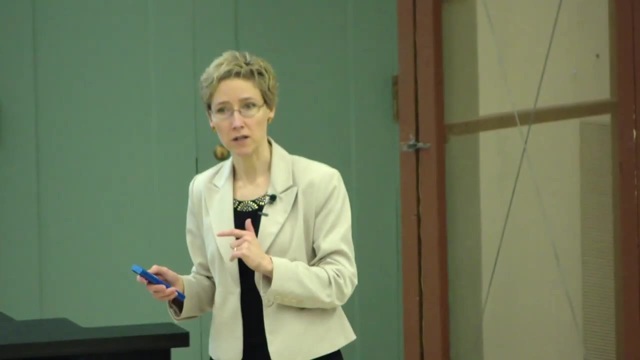 the changing electric flux in between the parallel plates of the capacitor, in which case, bam, it gives the right contribution. or, if we deform it a little bit, it'll catch that current piercing it. So, independent of which contribution it catches, it still gives the right integral. 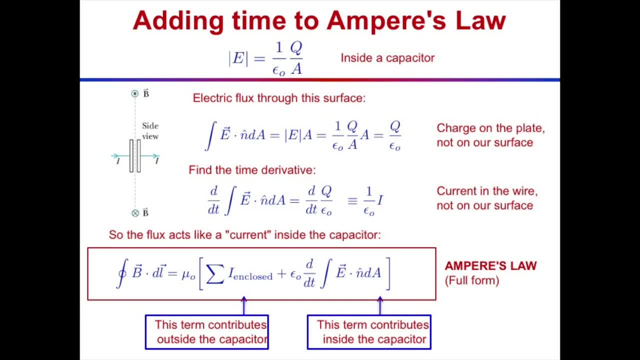 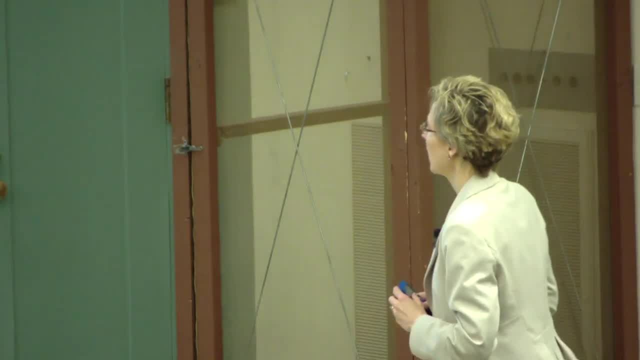 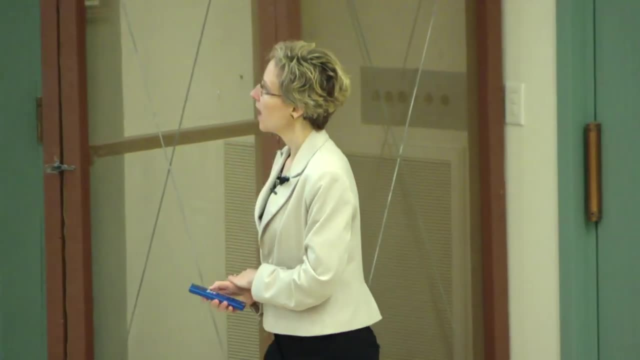 B dot D, L. okay, So that completes the equation. Do you have any questions about that so far? Okay, Alright, so this is now the full form. That's the Ampere-Maxwell law. that was the last piece in the equations. 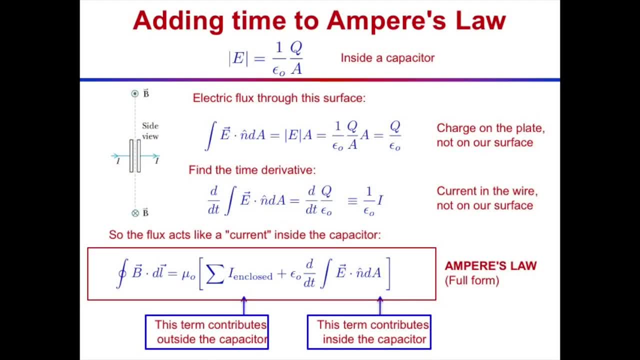 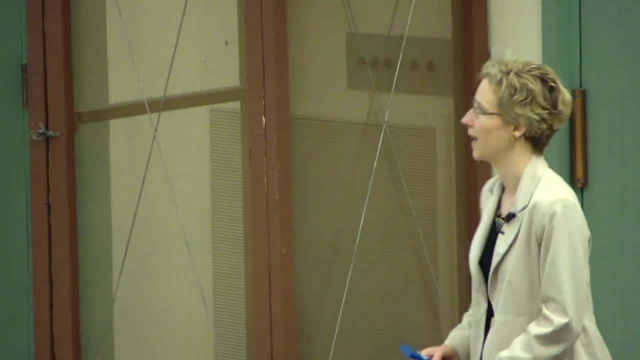 So this is it, this completes it. This slide now, this is the slide that if you snatched it and you ran back in time 300 years, you too could transform society. okay, So this is everything there is to know about electricity and magnetism. 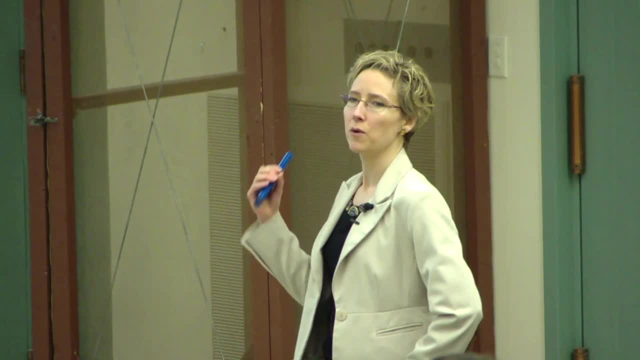 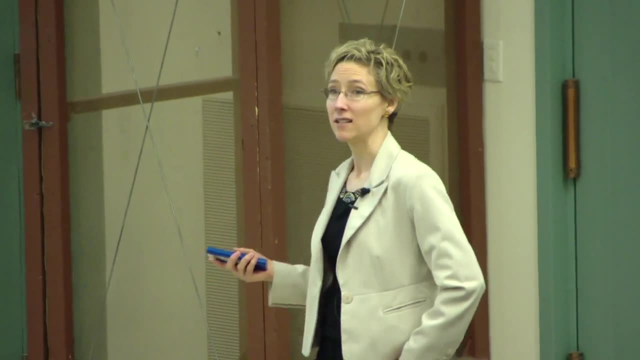 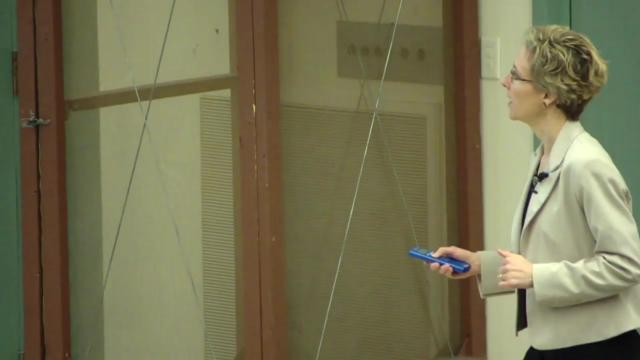 It's contained in those four laws. We also implicitly need the force law right, because the force law forces Qe plus Qv cross B. that tells us how these electric and magnetic fields affect charges. It tells us how charges affect electric and magnetic fields. okay. 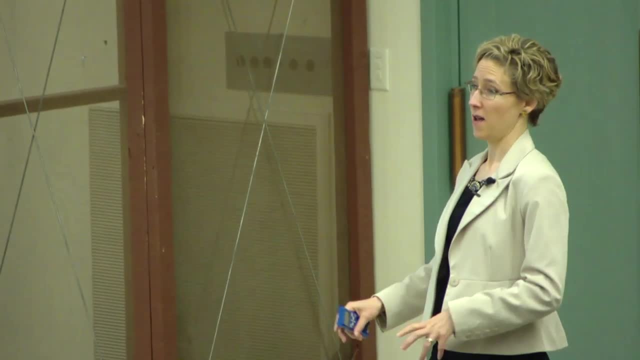 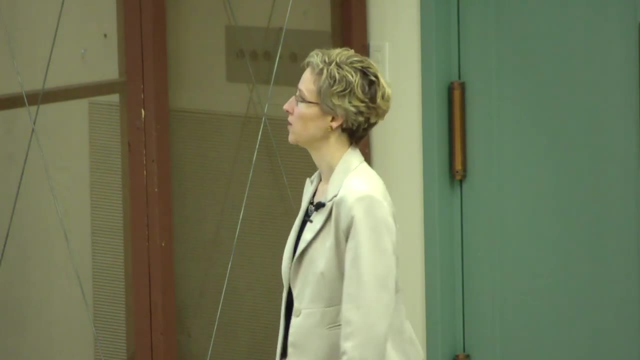 So all that together is everything we need to know and, as we said, this basically empowers a global society, right? It gives us everything from light to radio communications, to wireless communications, to the internet. okay, everything you need to know to run the 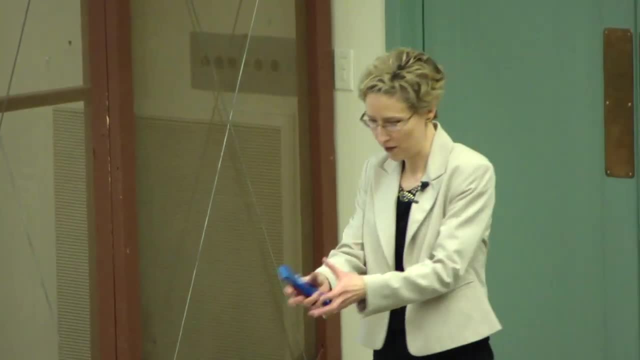 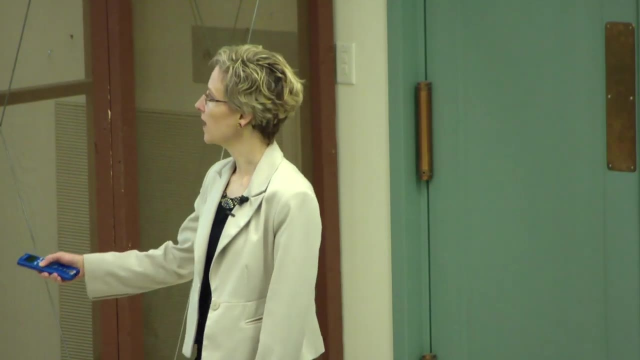 power grid. everything you need to know to make motors and all that great stuff. everything you need to know to make integrated circuits. Do you have any questions? so far? Okay, This is our last piece of the puzzle Now. okay, it's got a. 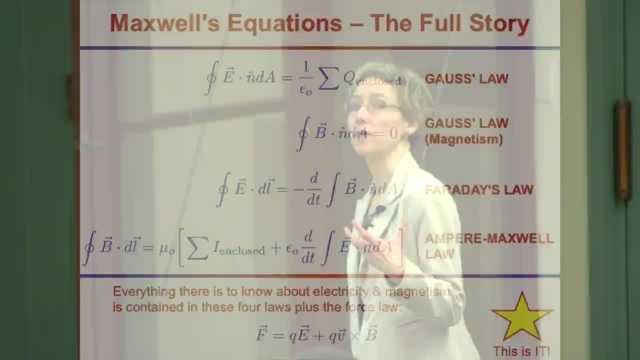 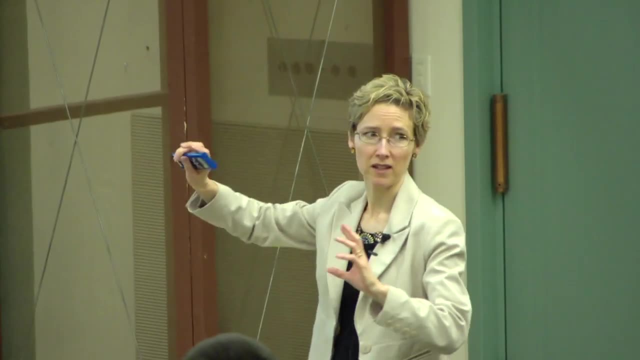 star, because this is it, and I just want to remind you of the pieces that are in here, okay, So, of course, as a theoretical physicist, I like math and you know. so some people look at the Mona Lisa and think that's. 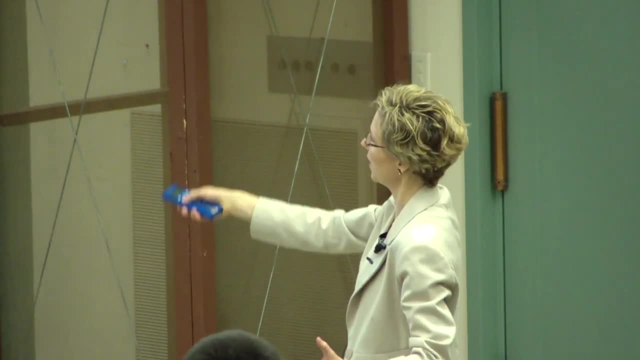 you know, a very beautiful thing. I look, I also agree that's a very beautiful thing. but I look at Maxwell's equations and I have the same, you know, reaction some people have to the Mona Lisa or to a beautiful sunset. I go. 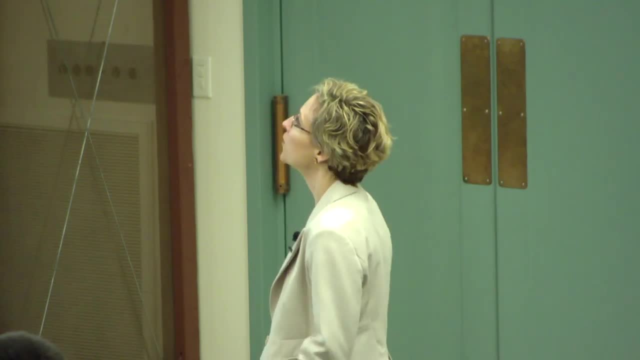 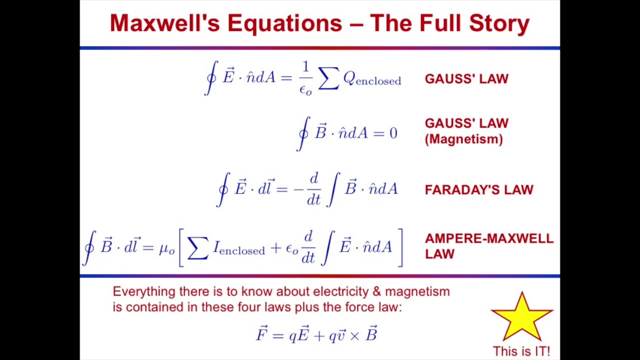 that's just the prettiest thing I've ever seen. So it is. it's so pretty, Okay, so what's pretty about it, right? So what is it? I've got two different kinds of integrals, okay, So I've got a flux. 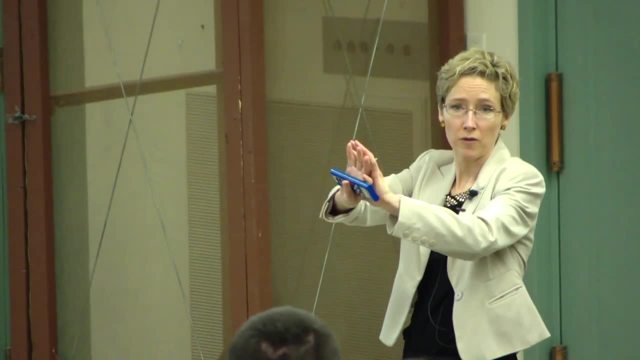 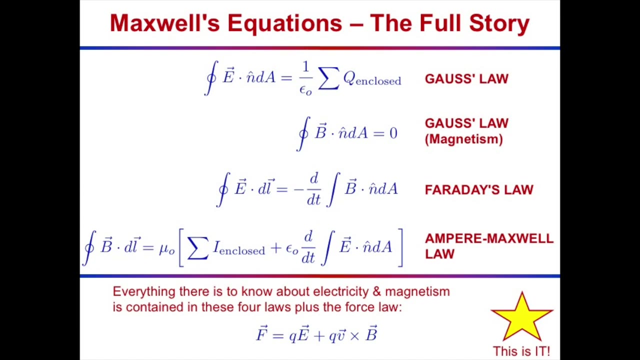 type of integral. okay, so this is about areas, so flux through areas, and these are enclosed areas, and I get one from the electric field and one from the magnetic field, so it's nice and balanced. That's very semantic, That's very beautiful And I have 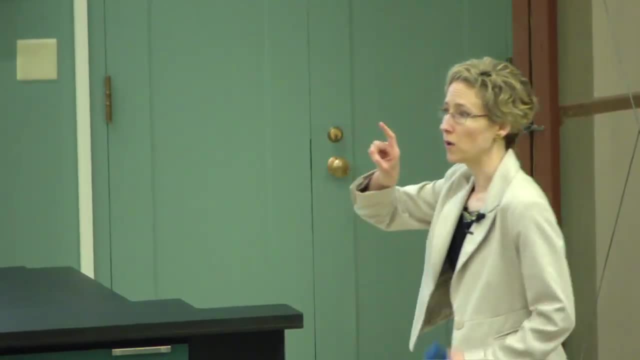 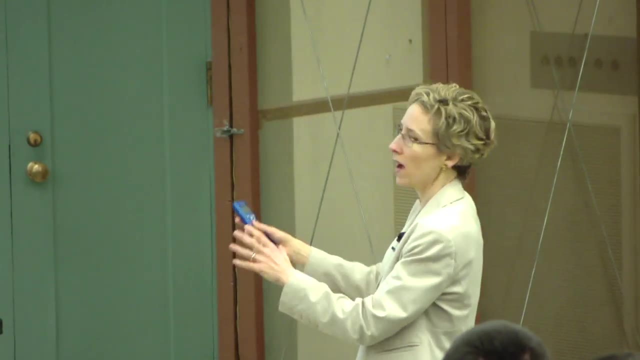 two, another kind of integral form or curl. okay, so a line, integral, that curls back around itself. okay, this tells me about curling electric fields and curling magnetic fields. and they're balanced. There's one of each, so that's very symmetric as well. And now 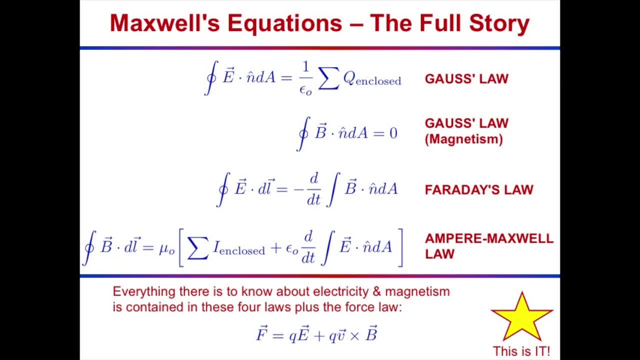 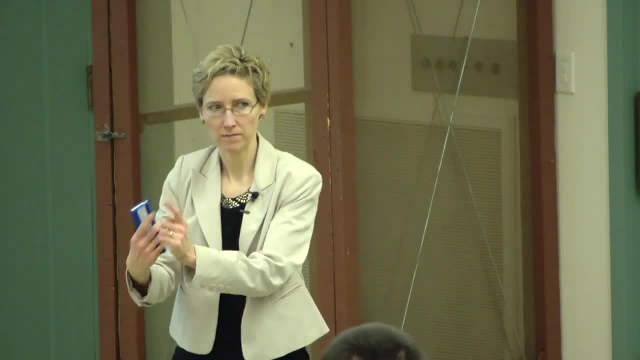 I have this nice symmetry here as well between changing fluxes. Okay, so this is the magnetic flux, and if it changes, if the magnetic flux changes, it causes a curling electric field. And then we know over here: if the electric flux changes it causes. 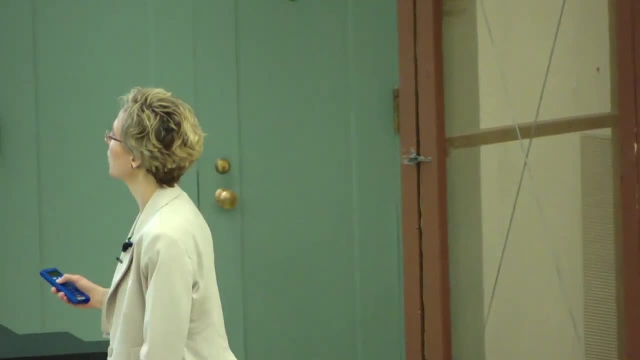 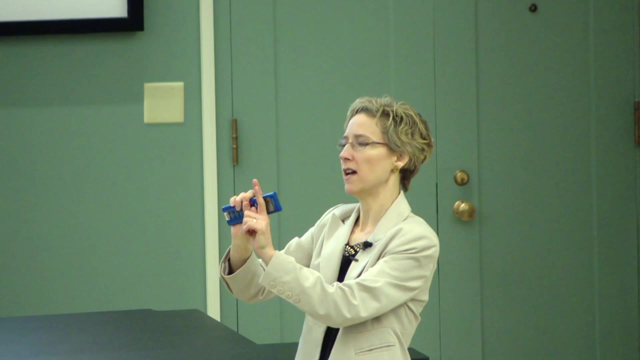 a curling magnetic field and so forth. I should also remind you of how these integrals are related to each other. right? This closed line integral alright, makes essentially like the rim of a bubble wand and then a soap film going through it. that's this. 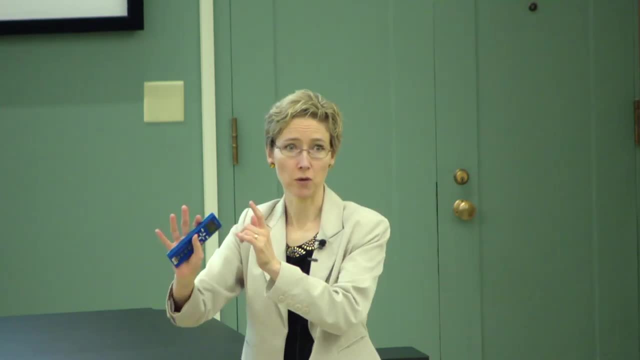 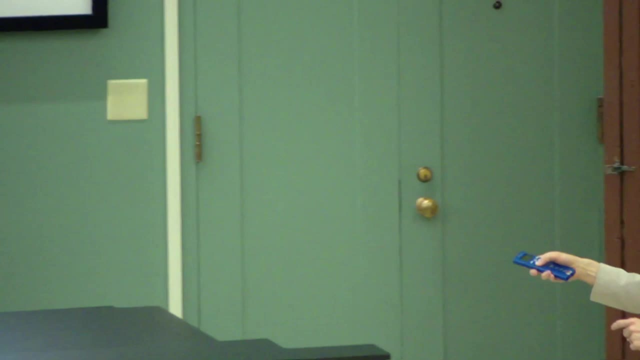 area here And you can deform that soap film and the math still works. Okay, so this area is just some area that ends on the rim defined by that Same thing here. So they're very beautiful equations and you can already see. you could kind of get a feedback. 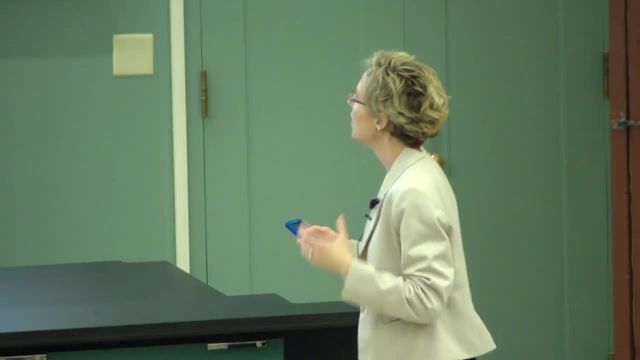 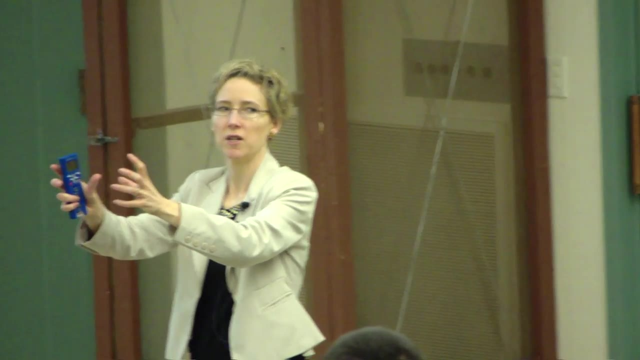 effect once you have these two time dependent terms there, right? So let's just think about kick-starting something. So let me just kind of kick-start a magnetic field somewhere and I'm going to have a region of space with a changing magnetic flux. 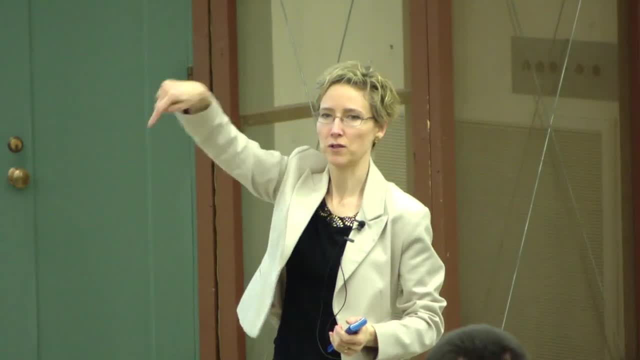 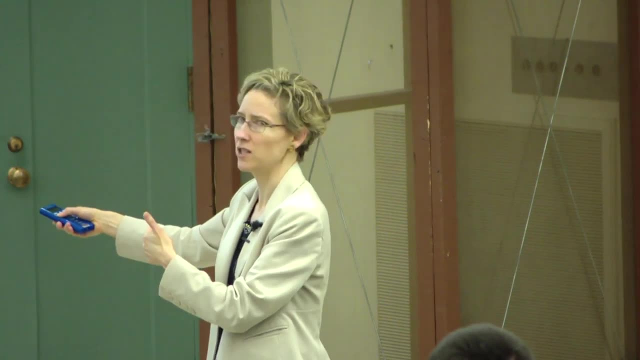 Okay, that changing magnetic flux causes an electric field to curl around itself. Okay So, and once you start a curling electric field, well, now you've got a changing electric field. So you've got a changing electric field. there's some region. 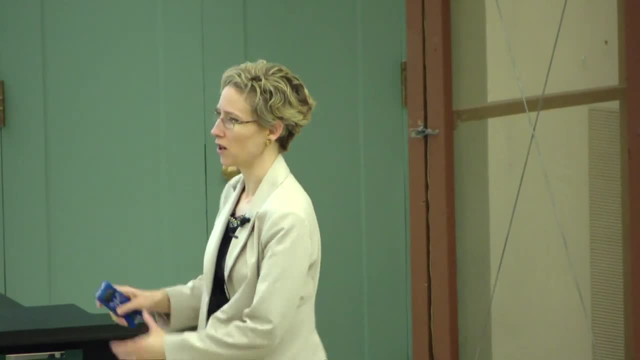 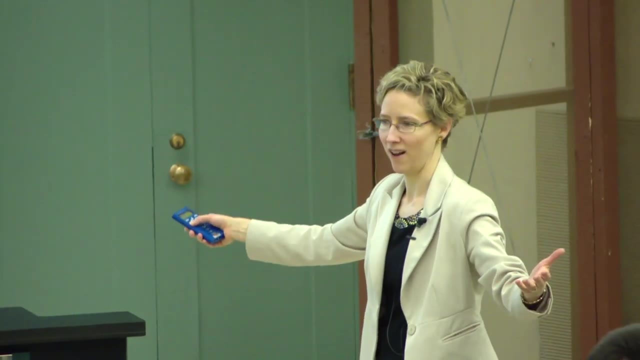 where there's a changing electric flux. Well, that changing electric flux starts off a curling magnetic field And the curling magnetic field is now changing, which means there's a changing magnetic flux somewhere, which goes on. it just loops back around. 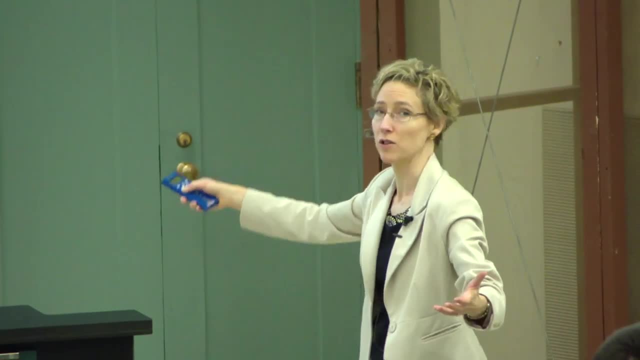 right. This causes that to happen, causes that to happen, causes that to happen, and so forth. So you can already see how you can get something that is a self-propagating wave And if we have time at the end of the lecture, 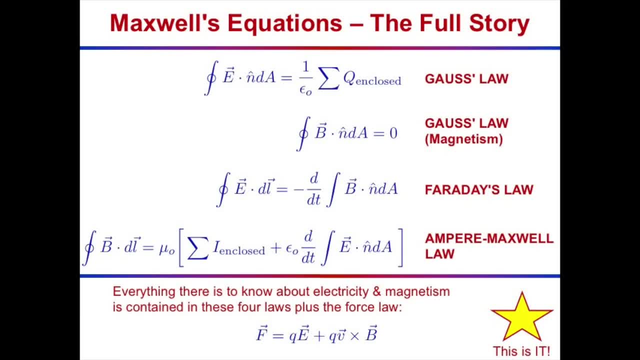 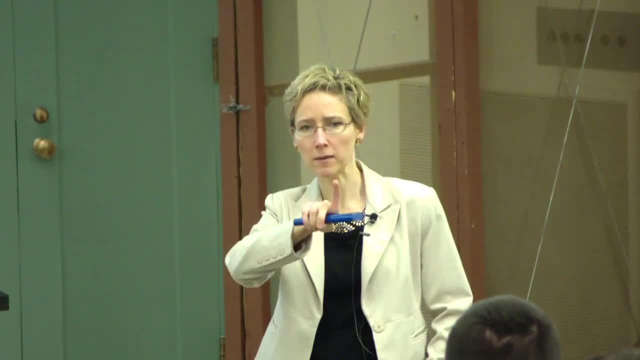 I'll show that to you. The next thing I'd like to show you, though, is how to convert these guys into their differential form, So here I'm going to take a different path from your book. okay, I'm going to skip to the end of the book, and 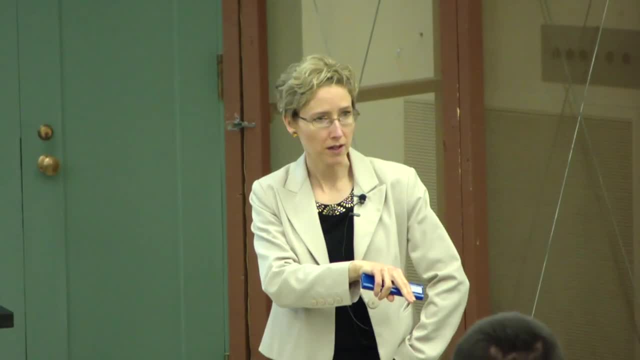 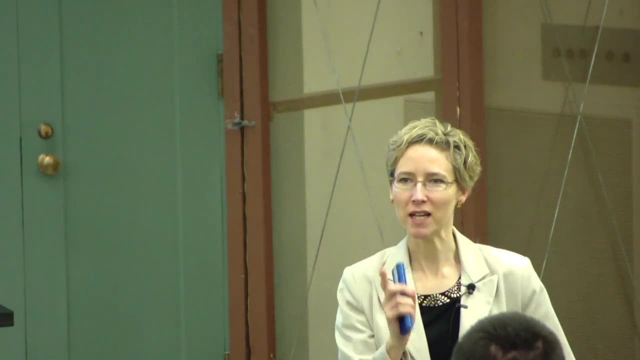 show you how to convert these integral equations into differential equations. Once we get the differential equations in place, you remember I've already told you how to solve differential equations. right, When you get a differential equation, you knock on the door of the math department and you say: 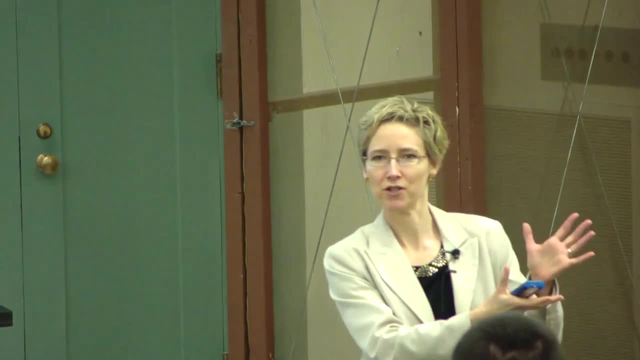 here's my differential equation. What's the solution, please mathematicians, And they tell you what's the solution if it's solved right. There are differential equations out there that we don't know solutions to yet, But if it's, 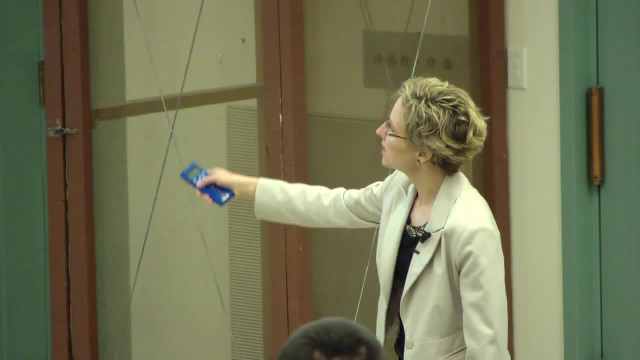 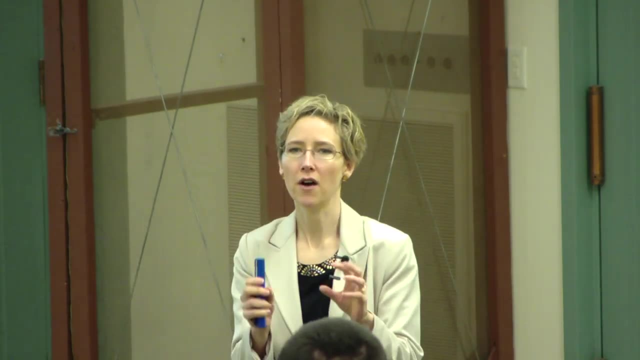 a solved equation. you ask the math department. So what we'll see is that when we convert these guys into their differential form, we'll get a differential equation that turns out to be the wave equation, right. So we'll see that we can actually 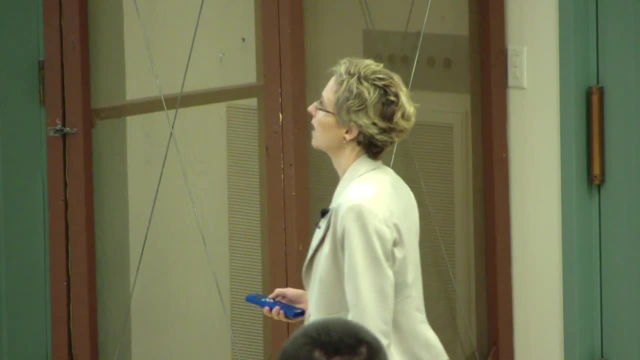 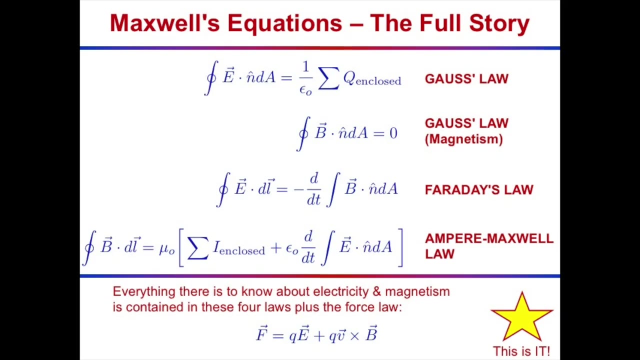 just predict light waves, electromagnetic waves, out of this stuff. So let me show you how to get the differential form. Basically, it amounts to taking derivatives of these integral equations, But let me show you how to do that in the very controlled calculus methods that you already know, okay. 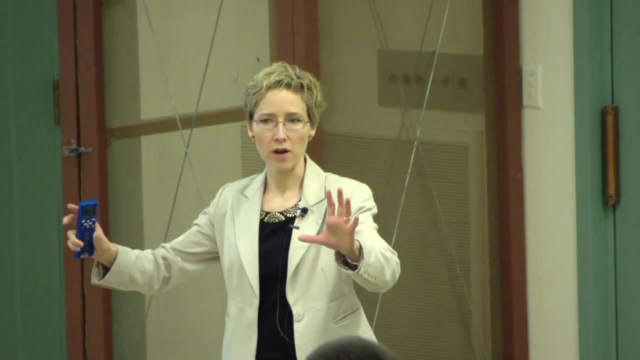 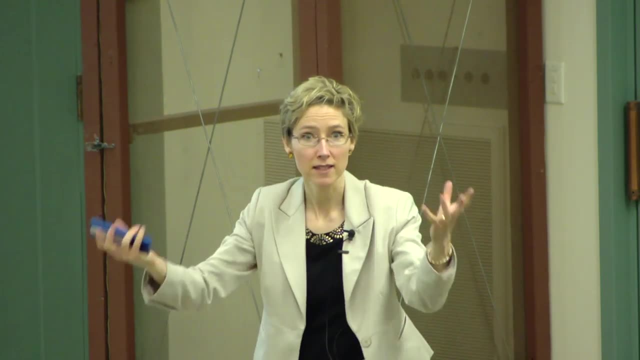 When you're going to take a calculus limit, what you need to do is you define geometries and then you're going to shrink those geometries down And then in the limit, calculus happens right. So let's think about Gauss's. 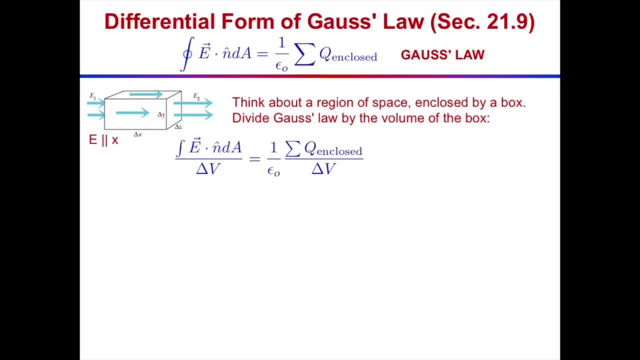 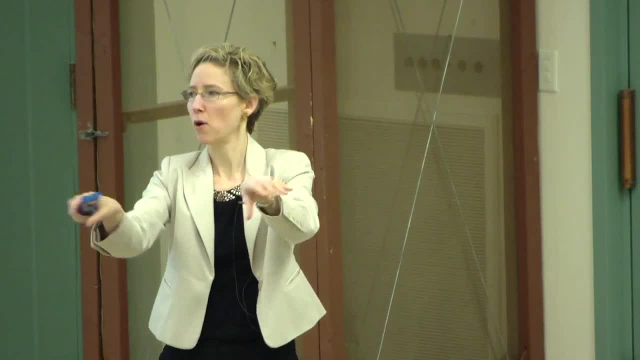 law first. So Gauss's law tells me that I need to think about some sort of charge, okay. And then if I enclose that charge with an area, the electric flux poking through that area is directly proportional to the amount of charge that's inside. 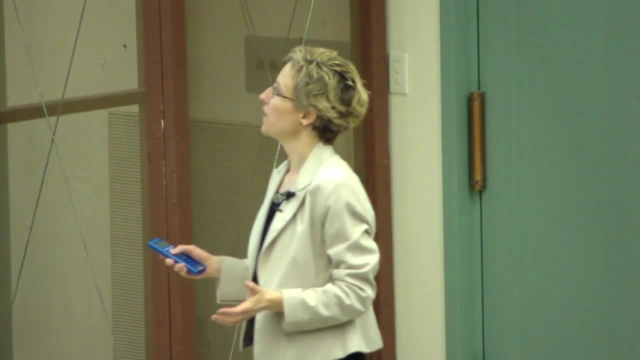 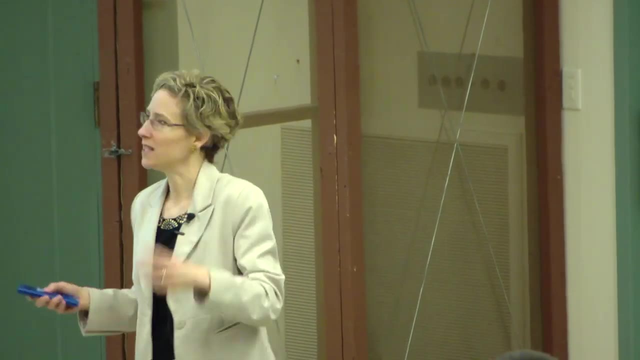 the enclosed area. So now think about a geometry that's going to be easy to take limits of right. If I'm going to take a calculus limit, set up the geometry to be easy. So in this case, I'm going to think about a region of space enclosed. 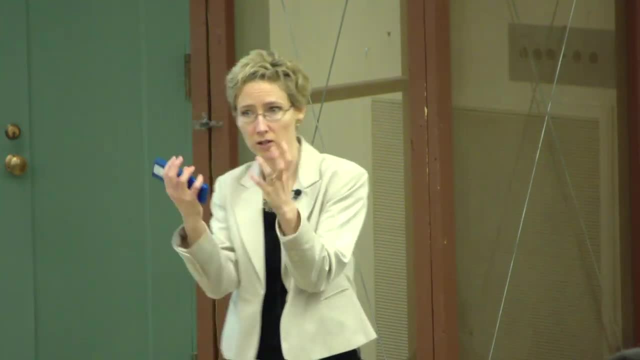 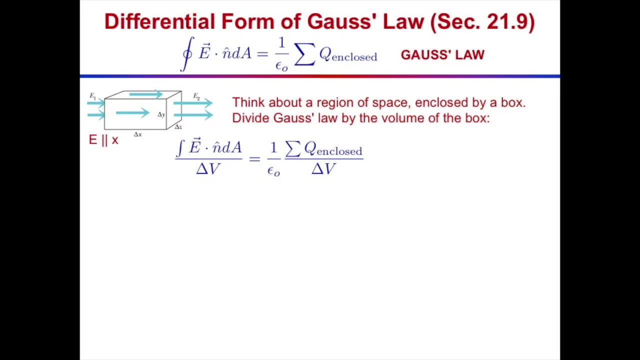 in a box. Now I'm going to make the box a nice square box, okay, So it's got a delta x that's lined up on the x-axis A delta y is the distance along the y-axis. Delta z is the distance of this box along the z-axis. 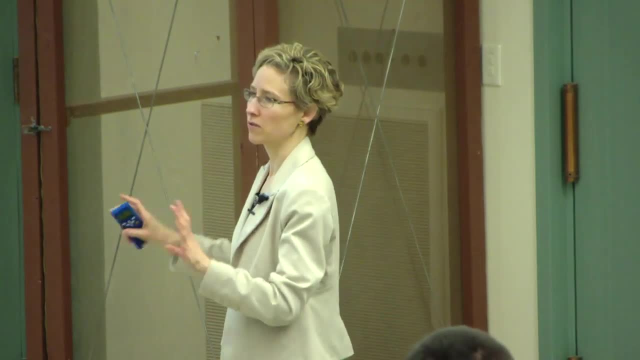 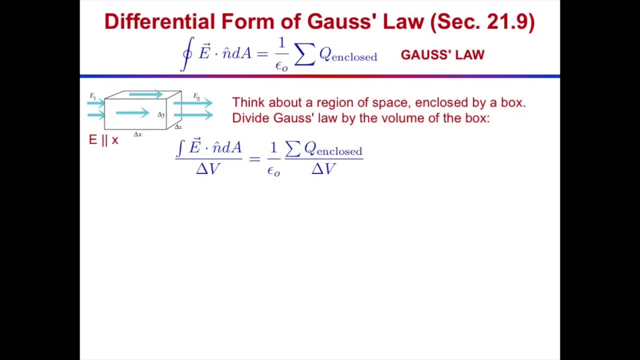 And I want to think about taking Gauss's law and just divide it by the volume of that box. okay, So I take the electric flux, divide it by delta v. I take the right-hand side, one over epsilon, naught, charge enclosed and. 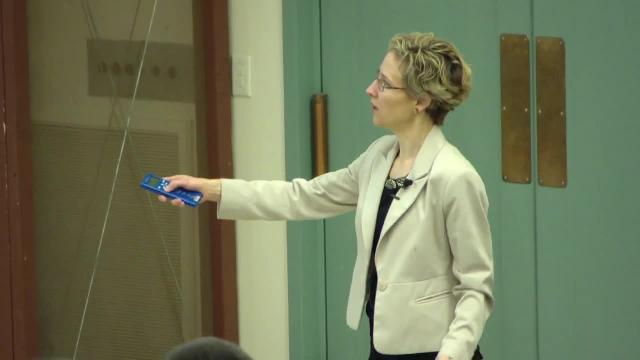 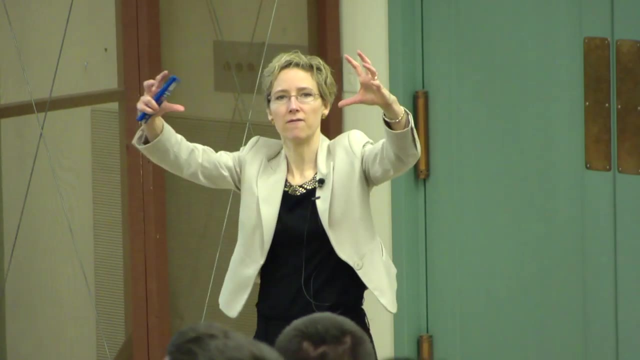 divide that by delta v. So far I haven't done anything magical. I just divided Gauss's law by delta v. Okay, Next, some calculus is going to happen. So now I want to take the limit that that volume goes to zero, And as that happens, 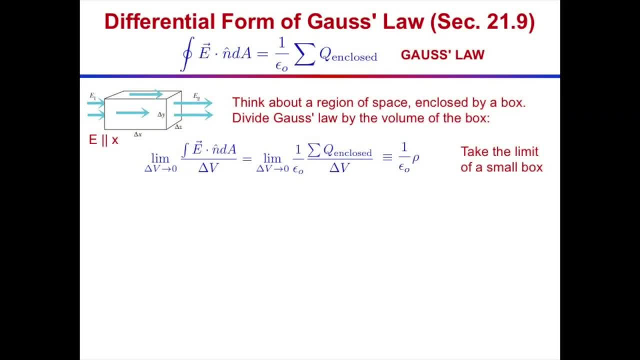 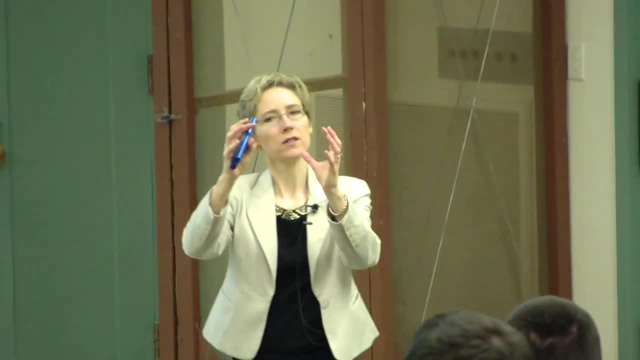 we'll see that some differential equations come out. So take the limit as delta v goes to zero. okay, On the right-hand side here, as I take the limit that delta v goes to zero, I'm going to enclose less and less charge. 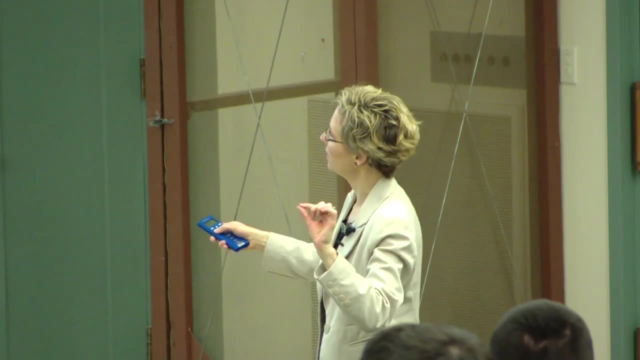 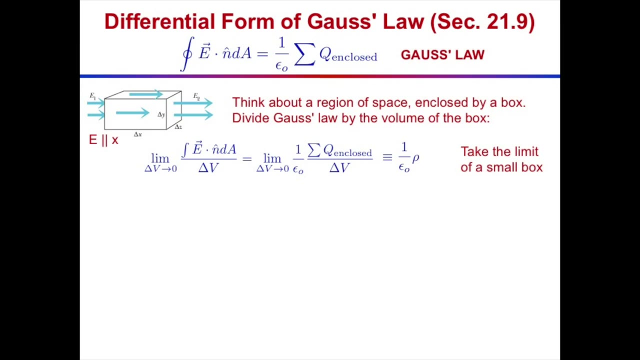 all right, But in the limit. that becomes charge density. So this is charge per unit volume and I'm just taking a smaller and smaller volume and that becomes rho, where rho is charge per unit volume. That's just that's. 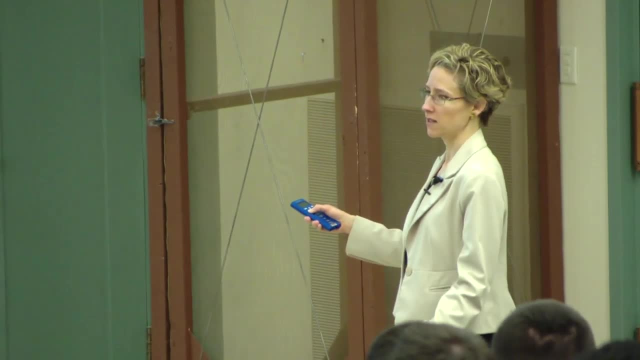 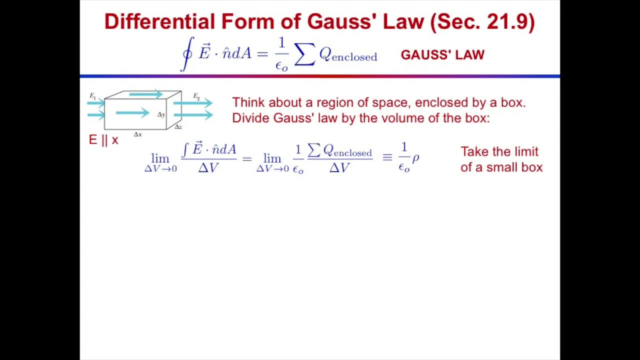 what charge density means. okay, So this becomes charge density. okay, That's just by definition. Do you have any questions about that part? Okay, So it's just by definition. Does no questions mean we're good or I need to spend more time on it? 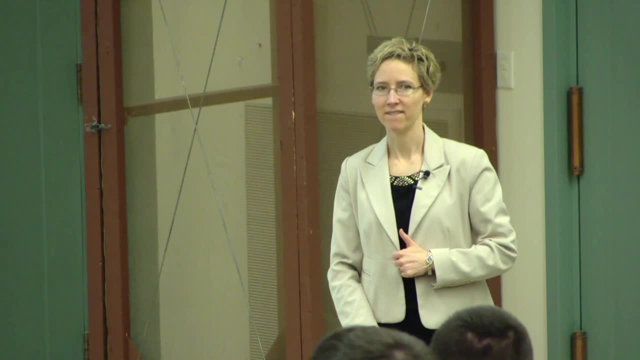 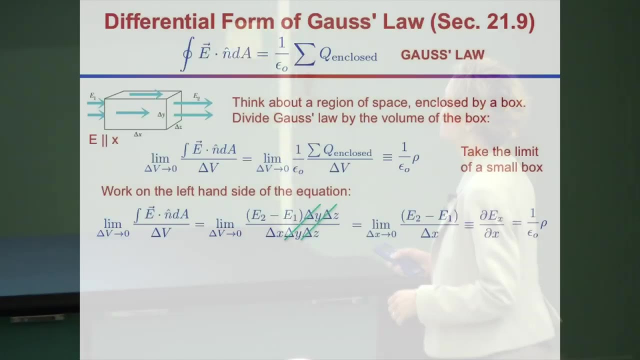 Okay, We good Going to go on. Okay, All right, I'm seeing some thumbs up, So work on the left-hand side of the equation now, and that gives me integral e, dot, d, n, d a over delta v. but I'm going to take. 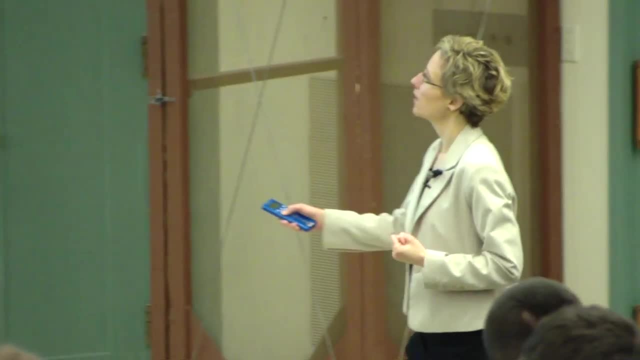 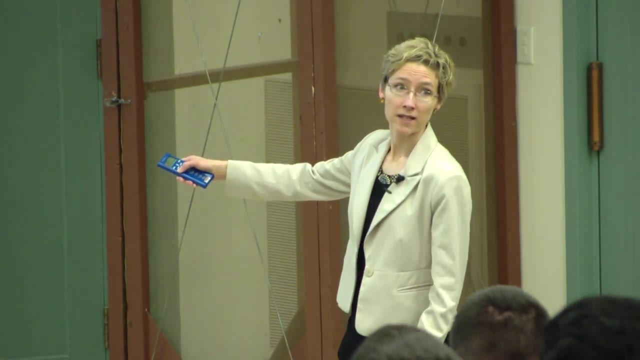 the limit now as the volume goes small. All right, So now I go back to my geometry. okay, Fifty percent of physics is drawing your diagrams really carefully. So now I just look back at my diagram. okay, I've set things up in a way that's. 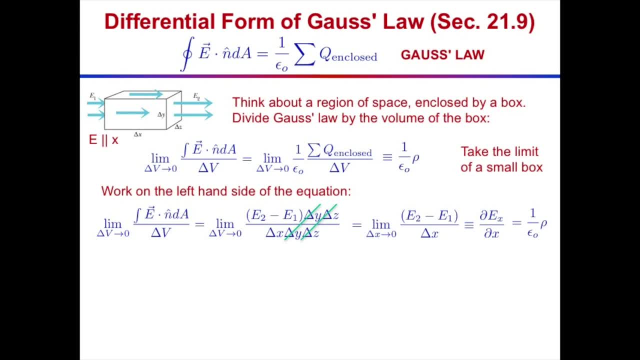 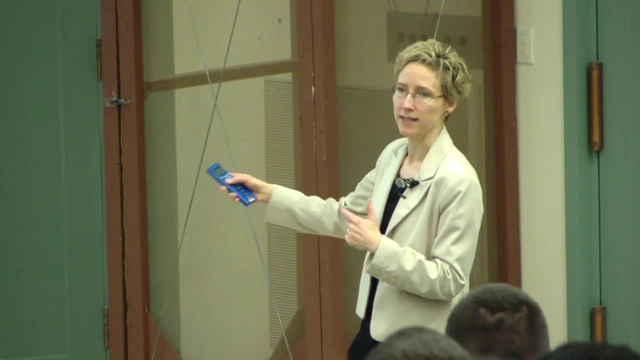 going to be easy to calculate. I set things up so that I have an electric field that's only in the x direction in this region of space, okay? And I've set my box up so that it's along the x, y and z axes. 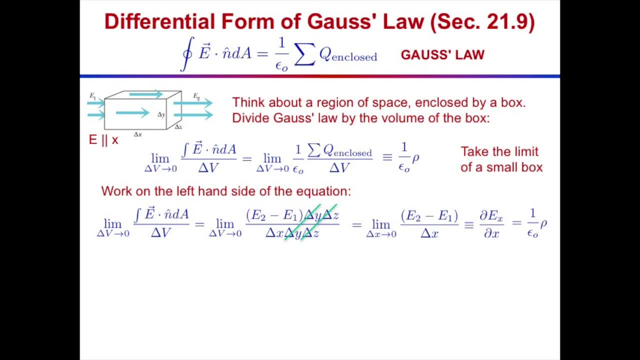 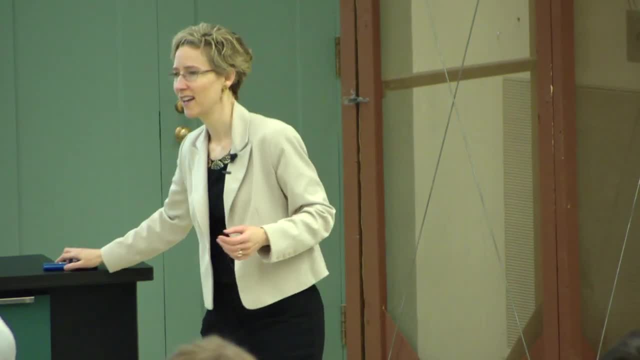 And so I have a case that's easy to calculate the electric flux. So there's pieces of the electric flux that are on, say, this plane or that plane, and there's no contribution. right Parallel nets catch no fish. so when the electric field is, 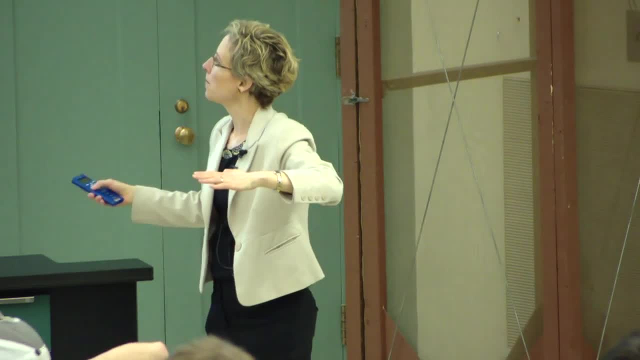 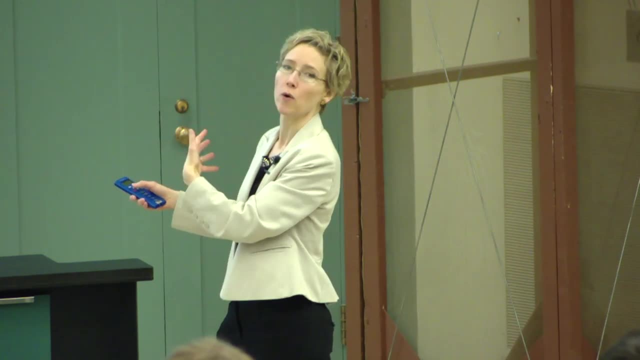 parallel to the area, there's no flux contribution. So I'm only going to get a flux contribution from the back end here, where e x is poking into it, and from the front end here, where e x is poking out of it. So let me take this piece first. This gives me. 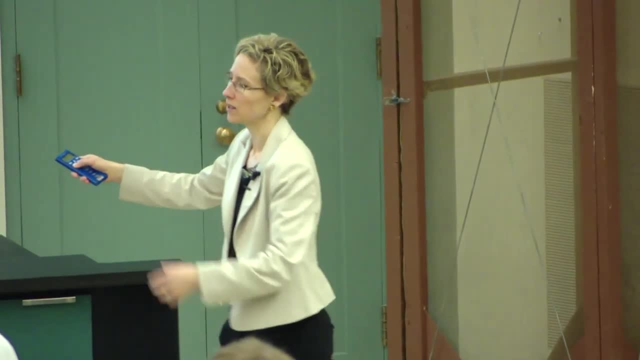 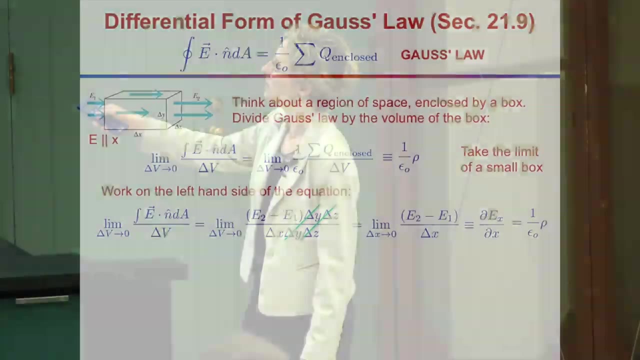 a contribution. I've labeled it over here: e 2,. okay, That's what's coming out of this side of the box And what's the area it's poking over. Can you kind of just see from my diagram This e 2 is poking. 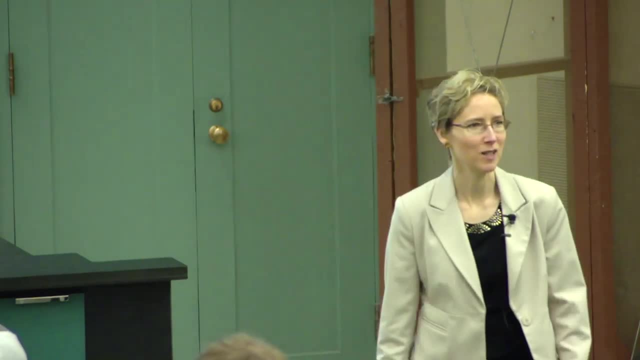 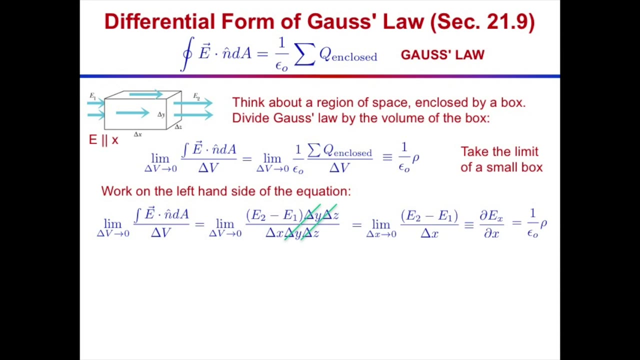 over. what's the area of that square? I set it up to be easy. So what's the area of that square right there? Yeah, exactly, So it's delta y times delta z. That gives me the area. So that's right here. That's e 2 times. 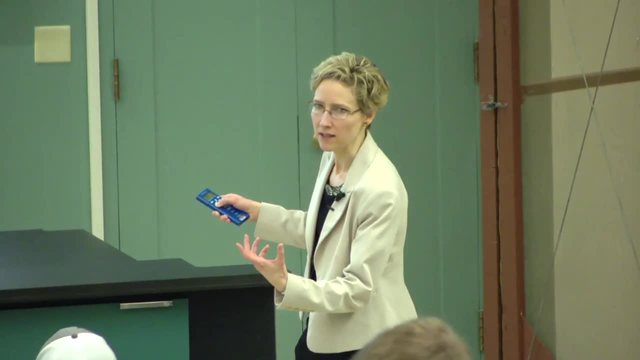 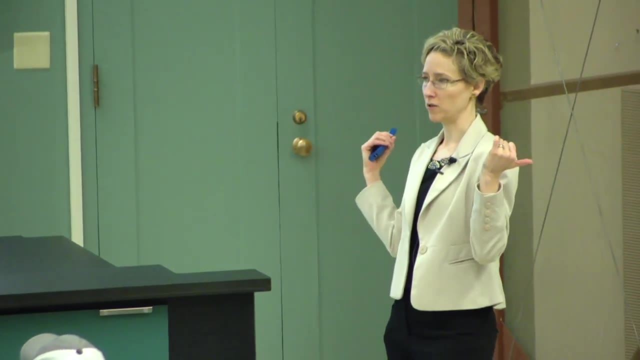 delta y, delta z On the back side, which you can't quite see in the diagram. on the back side it's the same area, but the flux is coming in. Flux coming out gives a positive contribution, Flux coming in gives a negative contribution. So there's this. 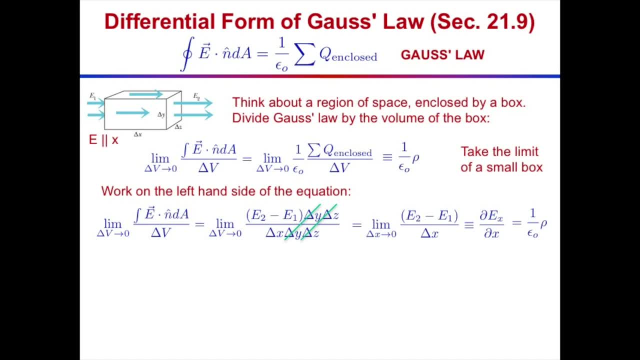 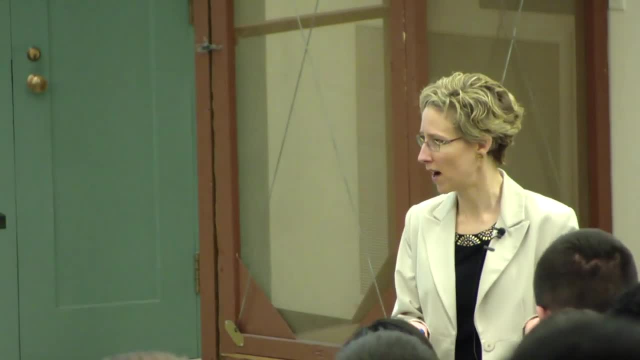 negative: e 1, delta y, delta z. okay, The other thing I'm going to do is write down the volume of the box in terms of delta x, delta y, delta z. What's the volume of my box in terms of delta y, delta x and delta z? 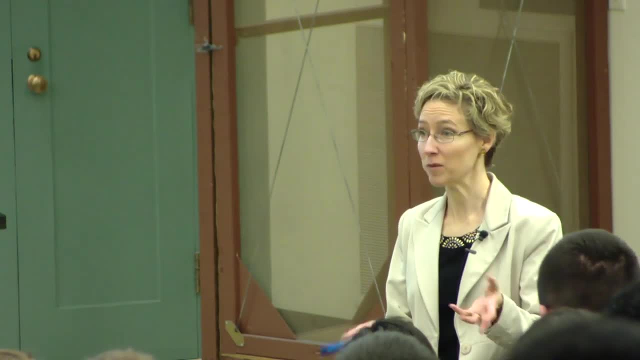 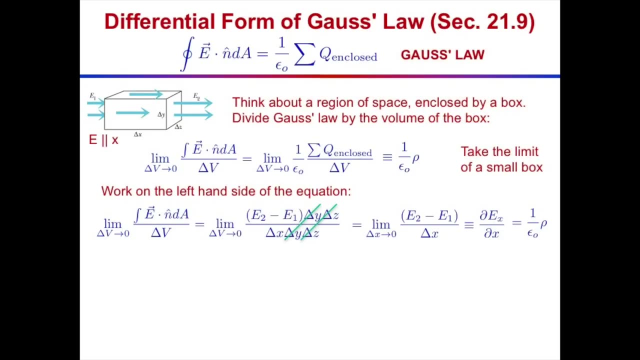 Yeah, I just multiply them together, right? So delta x times delta y times delta z, that's the volume of this box. That goes right there, And you might see already that I have a delta y divided by a delta y and a delta z divided by a delta z. 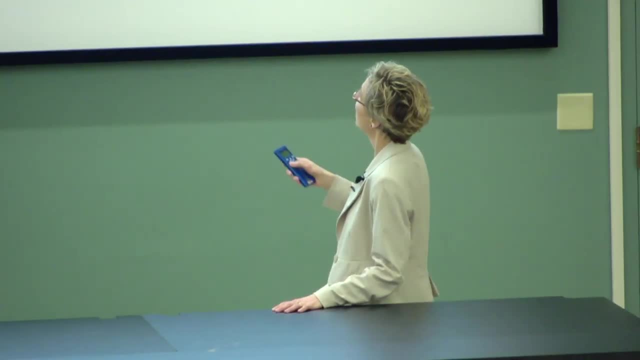 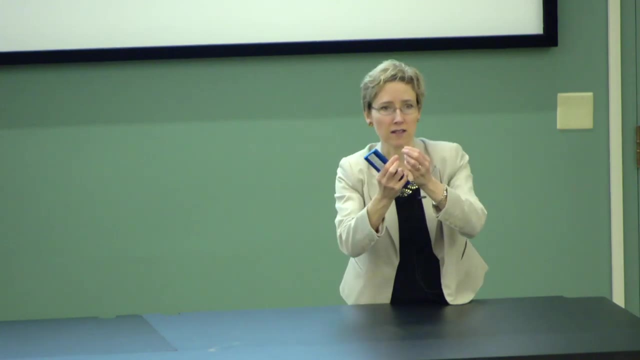 So I'm just going to cancel them, Cancel, cancel. And now my limit of delta v. so, as the volume shrinks down, what's shrinking is delta x, delta y and delta z are shrinking all at once. All I'm writing down over here: 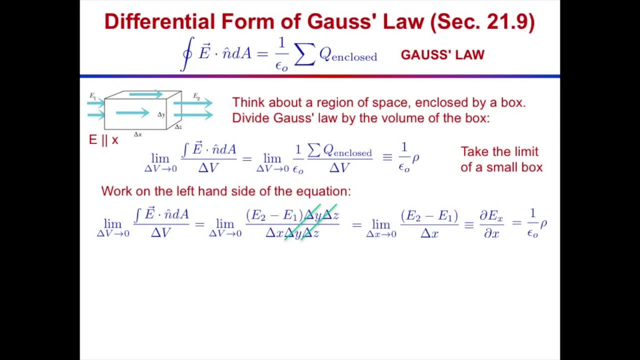 is the limit as delta x goes to zero, because I didn't have any delta y or delta z dependence left. okay, So limit as delta x goes to zero of e 2 minus e 1 over delta x. That right there. if you're a math major, you're very excited. 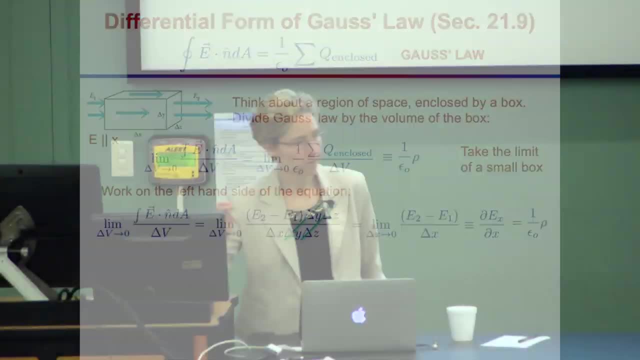 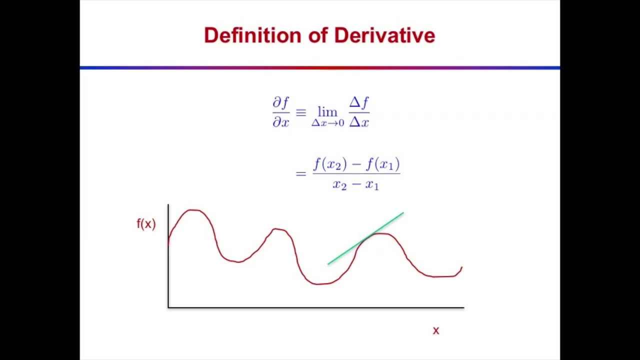 because if you're a math major, you say that's a derivative. okay, I know what that is. So let me just remind you of the definition of a derivative. alright, So the definition of a derivative df by dx is defined as the three bars mean: defined. 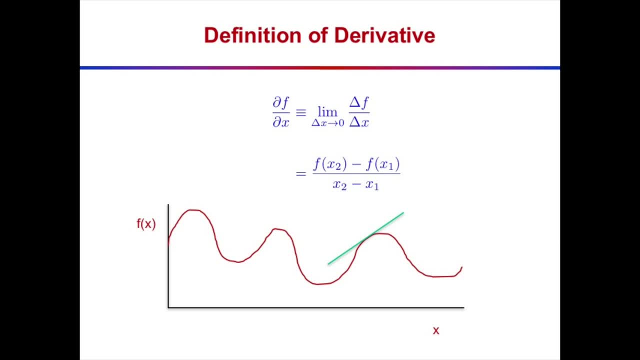 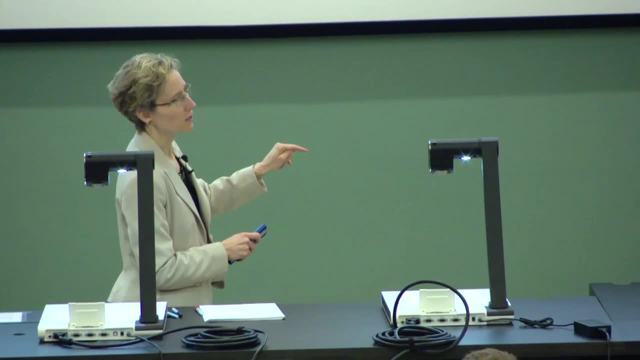 as limit as delta x goes to zero. delta f over delta x, which you could also write as the limit of f 2 minus f 1 over x 2 minus x 1, the limit as the distance between the points goes to zero. 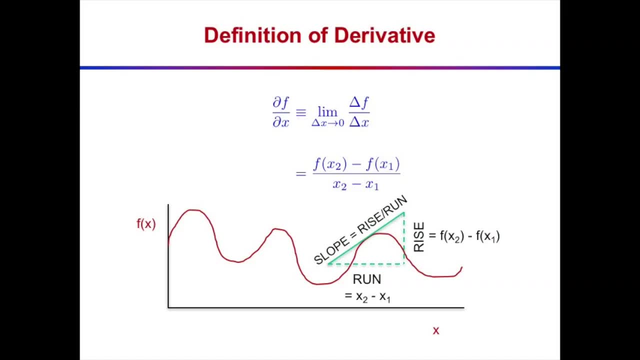 Graphically, if this is a graph of f, of x, some function versus x. so there's the squiggle, and this is point 1 and point 2, what this is telling you is: take rise, divided by run, and then take the limit. 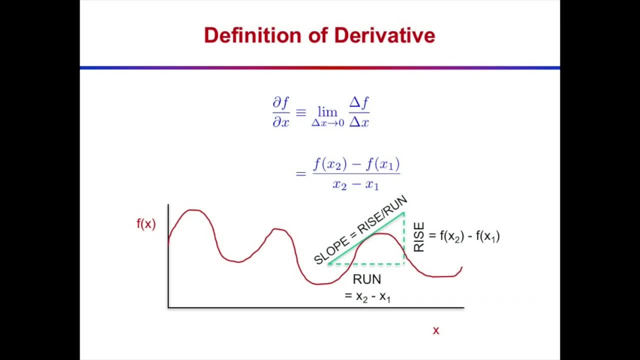 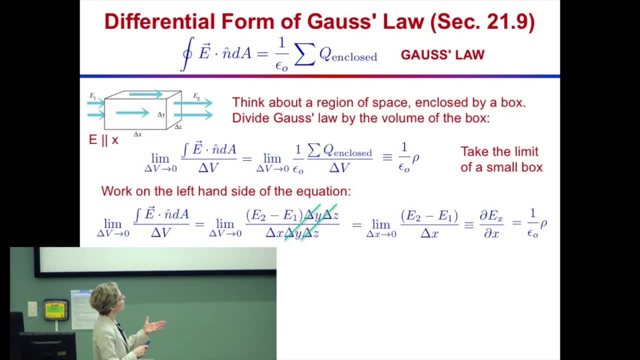 as those pieces go together, which gives you the local slope. So I hope all that's familiar from your calculus class, right? And then you can look at that calculus definition and say, oh, I have a limit, as delta x goes to zero. 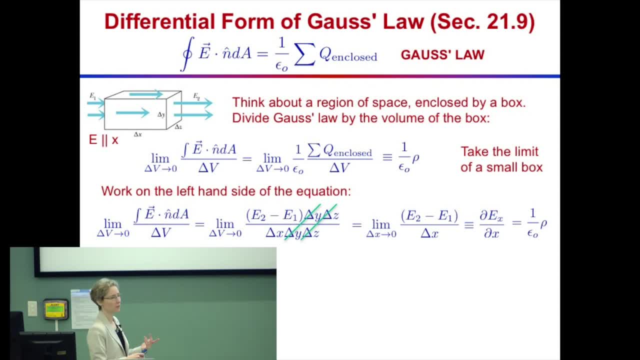 of the electric field. okay, Difference in electric field divided by delta x- and I take that limit, it gives me a derivative. So by definition then this is dx over dx. okay, So I know it's a d by dx because there's a delta x in the. 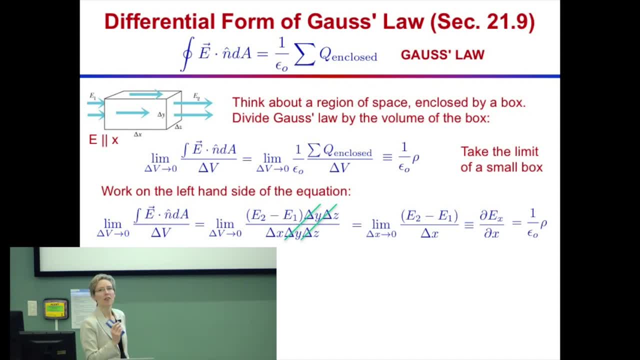 denominator. How did I know to put this as the x component? That's how I set up the problem. okay, I set up a physical situation where my electric field is parallel to x. Okay, So that's why there's an x sitting there, right? 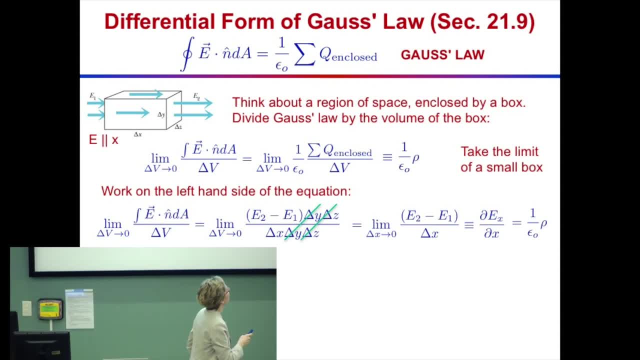 But that's how this flux is going through that box And what we've seen now so far. is that okay? this side of the equation has turned into dE by dx, and now that equals rho over epsilon naught. Do you have any questions? 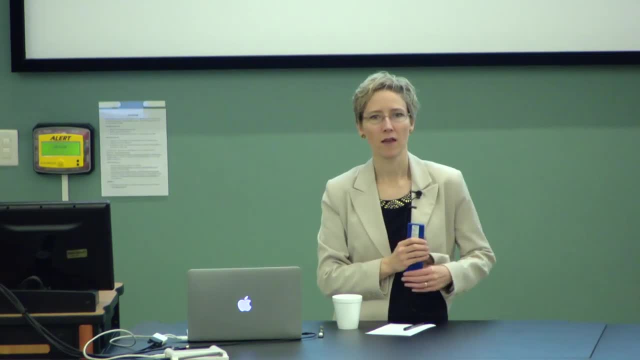 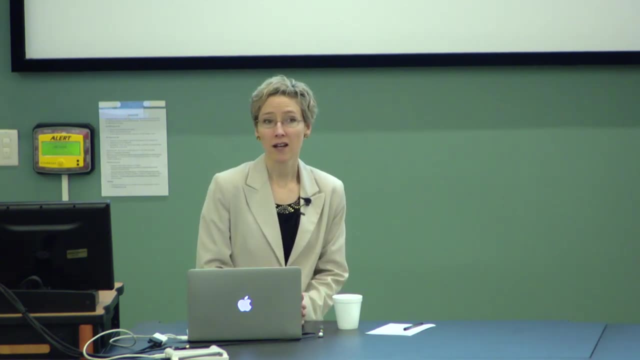 so far, Okay, Alright. Complaint Or thoughts? Okay, Alright. Now I set this up in the x direction and because I set it up in the x direction, I got a dEx by dx If I had set this up in the y direction. 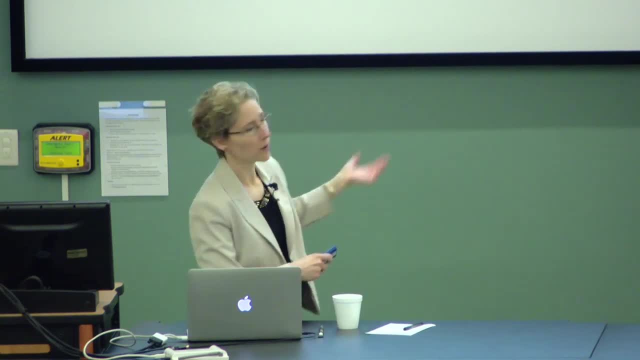 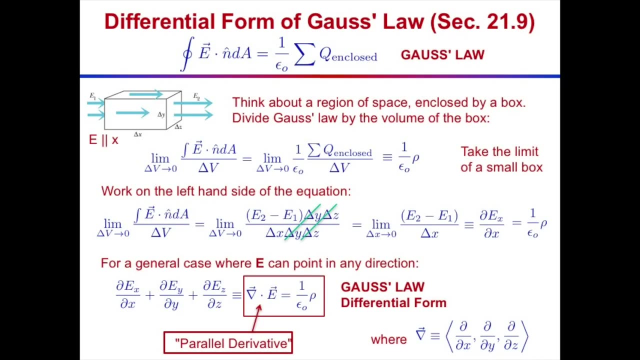 I would have had a dEy by dy If I had set it up in the z direction. I would have had a dEz by dz. So in a general case, all those guys contribute and I get dEx by dx plus. 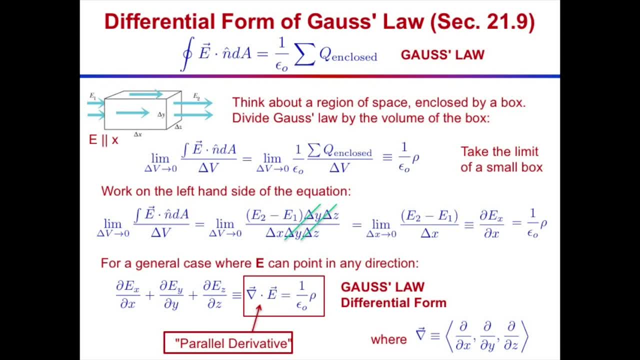 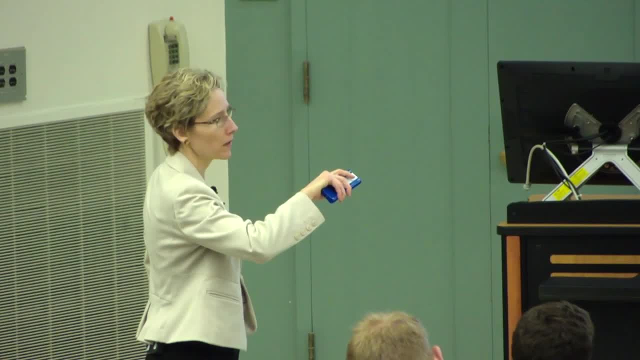 dEy by dy plus dEz by dz, is rho over epsilon naught, Okay. And then there's a nice shorthand for saying: well, when I'm taking the x derivative, I care about the piece that's parallel to x. Okay, When I take the 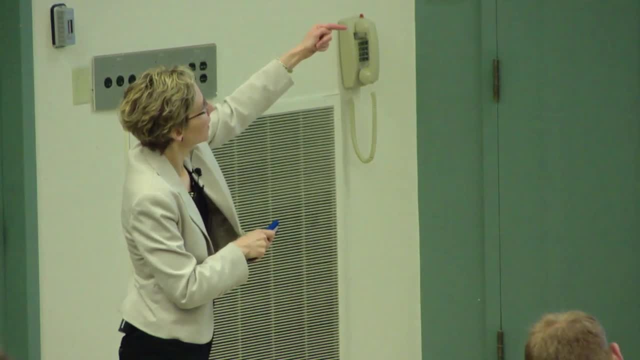 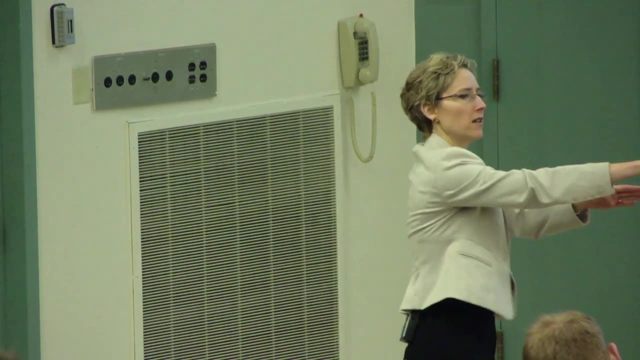 y derivative. I care about the piece that's parallel to y. That's because in going from the back of the box to the front of the box I walked along the x axis and I needed to know the flux that was parallel to x. 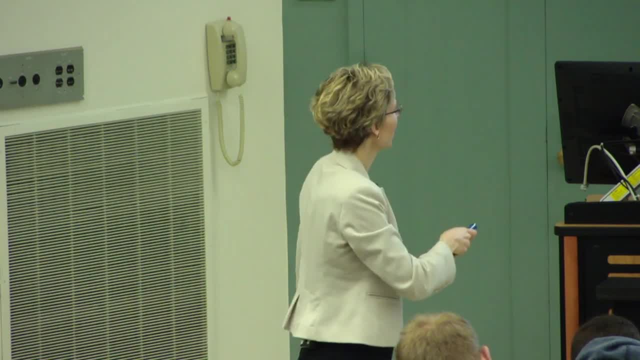 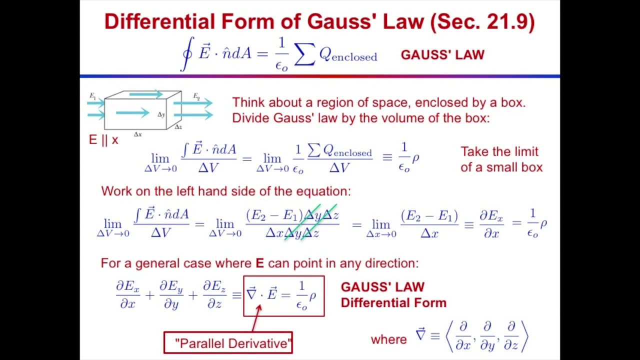 So that's why I got a derivative with respect to x there. Okay, So there's a shorthand for this, which is called del, dot e Alright, And del itself is a vector derivative: d by dx of the x components, d by dy of the y components. 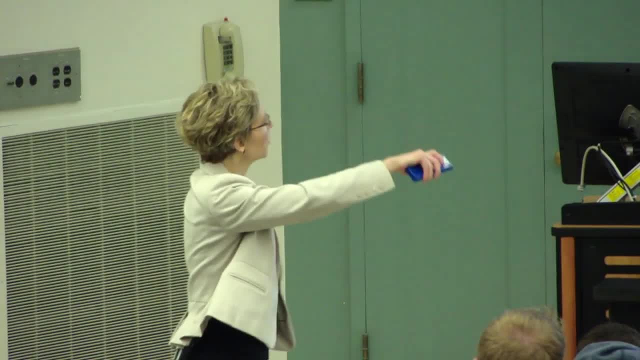 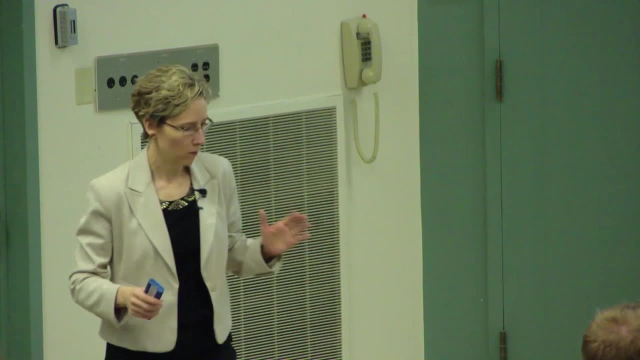 d by dz of the z components, And the shorthand is del dot e, but you can always just remember the longhand as well, Alright, So what that means is take a derivative in the following way: walk along the x direction and measure how much did. 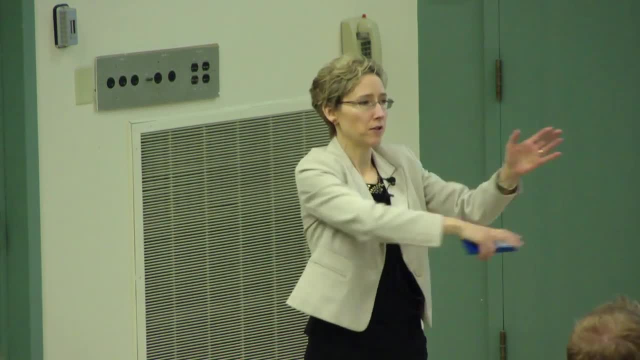 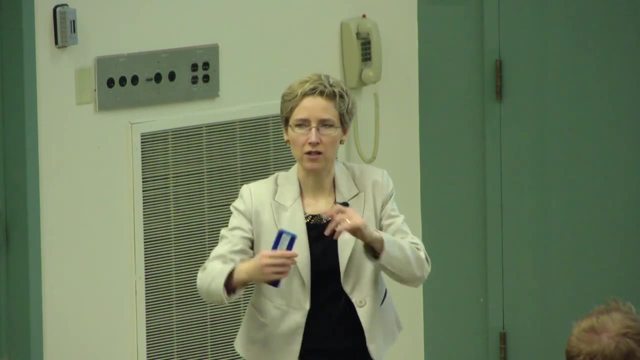 the electric field parallel to my step. how much did that change? Okay, Now take a step in the y direction and look only at the electric field parallel to my step. how much did that change? Now step up in the z direction and look only at the electric field. 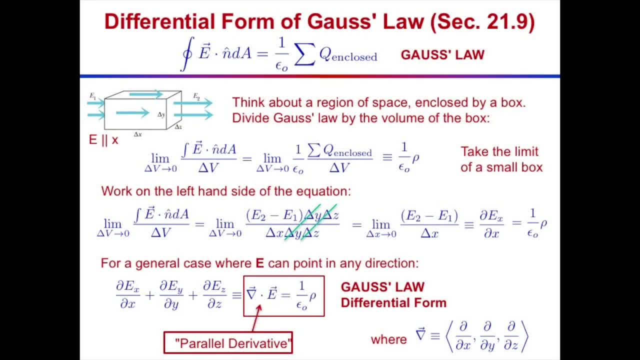 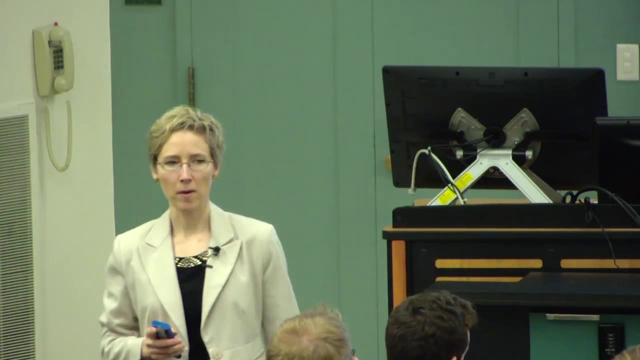 parallel to my step. how much did that change? All that together is what's called the divergence, actually, of the electric field, And that's the differential form of Gauss's law. Do you have any questions about that? Okay, How about the? 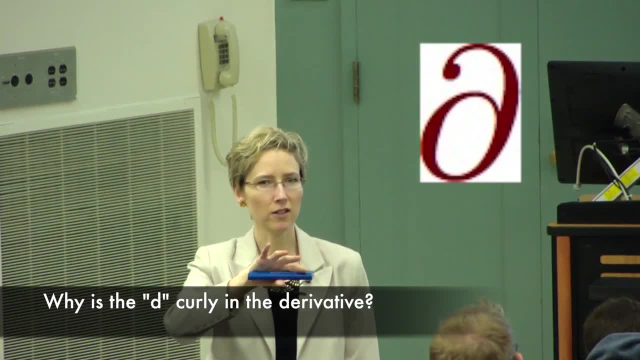 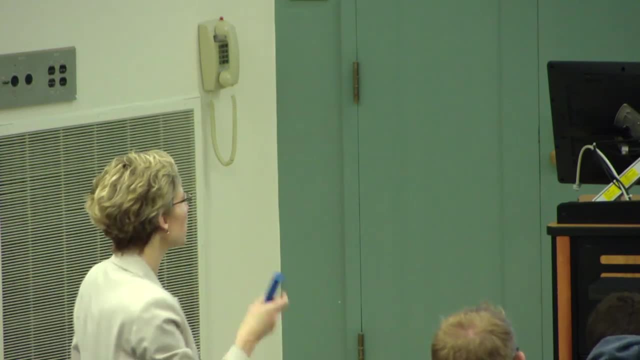 curly signs in the derivatives. Have you guys seen curly signs before? Okay, so let me, if you haven't. I see a lot of heads nodding, so some of you have. If you haven't seen the curly signs, let me just. 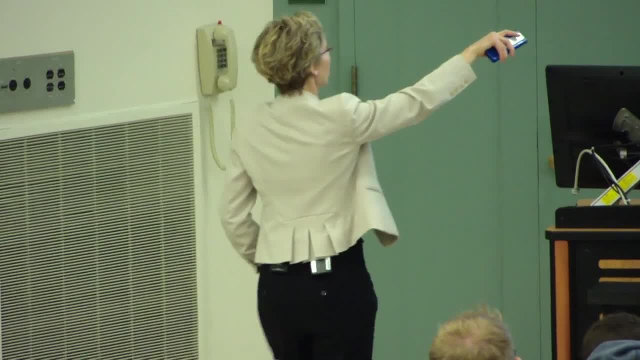 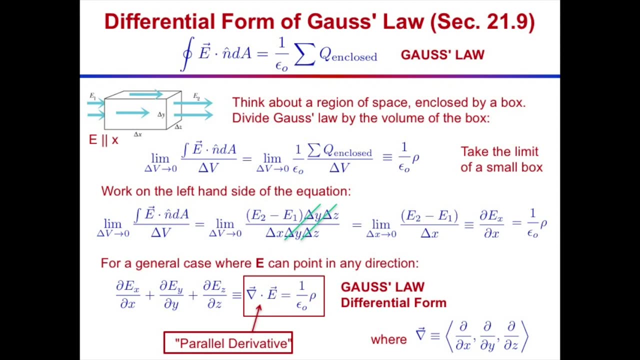 tell you what it means. It's actually not bad at all. The curly sign here, for you know, usually you see a d there, de by dx, I've got a curly d. The reason is to remind you that when you're working. 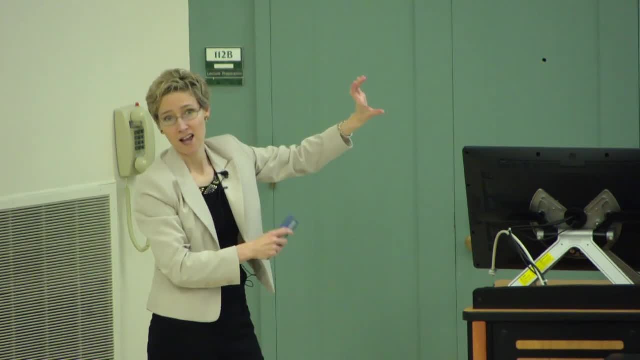 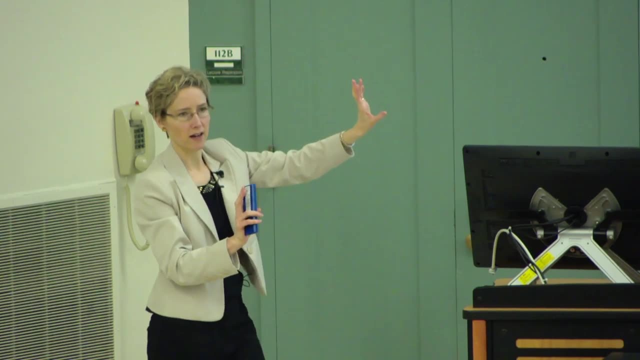 on this term, you only take the derivative with respect to x and ignore anything with respect to y or z. And when you get to this term, you only take the derivative with respect to y and ignore any z or x dependence and so forth. 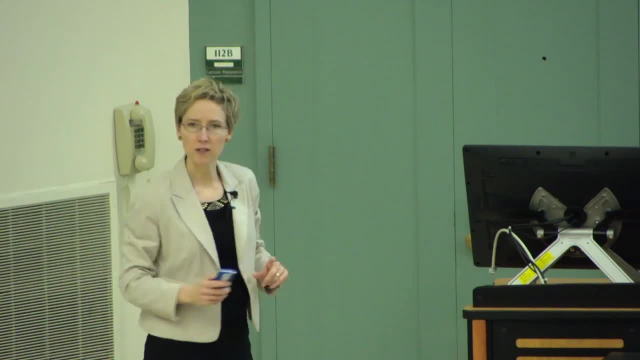 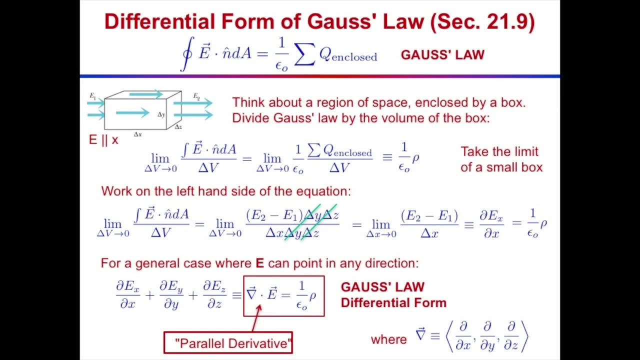 Okay, So it just means do one at a time, That's all. it means Questions, All right, And sometimes this is called a parallel derivative. Okay, So that gave us. that was a lot of math, but what we did was we converted the integral. 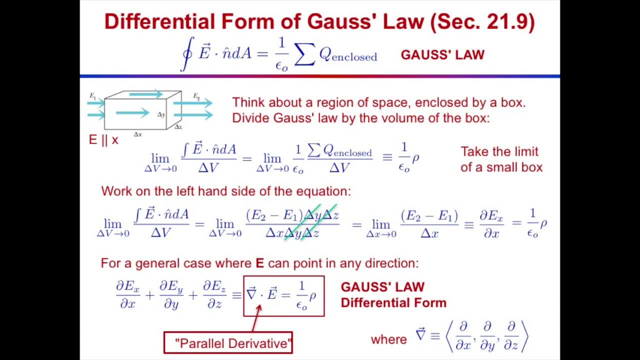 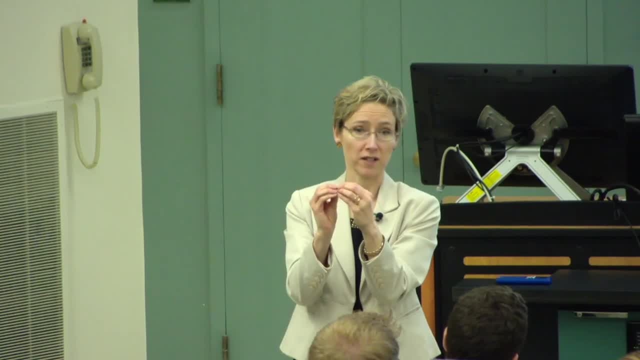 form of Gauss's law into the differential form, And in fact sometimes I said this is called a divergence because of the following idea: If I have a charge density, that's a point charge, for example, all right. and then I think of how do the electric field lines 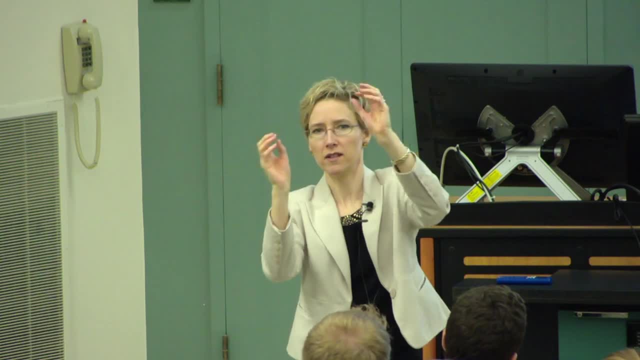 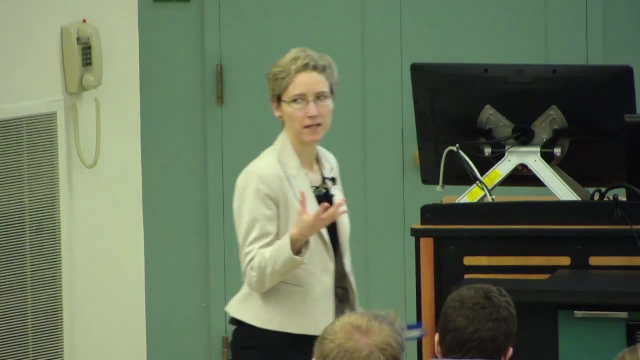 come off of that? the electric field lines come out in such a way that they diverge Right. They come out and they spread apart. That's diverging. And so this del dot e captures that piece of the electric field. that's diverging. 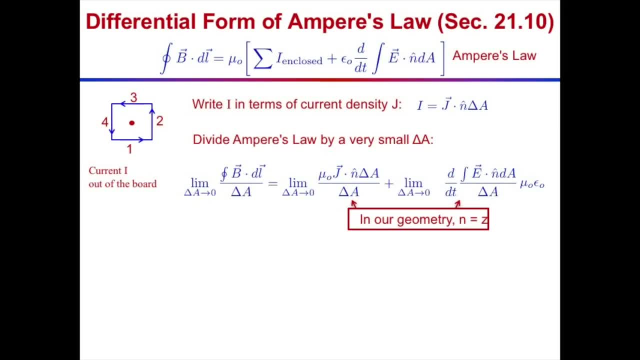 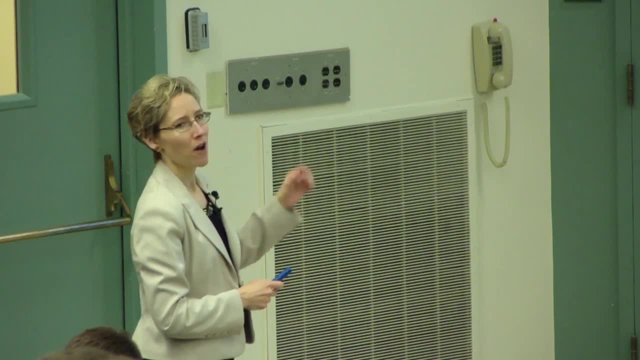 All right, The differential form of Ampere's law. So here's Ampere's law, All right. Integral line. integral of B dot dl around a closed loop is equal to the sum of the currents that are piercing the area inside the closed loop plus. 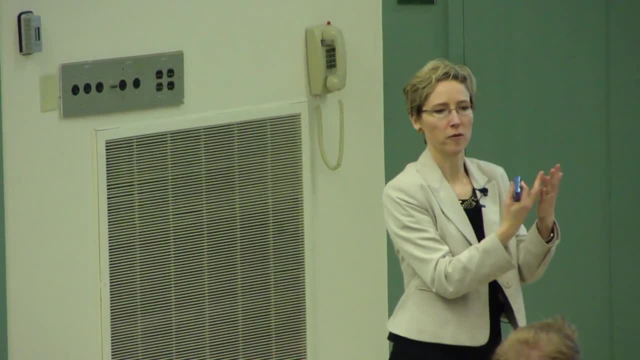 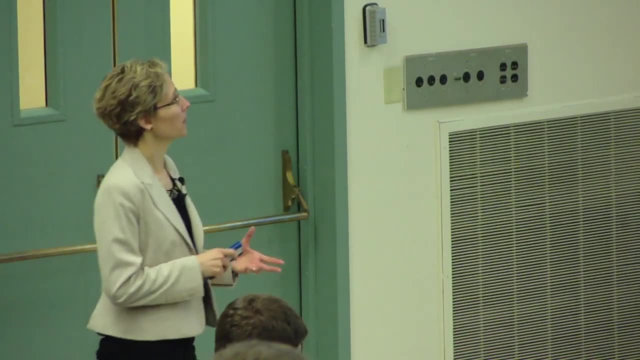 any time. derivatives of the electric flux through that soap film that attaches to the closed loop. That's Ampere's law. So now again, half of physics is writing diagrams carefully. I'm going to carefully set up a diagram here to where I can take. 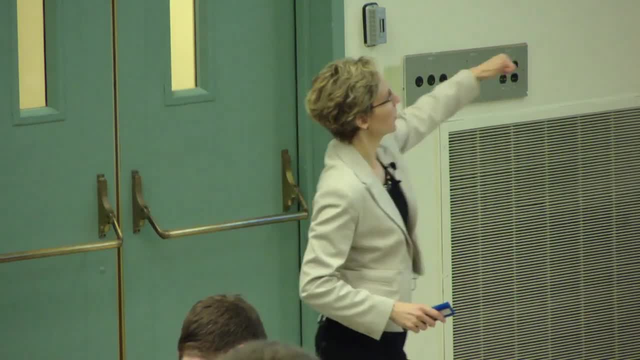 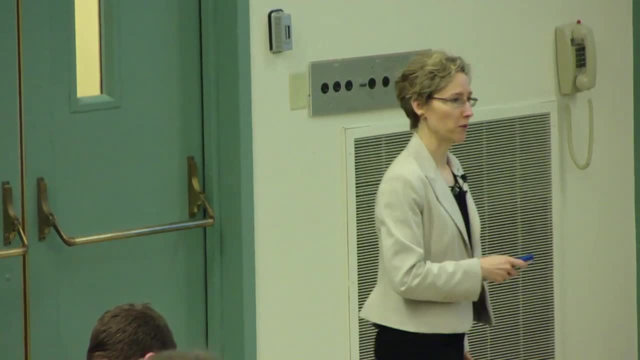 a calculus limit and get the differential form. So here I have current, i coming out of the board towards u And I'm going to let integral B dot dl be this nice square. I'm going to take a nice square path so I can easily take the calculus. 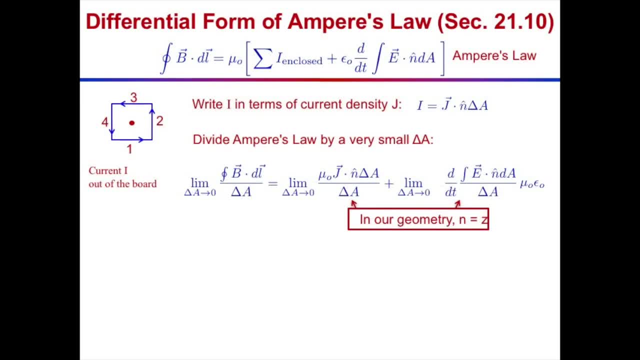 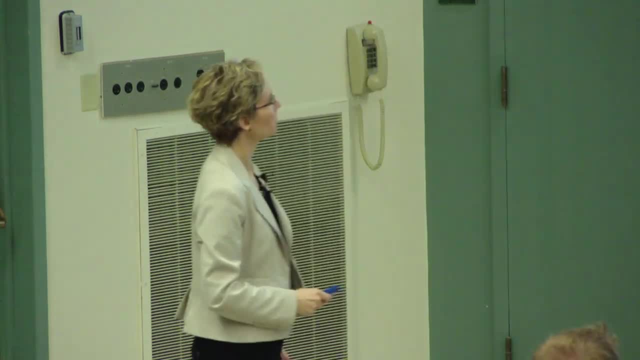 limit. So I'll go along step one, step two, step three, step four. X axis is horizontal, Y axis is vertical And z is out of the board towards u. So now think of applying Ampere's law to this case. 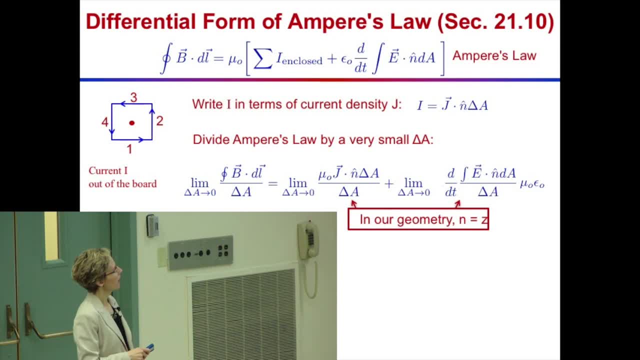 Okay, Integral B dot dl will be around that path. I have an i enclosed, All right, There could also be electric flux, so we'll keep that term as well, And what I want to do is divide all of Ampere's law by that tiny area associated. 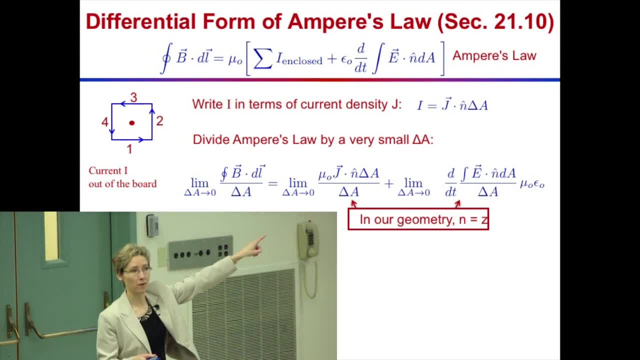 with that square that I wrote down. So delta A represents that area of the square. So I'll have limit as delta A goes to zero of integral B, dot l over delta A. Okay, And then again I'm just going to then take the limit as that area. 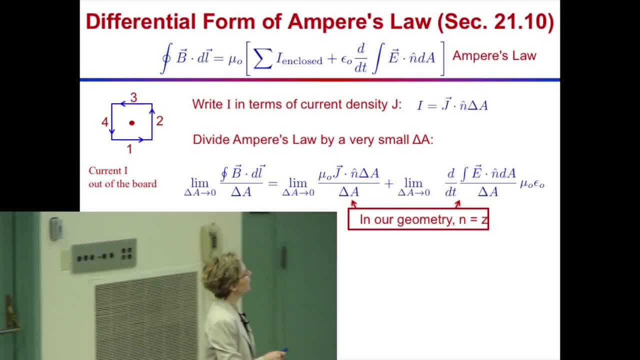 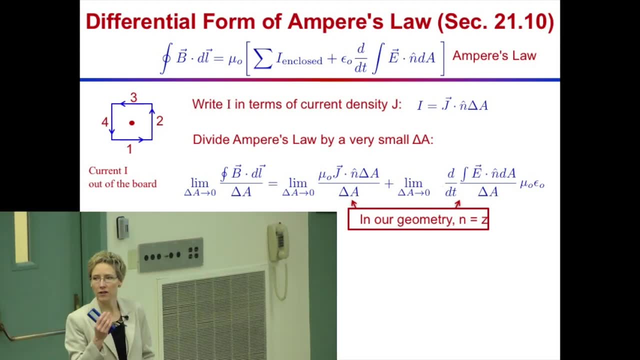 goes small. That's what calculus always does. So on the right hand side here I have current. Okay, I'm going to rewrite current as current density. Okay, Current density is current per unit area, And so if I take current density, which is current per unit area, 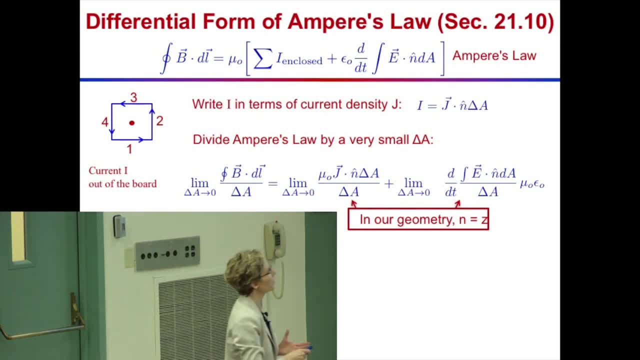 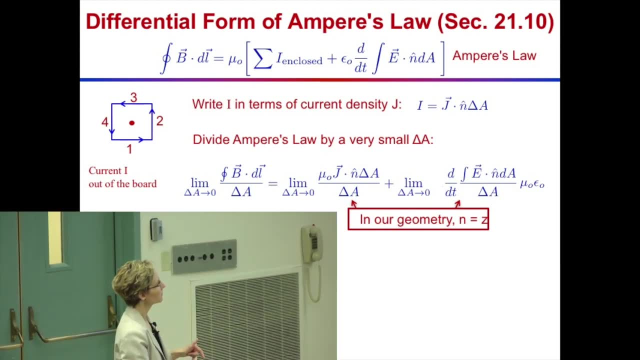 and then multiply it by area, I get back current. So current is current density times area. All right, So that's sitting right here. Divide all of that by delta A the area. Okay, And then the third term was d, by dt, integral, e, dot, nda, And again. 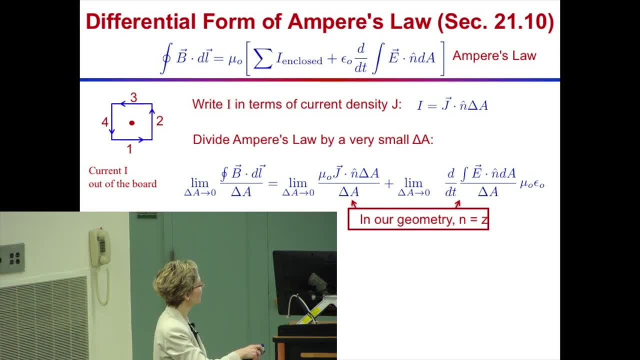 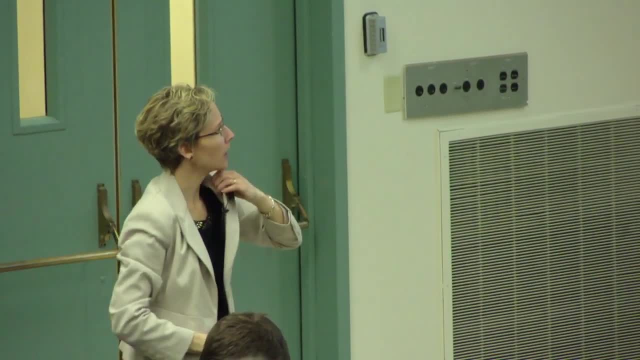 I'm just going to divide that by delta A, Then I'm going to take over the whole thing. So I took the whole equation divided by delta A. Now I'm going to take the limit that delta A gets small And I'll do the same thing I did before. 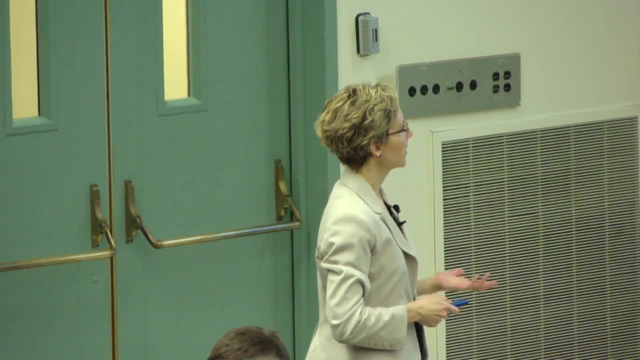 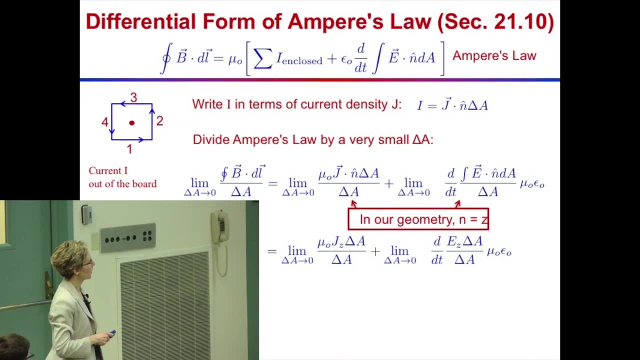 Re-express delta A in terms of things that are in the diagram. So let me do a little bit more simplification here. first, This j dot n. all right, I'm going to now say in my geometry that what I care about is the flux coming. 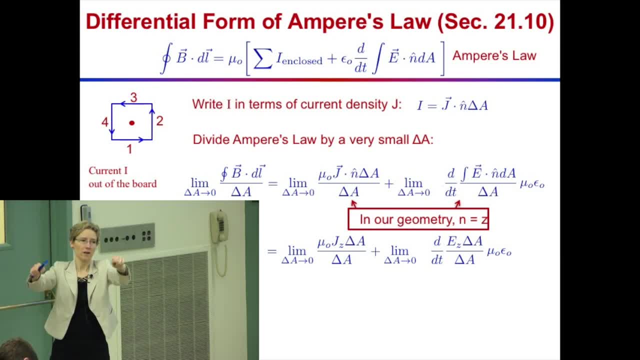 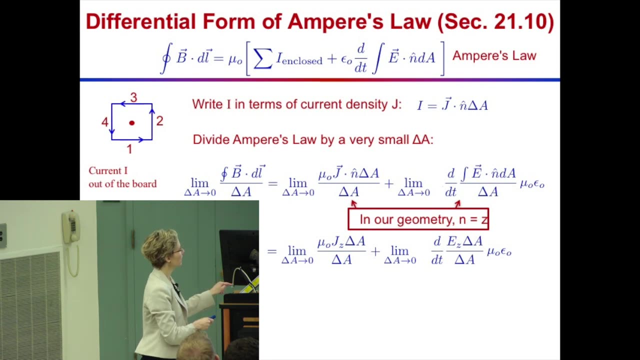 through the board Right. So I've defined an area, All right, And our area it's n. the normal to that area is along the z axis. So now, if I identify n as z hat, I need to take j dot n, which becomes jz. 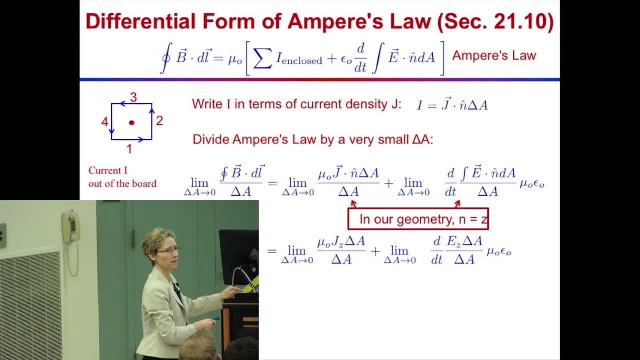 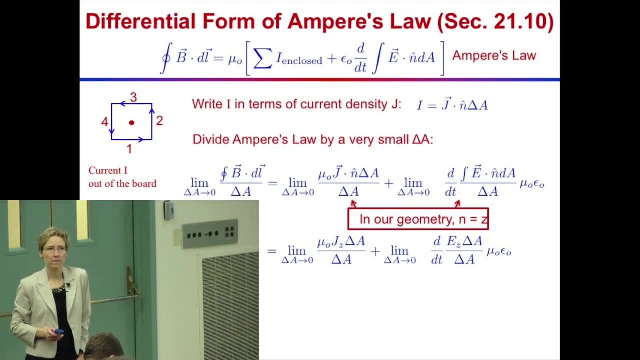 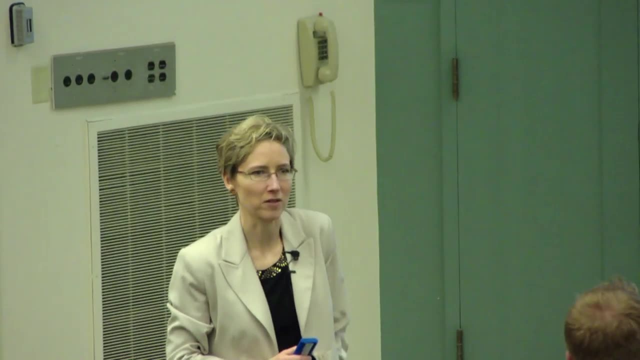 and I need to take e dot n, which becomes ez, So it's the z component of the electric field comes down. Any questions? so far? All right, Okay. Does no questions mean we're doing okay or I need to talk about something more? 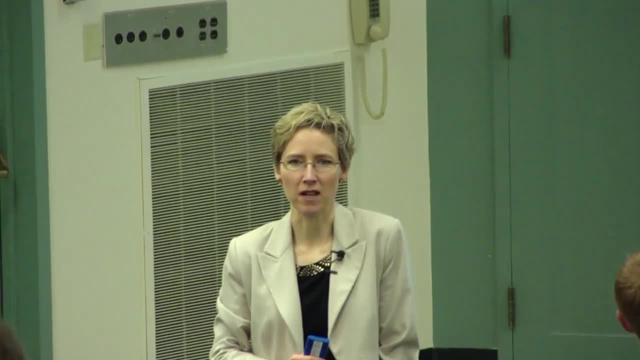 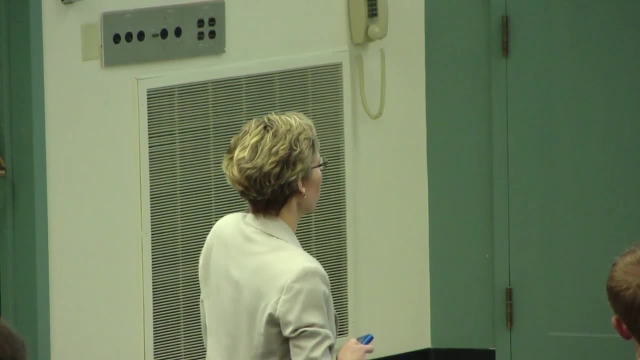 Just give me a little thumbs up or a thumbs down if you want me to. Thumbs up means keep going, Thumbs down means I've got a question. Okay, We good. All right, I've seen a lot of thumbs up, All right. So 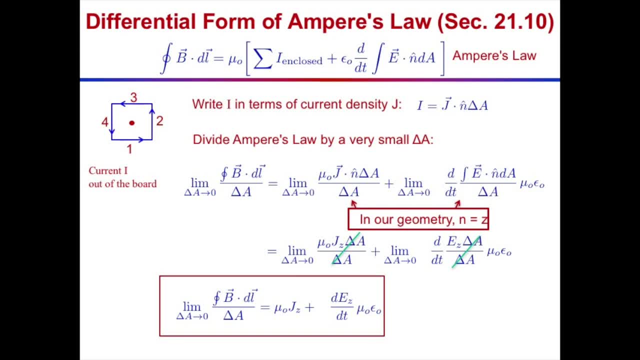 cancel the a's. All right, Cancel the a's. Cancel the a's there And take the limit as delta a goes to zero. So now the right hand side became mu, not jz. There it is, And the right hand side over here. 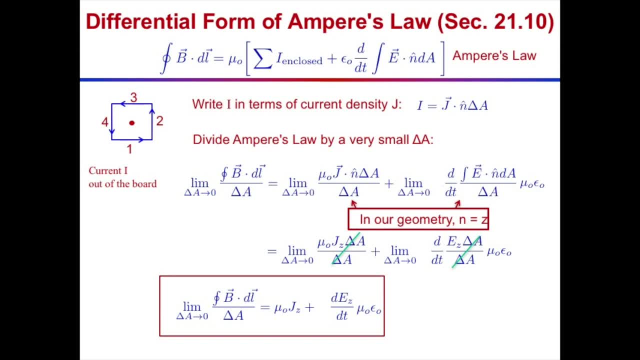 all the a's fell out, So the limit as delta a goes to zero was easy. in this case Again, I'm just shrinking that loop down And I get dez by dt times, mu, not epsilon not. So it's this left hand side we're going to have to. 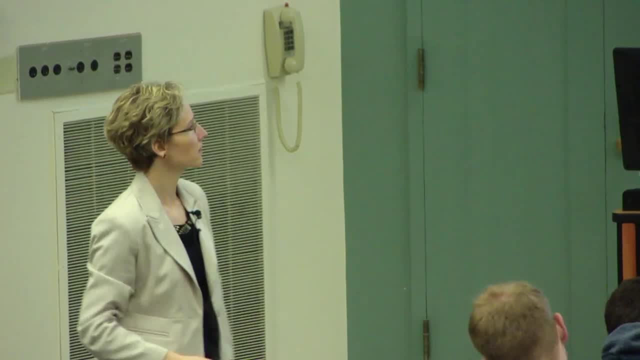 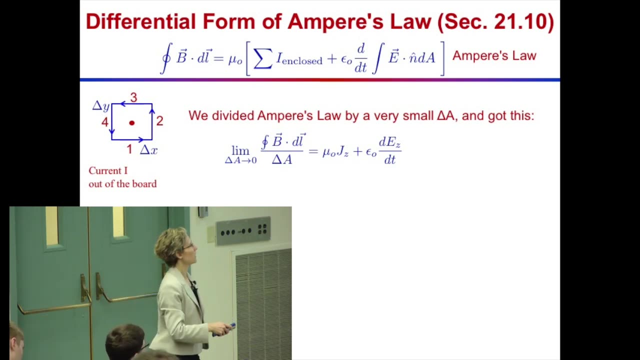 work on. Okay, So this equation I'm going to copy on the next slide. There it is Straight down, And the thing we need to work on now is the left hand side. So work on the left hand side. You see, that's a bunch of 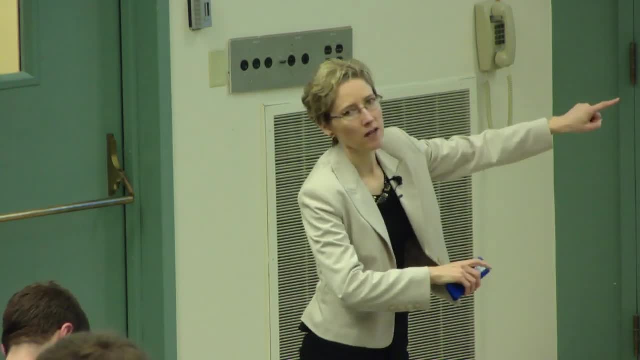 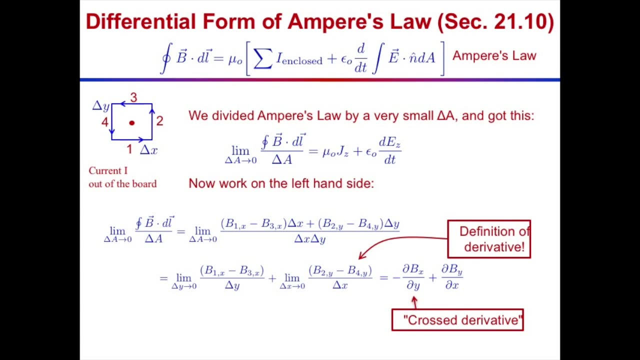 math. But before we get to the bunch of math, what's going to come out is derivatives. All right, So that's the purpose of what we're doing. We've divided by a delta a. We're going to take the limit. as delta a goes to zero, We'll 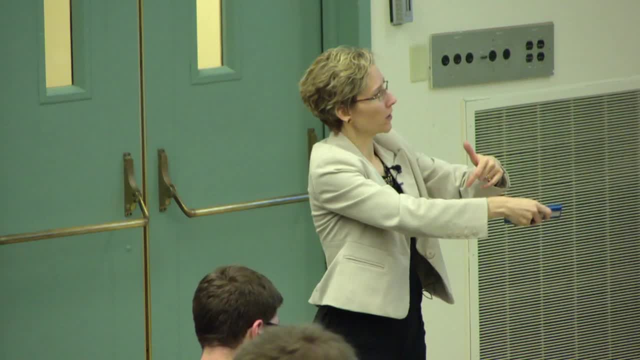 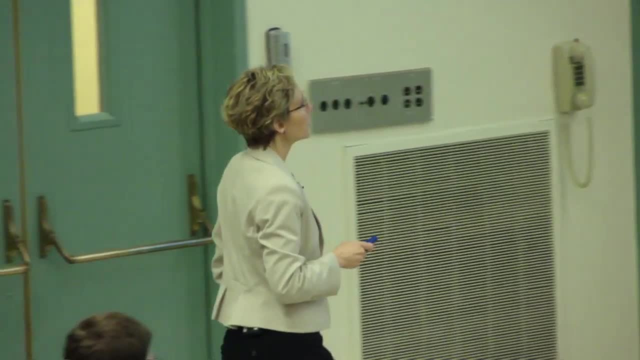 find the derivatives based on the definition of a derivative over here, And then that'll tell us that these are the derivatives. Okay, So let's work on this. We'll massage this guy a little bit. So I have a limit as delta a goes. 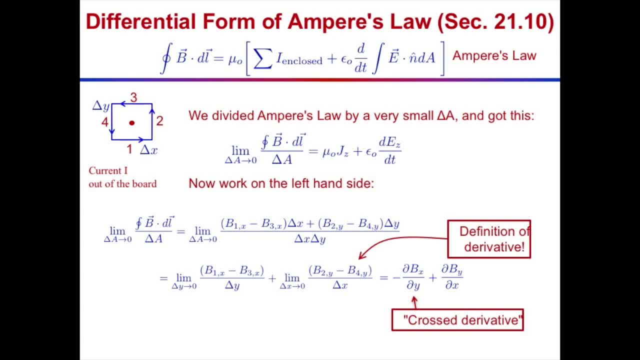 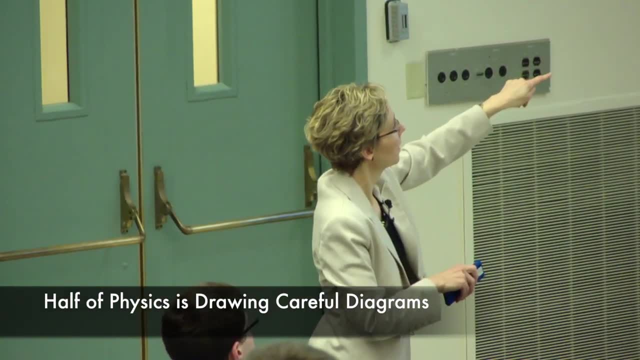 to zero of line integral b dot dl over delta a. So now I need to just look up my carefully drawn diagram. Half of physics is carefully drawing your diagram. So I have segment one, two, three and four. And so now what does integral b dot dl? 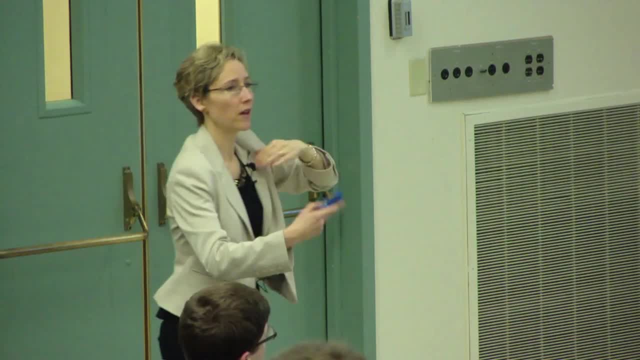 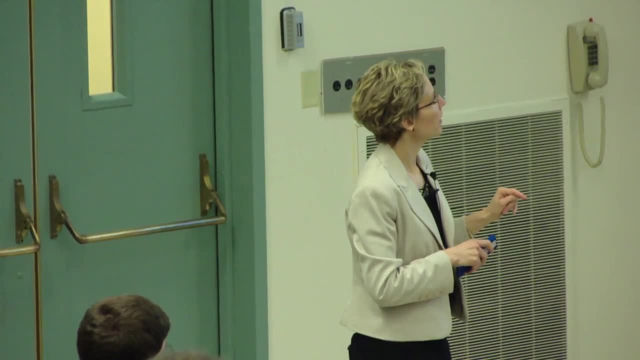 mean, It means walk around that loop. So I walk around that loop and I take b dot dl at every step. So one of the steps is along segment one. So, along segment one, I'm going to take a step in the dx direction. 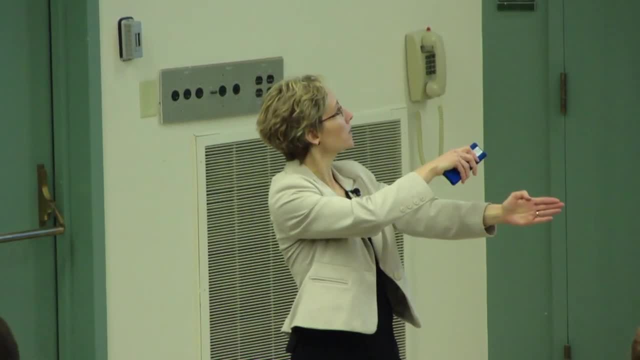 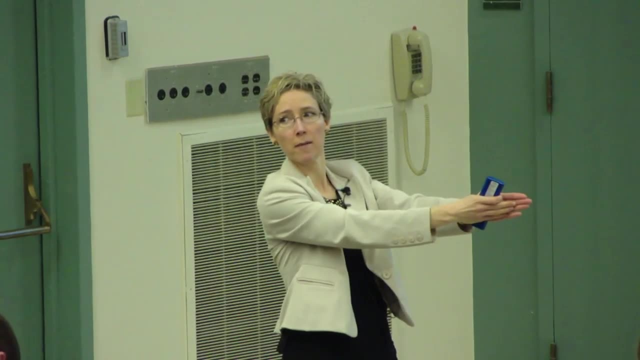 And I'll take the magnetic field that's parallel to me. So I'm at position one, So I call that b1.. And I'm taking the component of magnetic field that's parallel to my step, which means I need the x component. 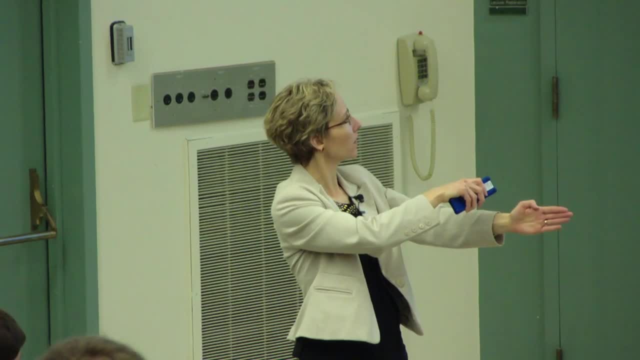 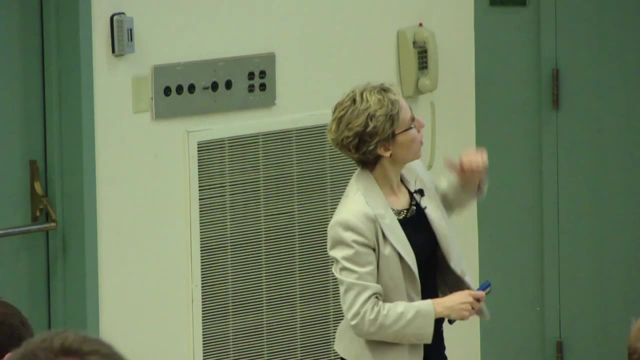 So that's b1 comma. x Just means x component, And then times delta x. There's the delta x. That was the first leg. The next leg is we're going to walk up. So now walk up in the y direction, And so I take a delta. 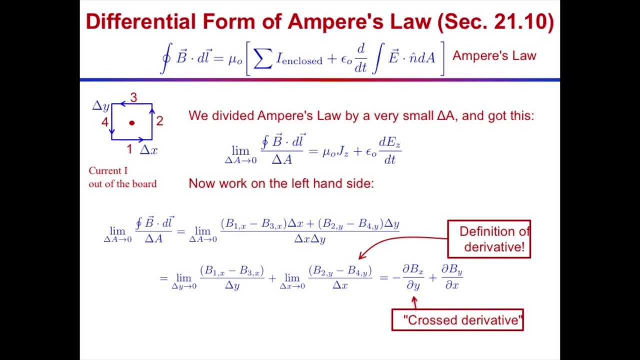 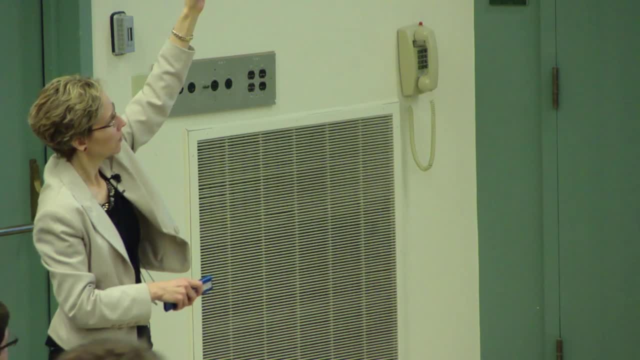 y step up, There's the delta y Times the magnetic field at that spot, which is b2.. Just according to how I drew the diagram And I need the y component of that. So that's here: b2y times delta y. 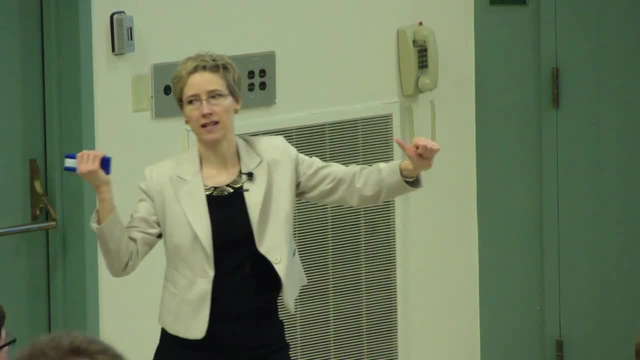 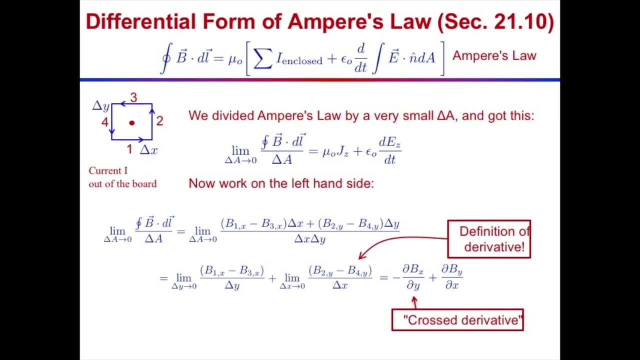 Now the third leg is up top. Now I'm going to walk backwards along the x axis. So I'm taking a step now in the minus delta x direction. So there's a minus delta x right there. for that. Which piece am I picking up? I'm picking. 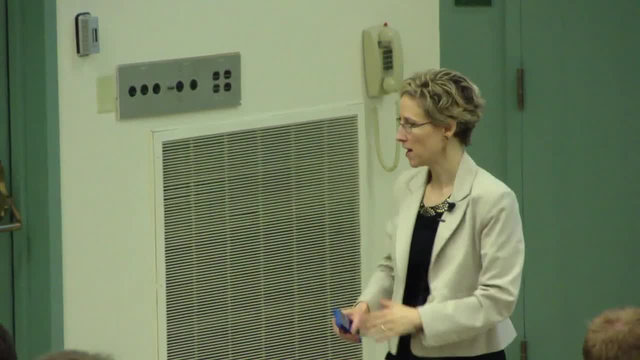 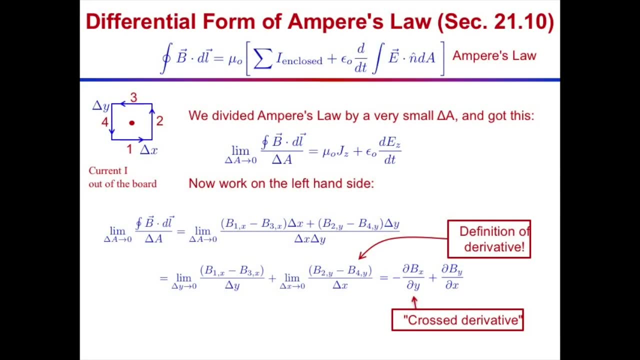 up b3.. That's just magnetic field. at position three, I'm going to take a minus delta x step. I need the component that's parallel to the x direction, which is b3x. So there it is: b3x. There's a minus sign. 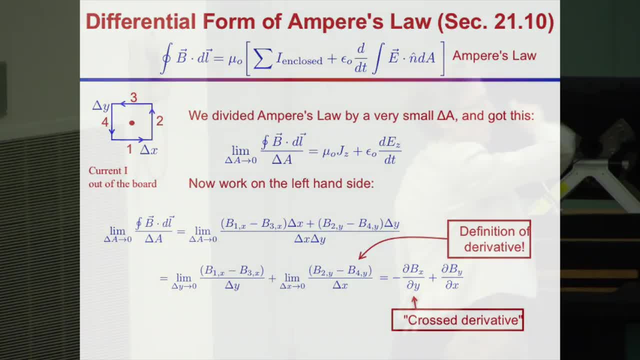 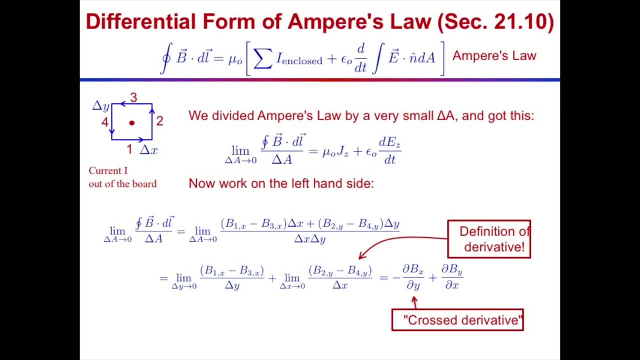 because I walked backwards. Now I walk here. Now I'm going to walk down along the y axis. As I walk down along the y axis I get a minus delta. y contribution Times the magnetic field at position four in the y direction. 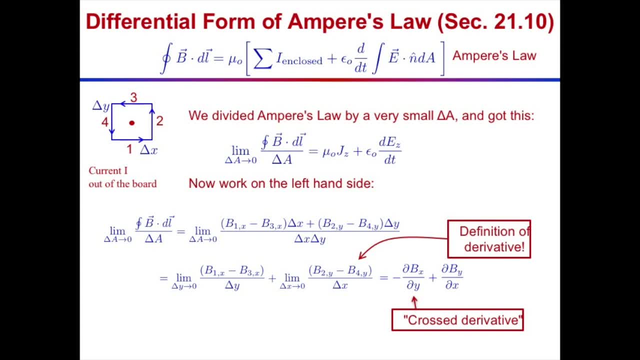 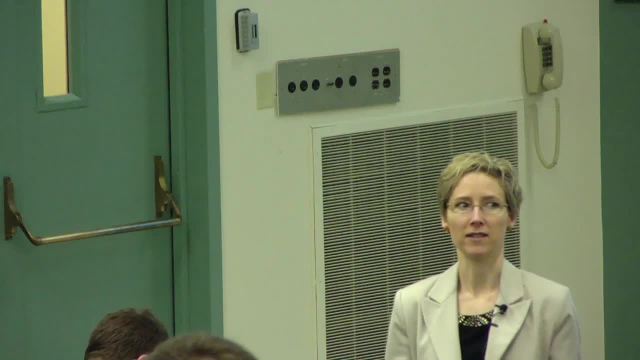 So that's all that numerator right there. Delta a: I'm going to re-express in terms of delta y and delta x. What's the area of my square in terms of delta x and delta y? You can just read it off the diagram, right? 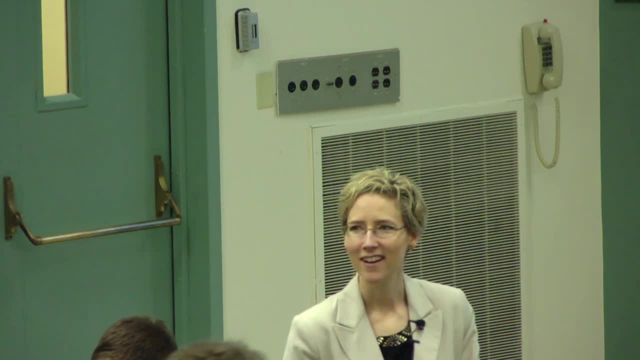 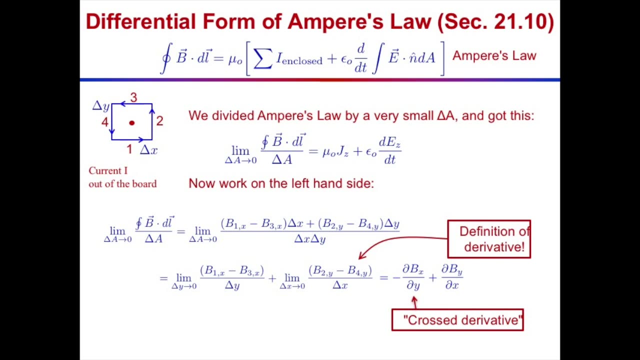 So what's the area of my square? Yeah, I'm hearing some whispers here of delta x, delta y. That's just how I set it up. So this area becomes delta x, delta y, And now you can see in this first term here. 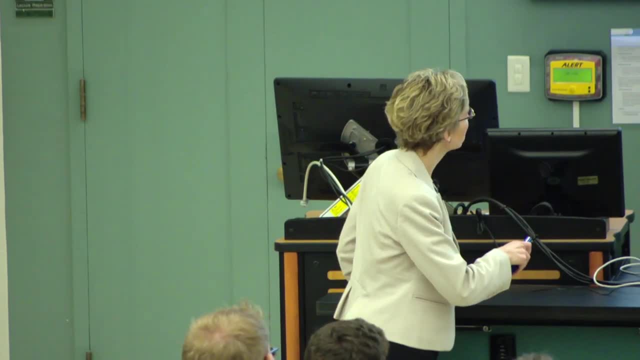 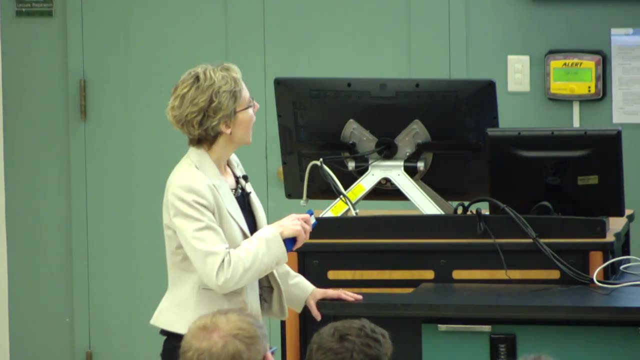 delta x will cancel delta x. So now I just have a delta y and this first term is here. The second term is going to land there. So the first term here, delta x cancelled, and for the limit, as delta a goes to zero. 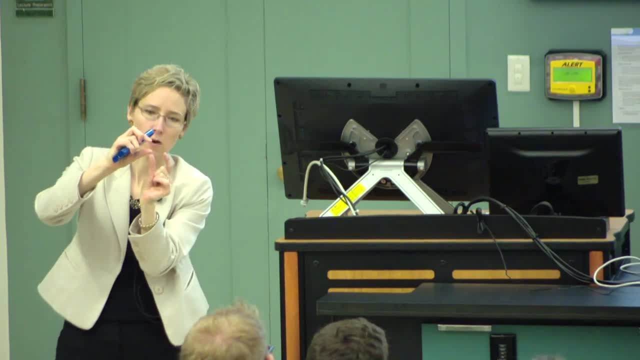 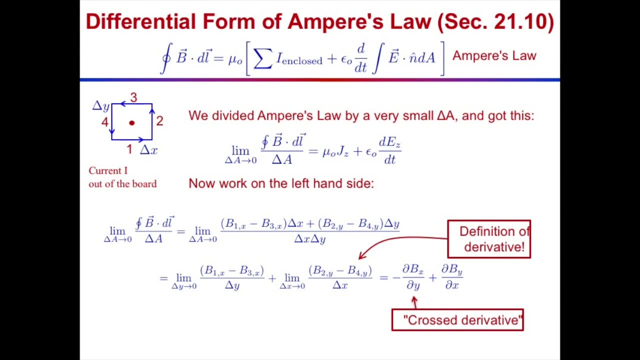 what that really means is shrink delta x to zero while I shrink delta y to zero. Okay, And in this term I don't have a delta x left, so I already took the limit, And what's left is this: delta y Right, And then over here. 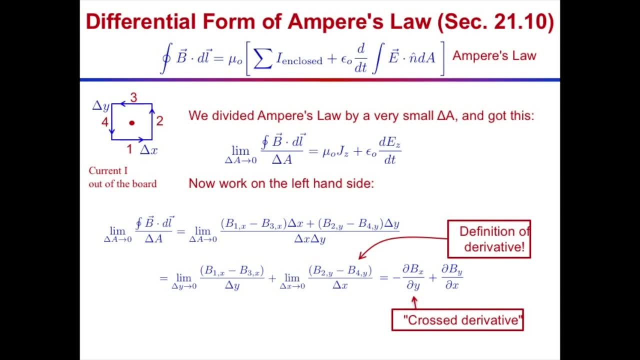 I have b2y minus b4y. The two and the four just represent where we are in the diagram And the delta y is cancelled. so I have an over delta x and I have the limit as delta x goes to zero. Alright, So this guy right here. 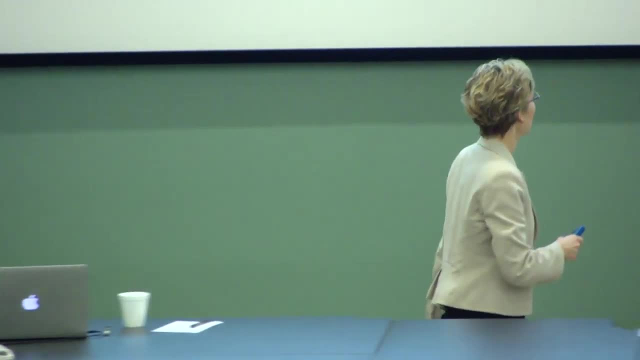 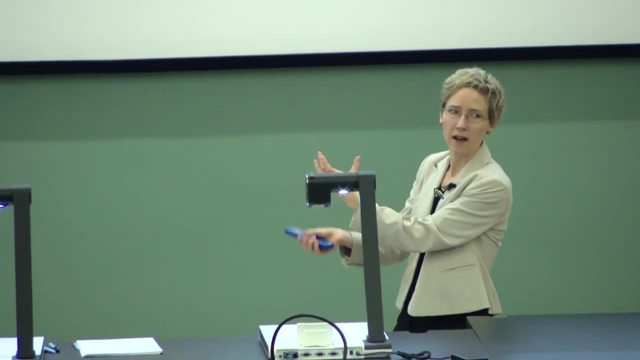 I can spot as the definition of a derivative. Same thing here. Alright, So in looking here I have again a function difference in a function divided by the space distance that I walked and the limit is that space distance goes to zero, That's. 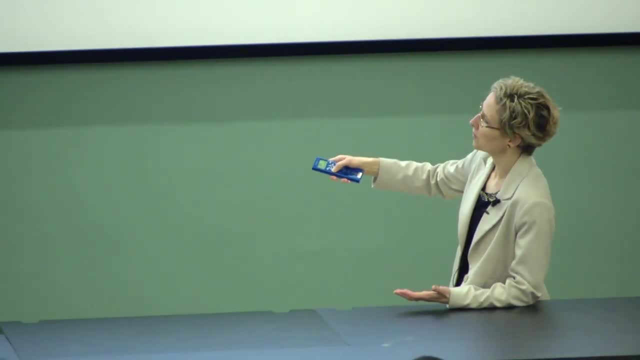 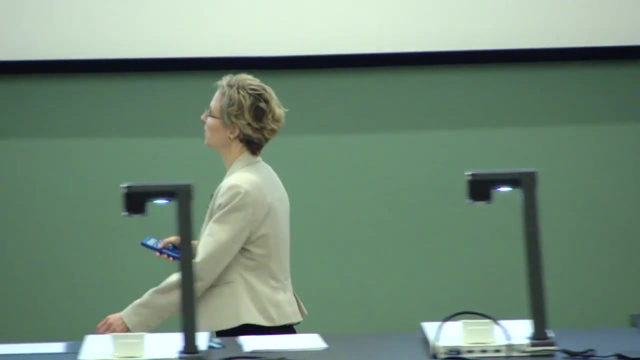 this again: It's rise over run, Okay. It's rise over run of the magnetic field in the x direction, Okay, And in fact it's about how the y component is changing. So this piece right here becomes d by, dx, of by, because notice. 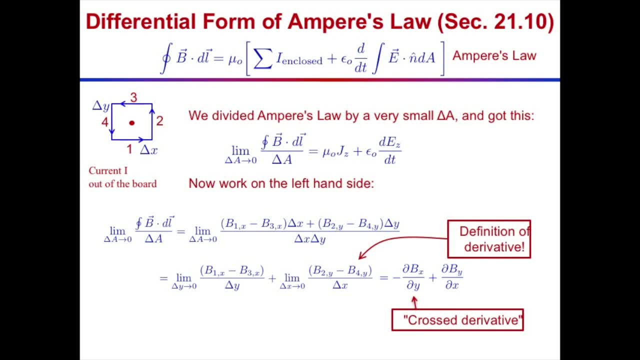 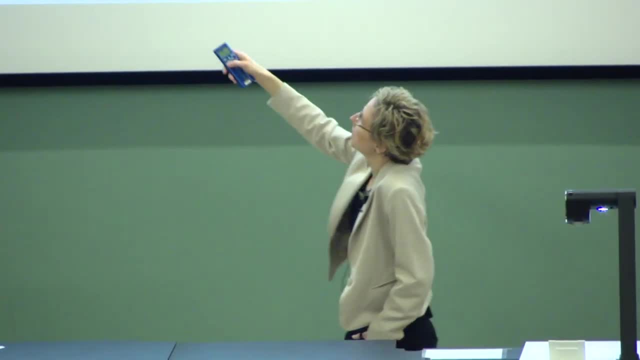 the y was there, so just carry the y over. This piece right here becomes d by dy of bx, So bx is right here, d by dy. Alright, Now, because of how I set things up, this guy has a minus sign in front. 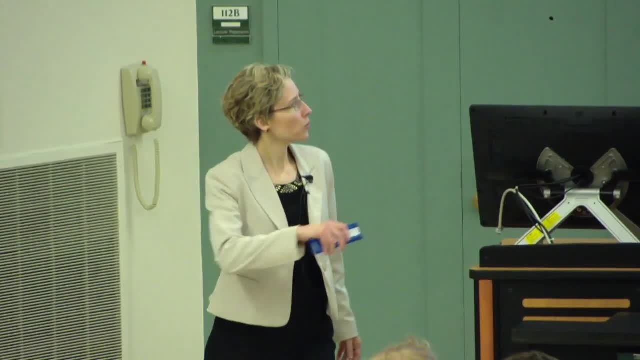 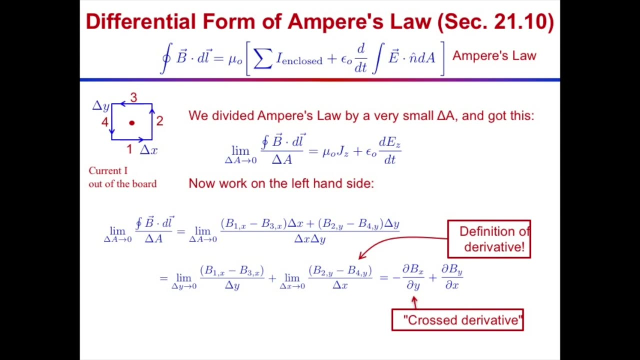 That's actually physical. And so what does this mean? Okay, This is called a crossed derivative, because I'm taking a d by dx of the y component and I'm taking a d by dy of the x component. So let me just tell you what it means. 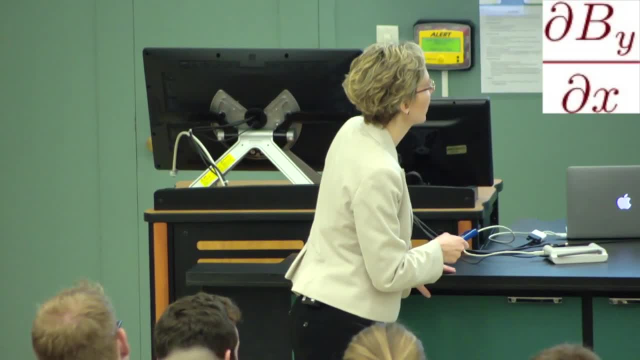 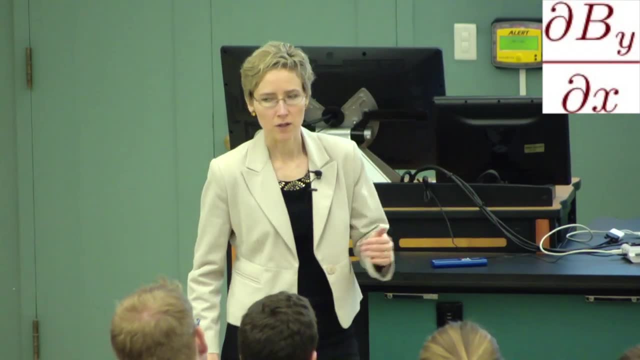 physically. okay, This guy right here. okay, This x component says d by dx. d by dx means as I walk along the x direction. okay, So as I walk along the x direction. I'm taking a derivative of by. By is pointing in the y axis, right? 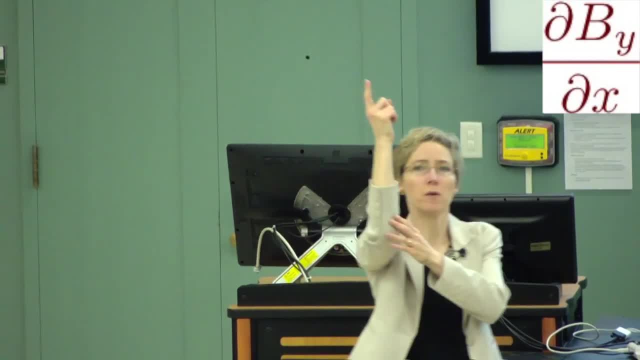 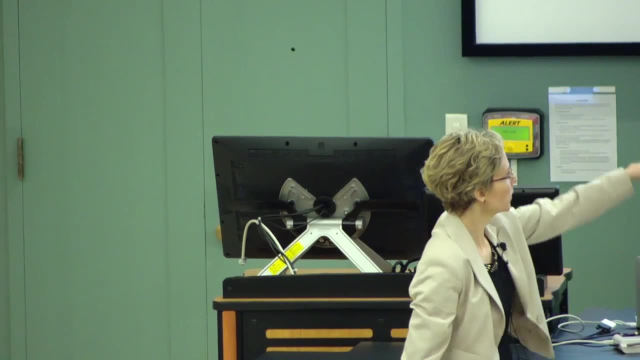 So if by is here at this spot, and then if by changes to this at this spot, I just got a derivative in by Right, It's a change in by. That's what that term's about. So this is called a crossed derivative. alright, And 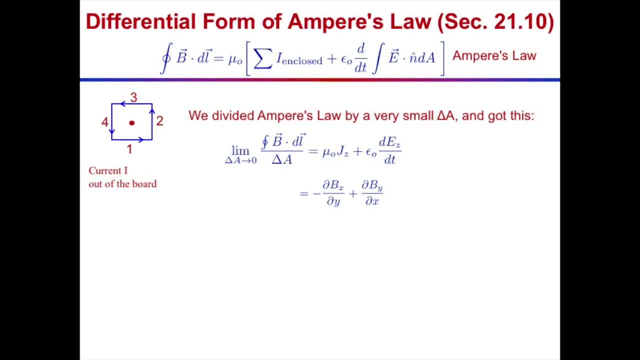 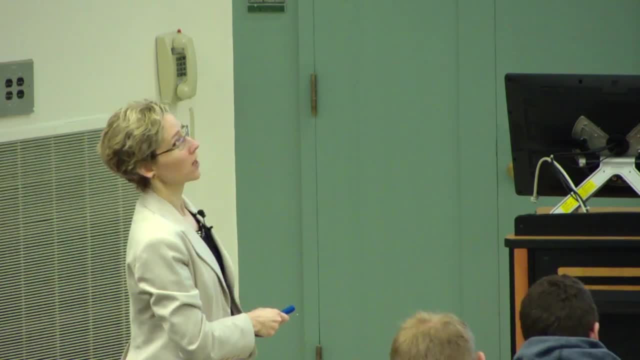 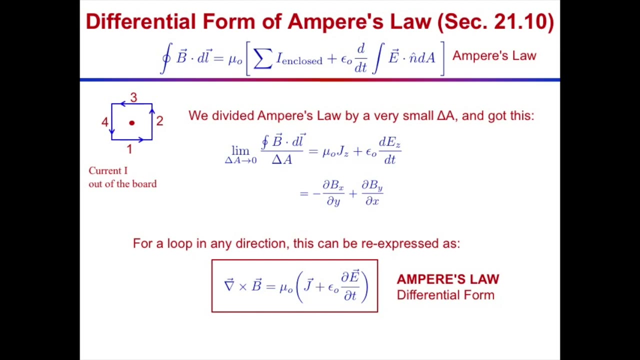 in fact in this case here it's about z components. Alright, So this can be re-expressed as del cross b. It's a crossed derivative right. It says: when I walk along x, I want to know how by is changing And when I. 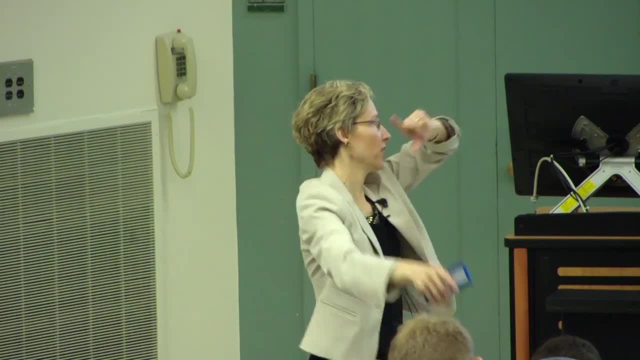 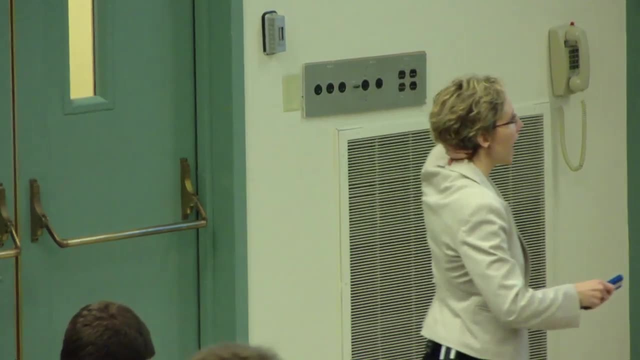 walk along y. I want to know how x is changing. Okay, So it's a crossed derivative, Turns out. you can summarize it as del cross b. I'll show you what all that means on the next slide. And so, for a general case, 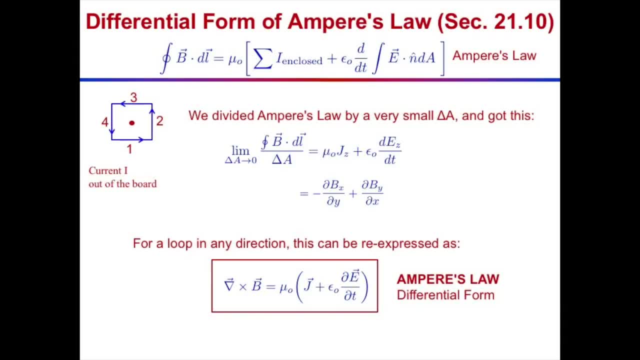 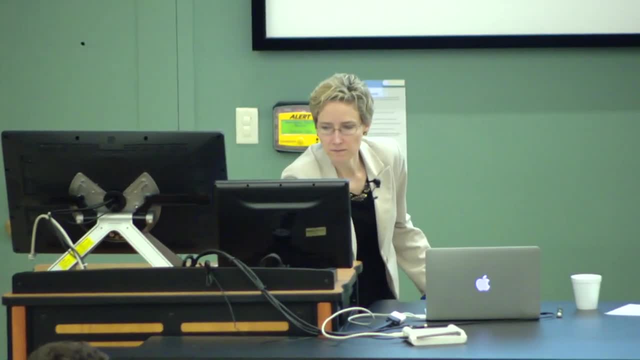 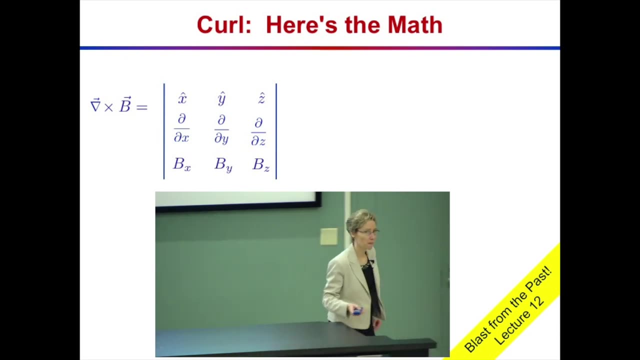 then this is del cross. b is mu-naught times j plus epsilon-naught dE by dt. So let me show you on the next slide what del cross b looks like. Okay, So you've seen this math before for a curl, This is del cross b. 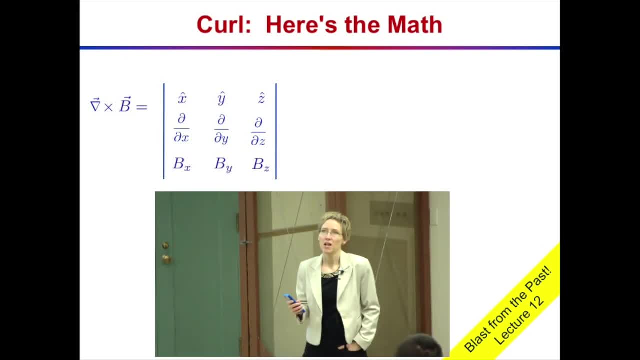 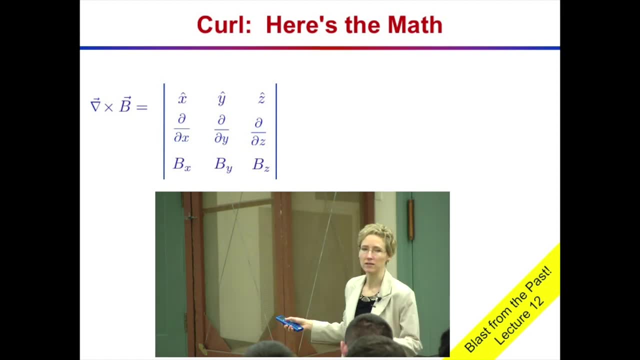 Alright, So del cross b. so for um. you've seen it before as crossing two vectors, right? You saw it as a cross b before. Now I've got this thing called a del, right, As we said before, what is del? 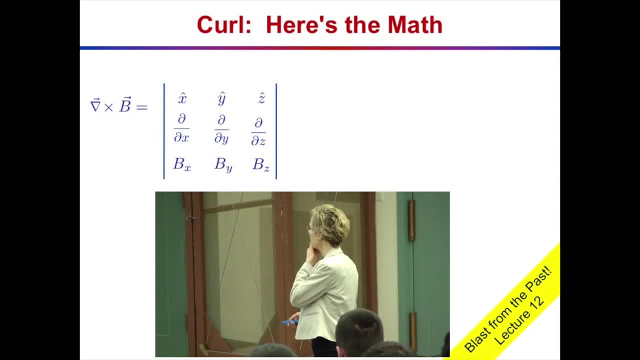 You've seen del. So you said before: there we go. This del vector is d by dx, comma d by dy, comma d by dz, And now I'm going to take that vector derivative and use it in a cross product. So here's what that's. 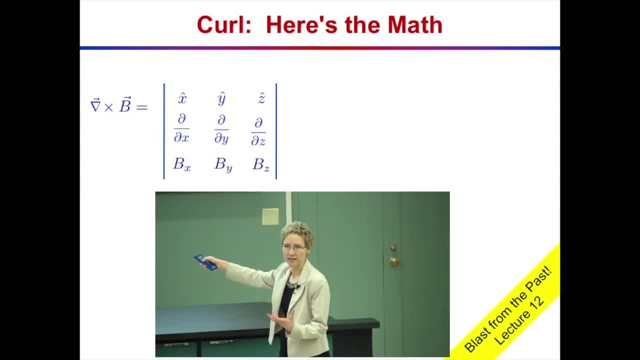 going to look like. Okay, A cross product. I can always write as the determinant set up in the following way: Determinant of x hat, y hat, z hat. Now I put this funny del vector in. Okay, Just treat it as a vector. 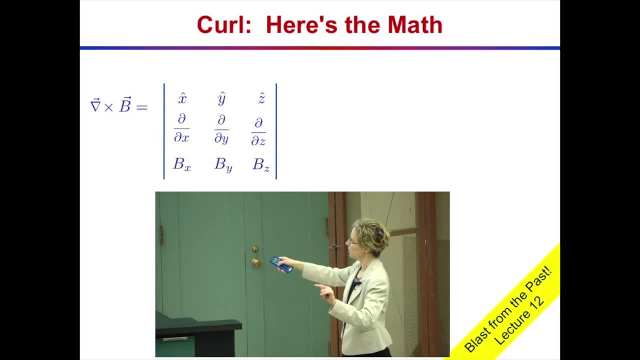 Okay, The del vector is d by dx, comma d by dy, comma d by dz And then b. I just write down Bx by bz. So this is the first time you've seen a derivative put into a cross product, but it's the same. 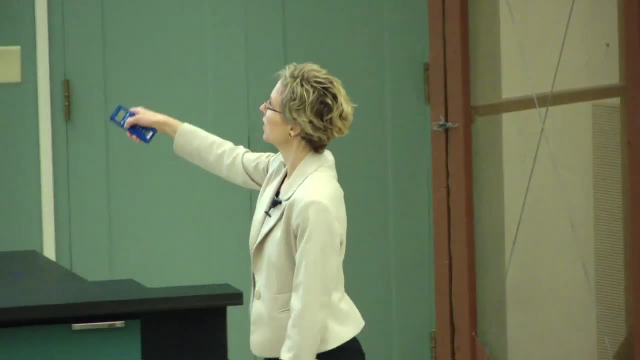 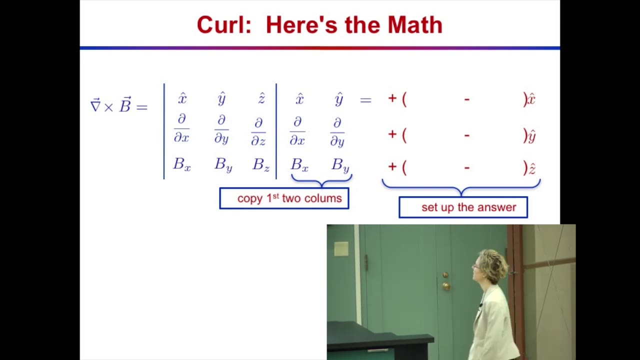 the same structure. So the way you take a cross product is you copy down the first two columns. Okay, Set up your answers. You're going to have some pieces here that are x component, y component and z component, If I think about drawing arrows down. 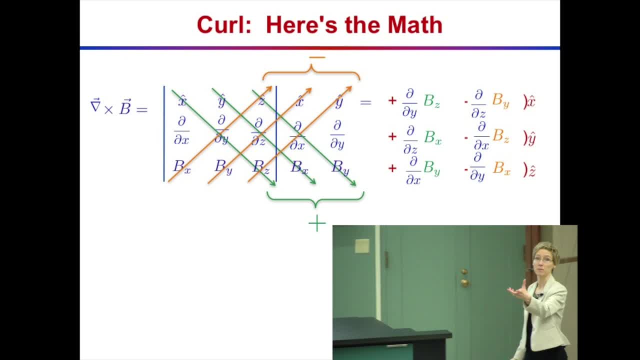 into the right. every time I have an arrow down into the right it comes up with a positive contribution. So this thing right here is x hat d by dy bz. So that gives me a d by dy of bz in the x hat direction. 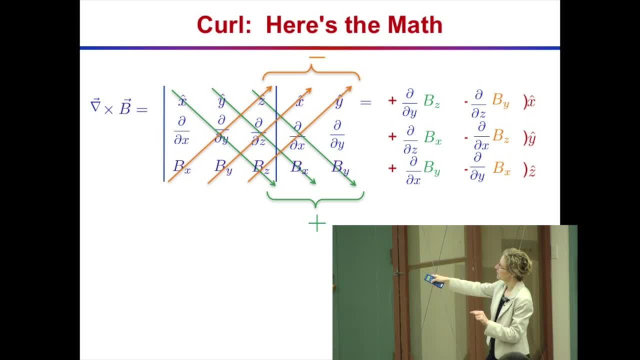 It's right here. This guy gives me d by dz of bx. Okay, d by dz of bx in the y hat direction. This guy catches z hat d by dx and by. That goes here as d by dx of by in the z hat direction, Okay. 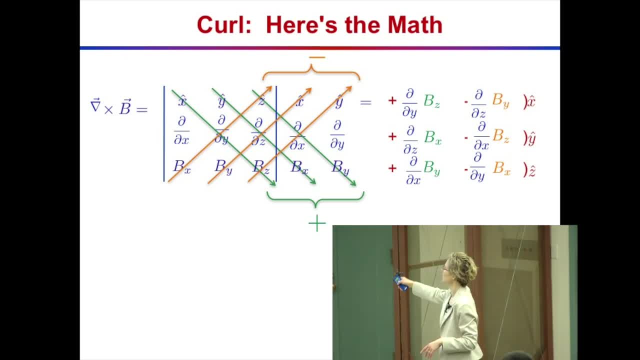 And then up and to the right gives me minus signs and those guys go right there. So it's kind of a lot of math. You can see why, with all these terms, we like to just express it as del cross b. Okay, But what it tells? 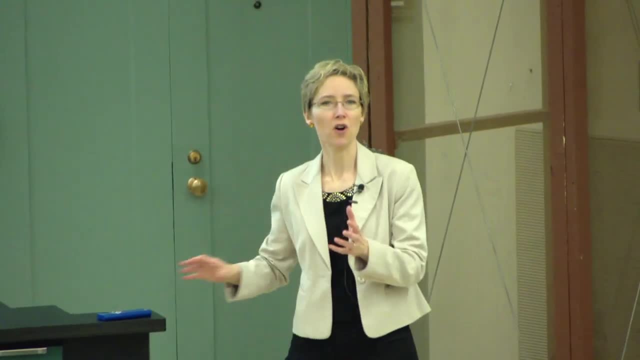 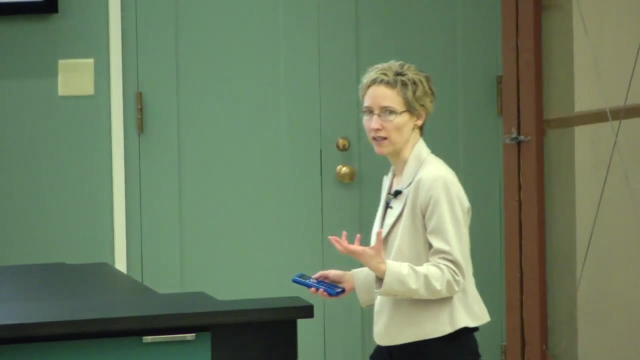 you is, is the magnetic field. this is actually called the curl Del cross, b is called the curl of b, And it actually tells us whether or not the field is curling. So I'm summarizing here for you now the integral form of Maxwell's equations. 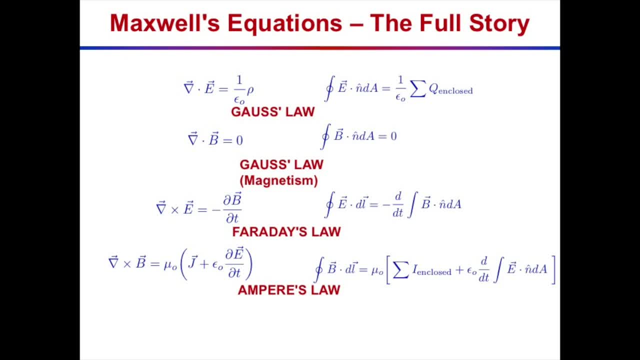 and the differential forms that we just found. We showed it for Gauss's law, but the same math would say that Gauss's magnetic law has the same form. Okay, We showed it for Ampere's law, but the same math on Faraday's law would also give you the 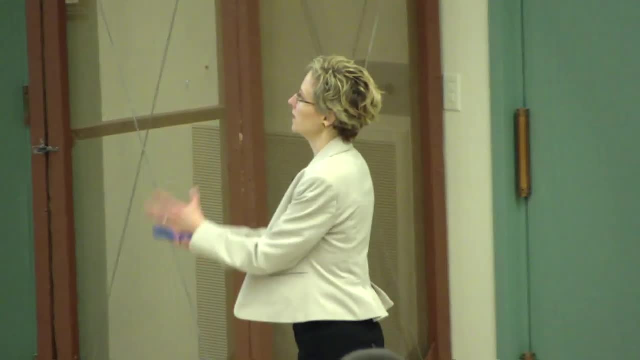 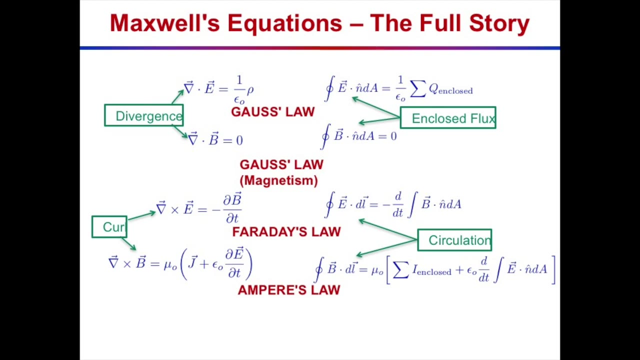 differential form of Faraday's law. Okay, So now I want to just kind of give you a sense of how this math compares. What we had before in the integral form was we had fluxes, Right, We had enclosed fluxes. So 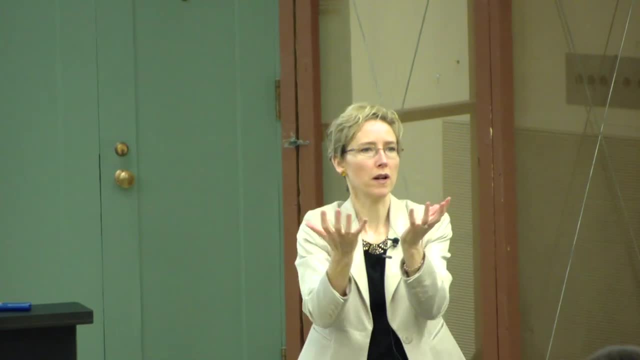 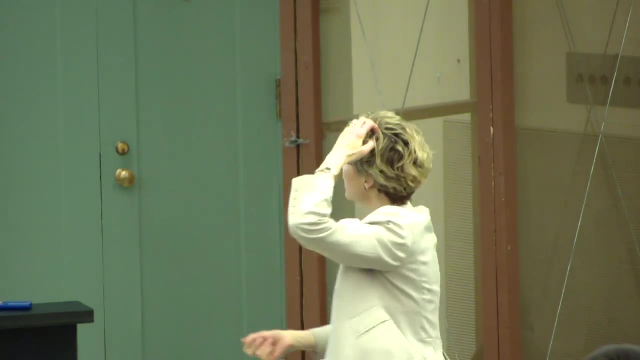 every time you see the circle on the integral, it means close, whatever this object is. If it's an area, close the area. Okay, How do I know an area is closed? If there's an inside or an outside, then it's a closed area, So enclosed. 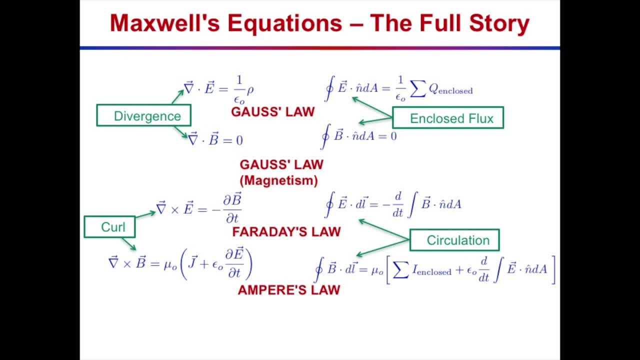 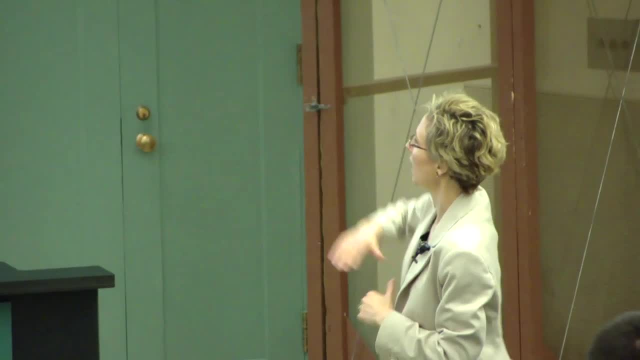 flux as an integral turns into something called divergence on the differential side, And it's very physical, Right? So just think about the top two equations at first. Think about Gauss's law in the integral form, Right? Let's think about a point: particle. 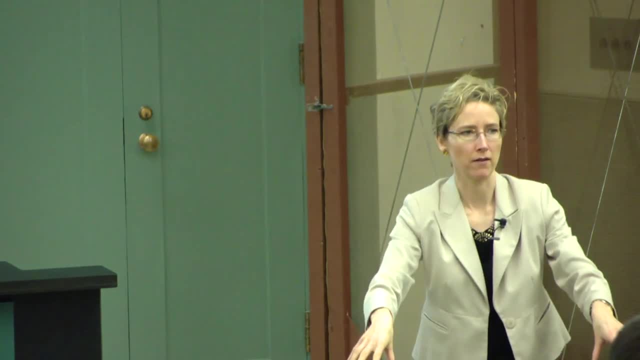 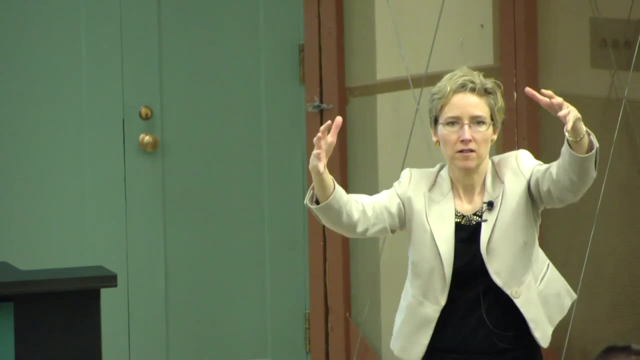 So the point particle had an electric field splaying out around it and the integral form said: okay, enclose your point particle with a Gaussian, you know, box- which, in this case a sphere, is a good thing to use- and add up all the electric flux coming.